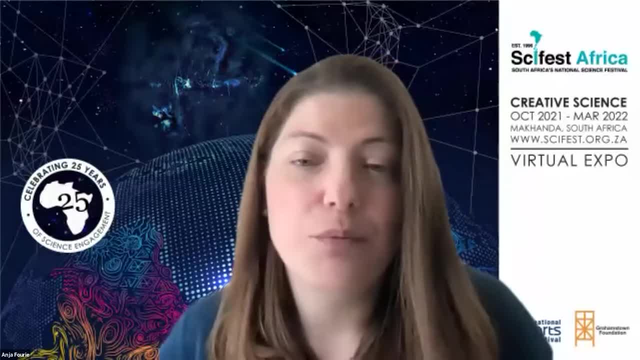 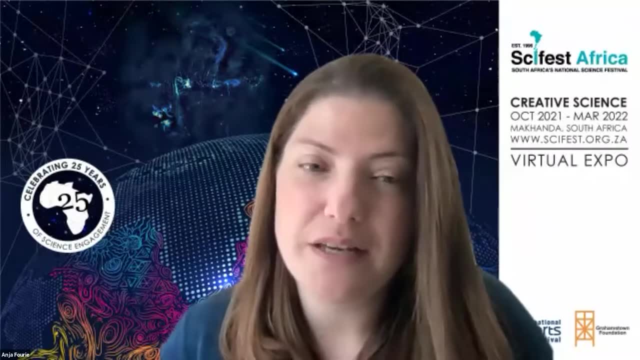 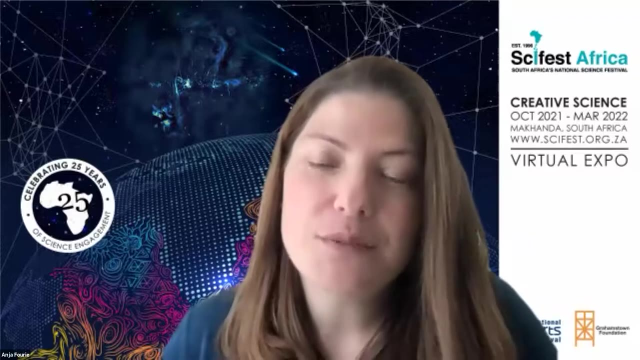 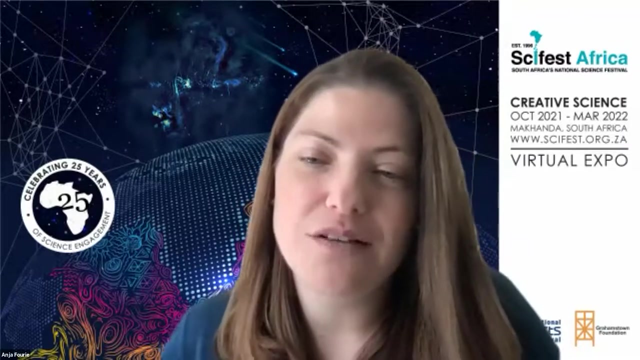 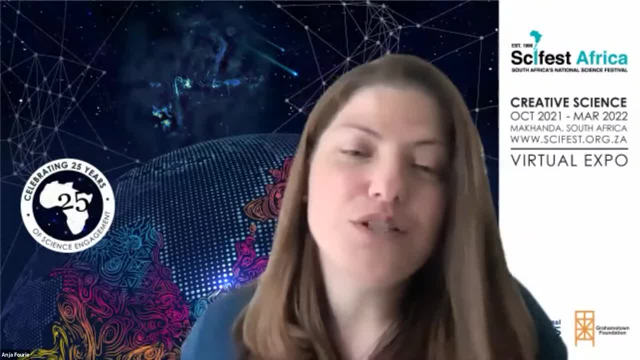 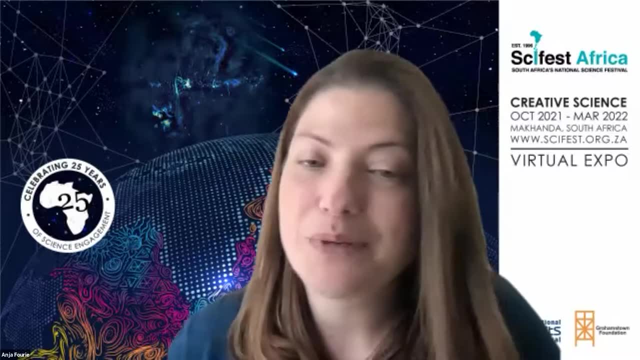 Now established in 2011,, the IAU-OAD has supported over 200 innovative projects which really work at the intersection of culture- you know, business and science, and have reached beneficiaries in over 100 countries in just those 10 years. 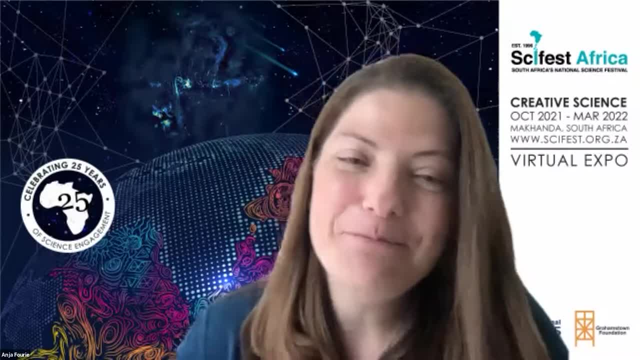 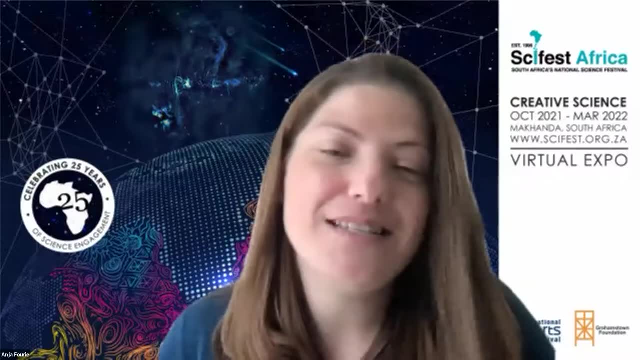 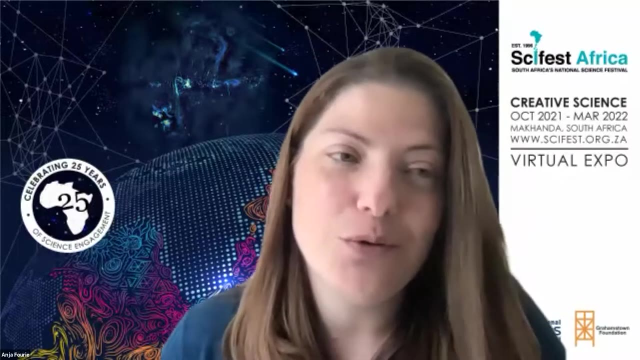 Our speaker today, Kevin Govender, began work at the IAU-OAD on the 1st of March 2011 as its first director, and he has since led the establishment of 11 regional offices around the world, and I'm proud to say that NRAO partners with the North American office, you know, hosted 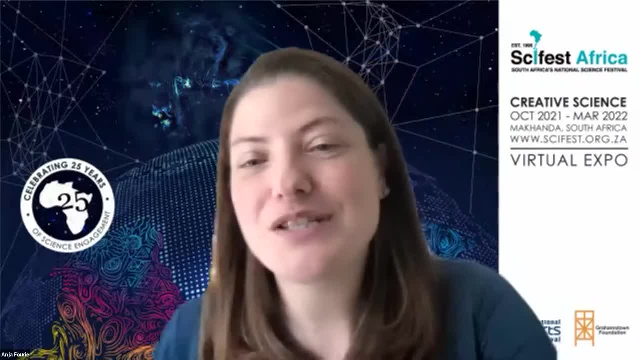 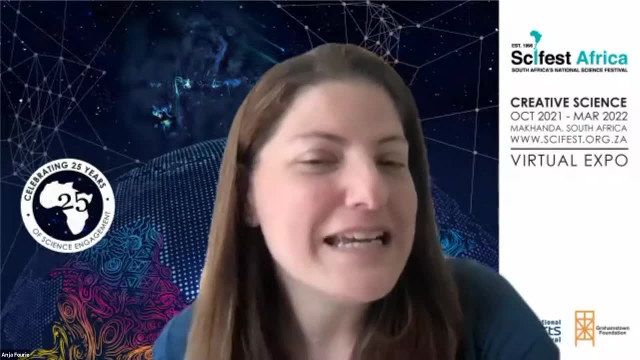 by the Association of Universities Incorporated here in the States. Kevin has extensive experience in using astronomy in research and development and he's also been a member of the IAU-OAD. really clever ways for development, not only during his previous position as the manager of. 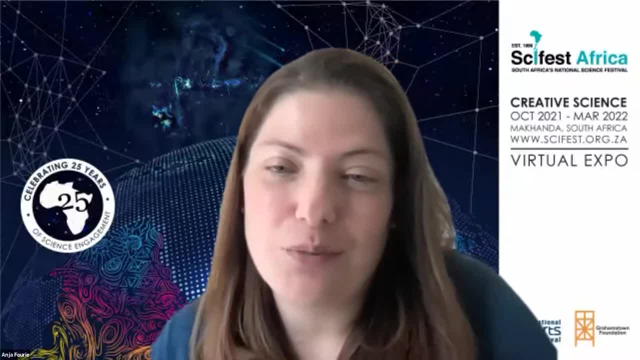 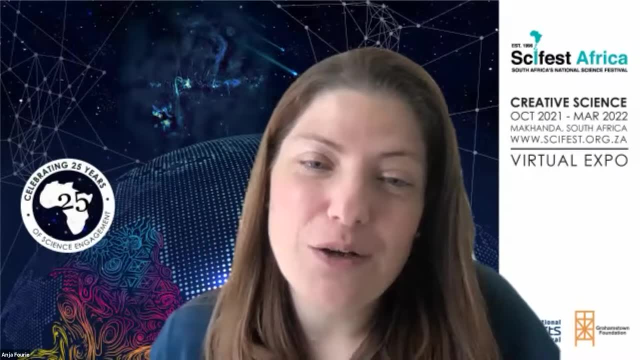 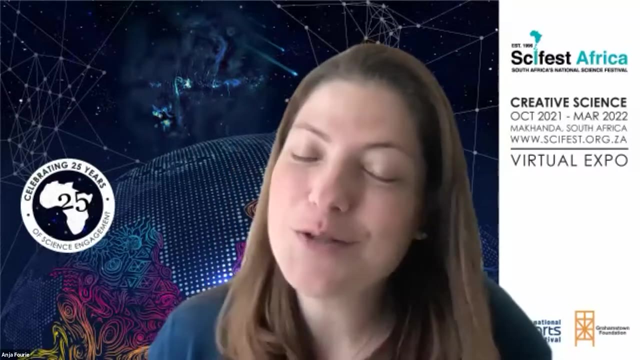 the SALT Collateral Benefits Program at the South African Astronomical Observatory, but also now as the director of IAU-OAD. He has chaired the Developing Astronomy Globally Cornerstone Project of the International Year of Astronomy, known to those of us in astronomy as IYA 2009,. 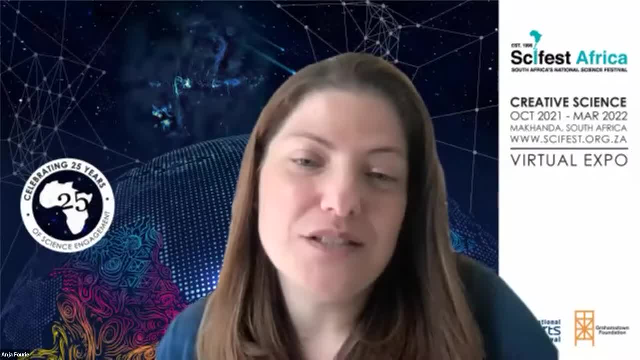 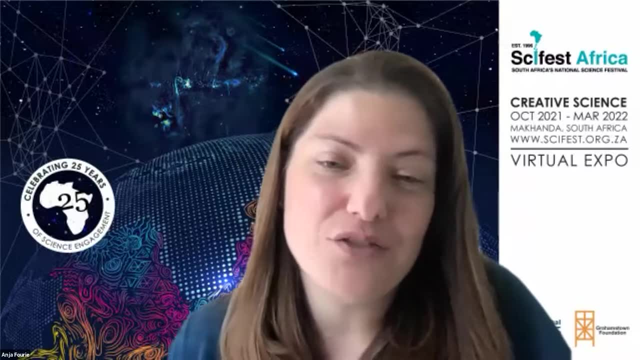 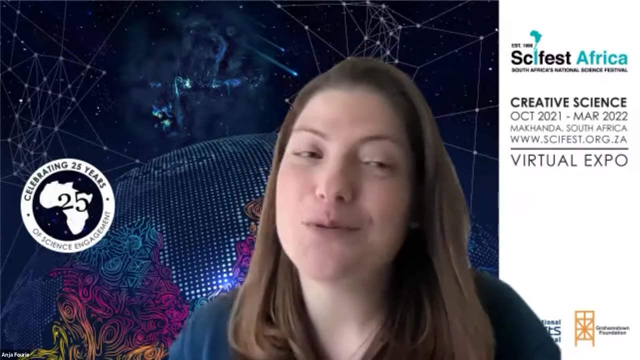 and he was involved in the development of the IAU Strategic Plan. He has been a key facilitator in the establishment of the African Astronomical Society and the movement to bring the 32nd General Assembly of the IAU to Cape Town, South Africa, in 2024, which we are very 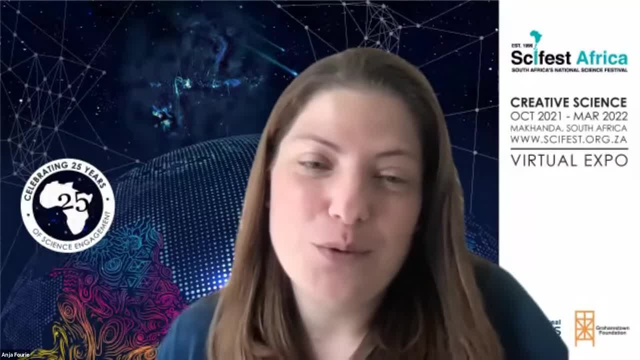 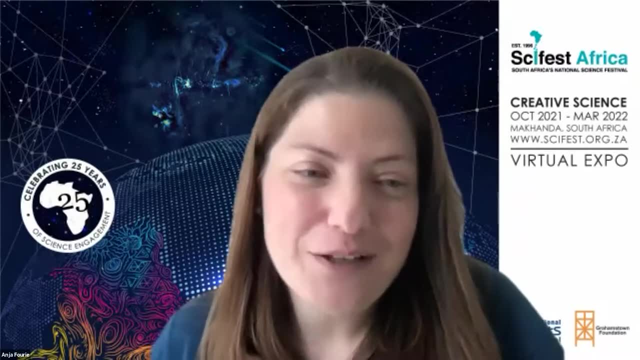 excited about. Kevin is also the first South African to be awarded the prestigious Edinburgh Medal for Science jointly with the IAU, and it gives me great pleasure to welcome you today, Kevin. It's wonderful to see you again and we look forward to hearing about the innovative 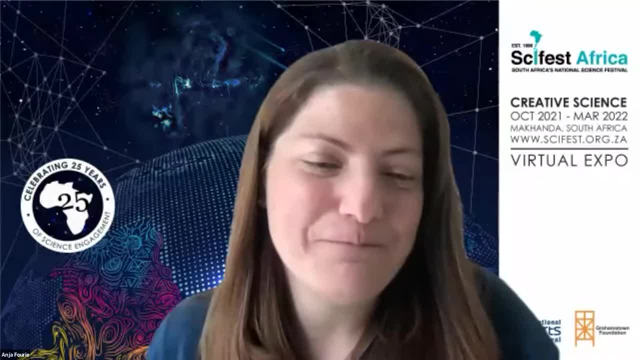 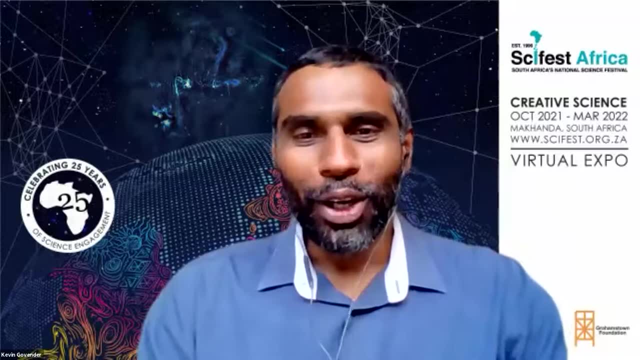 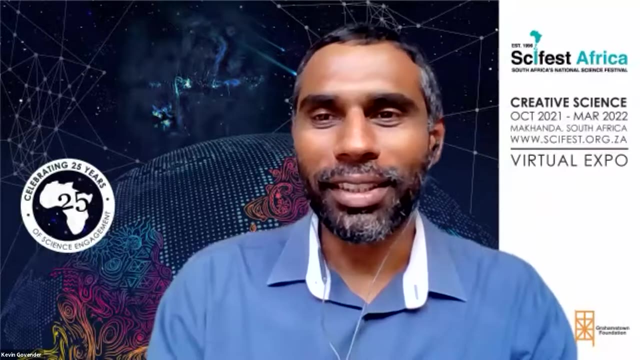 projects that you're working on in the future, Thank you. Thank you for those kind words, Anya. Anya and I go back a long way and she's singing all this praise now, but when she sees me behind the scenes then, yeah, it's a different story. So, thank. 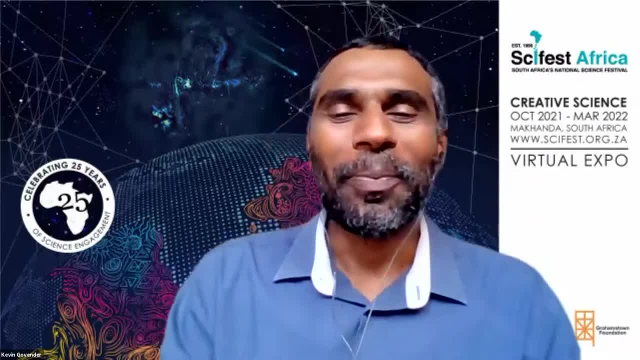 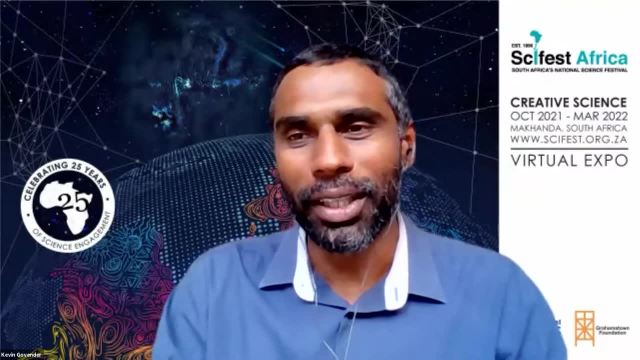 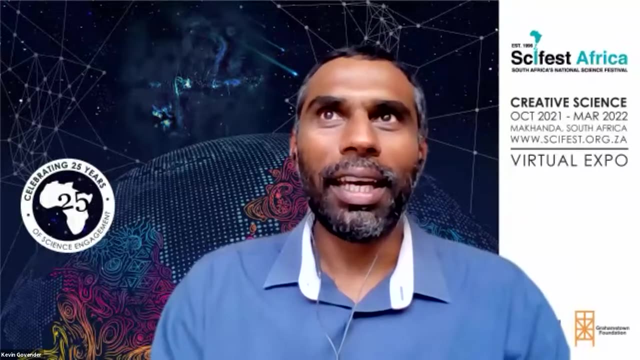 you very much for all the kindness, Anya, It's a real pleasure to be back at SciFest and to be able to work with you. I worked with Anya and with the SciFest team several years ago and it's a pity that this has to happen virtually now. 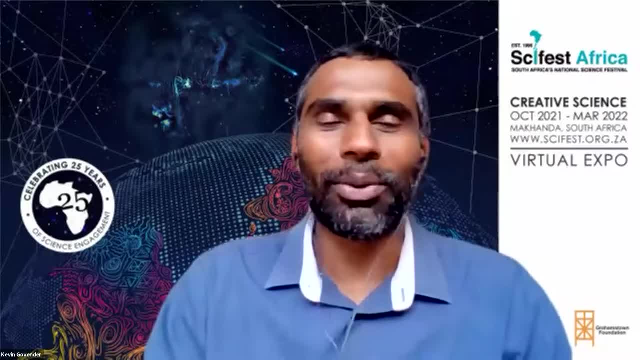 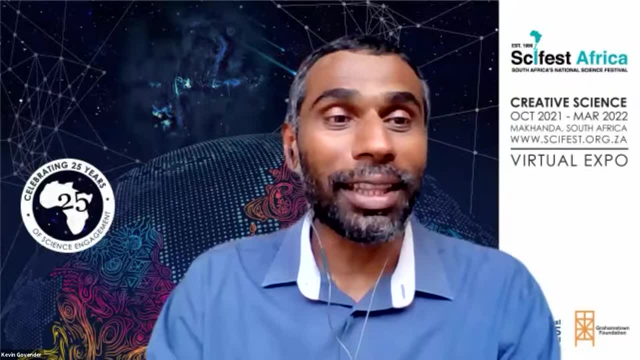 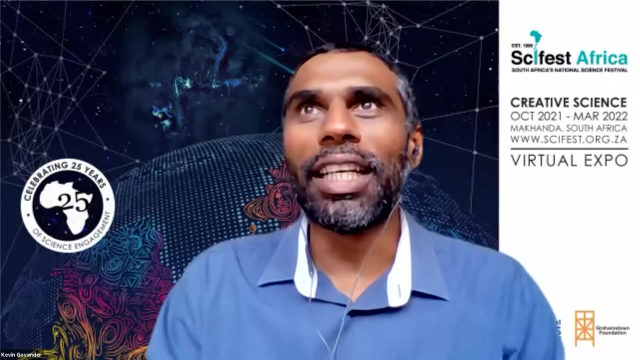 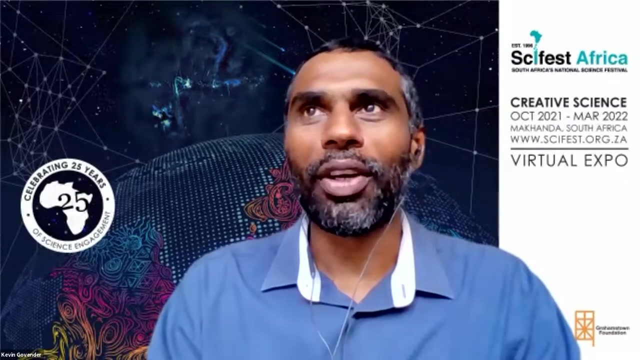 The actual SciFest event was always a highlight in South African science and in African science, But it's great that you're still able to make this happen. So I'm going to take you on a little journey from our experiences in terms of the field of astronomy, but in terms of the theme of the SciFest. 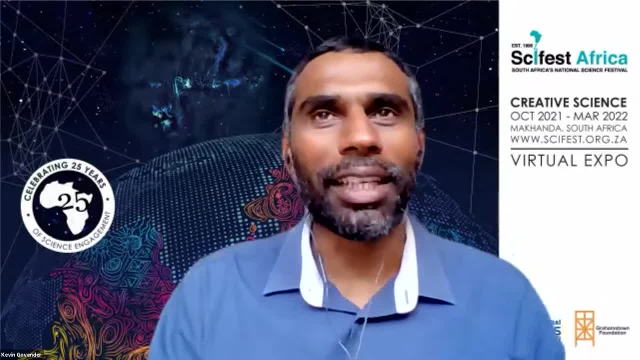 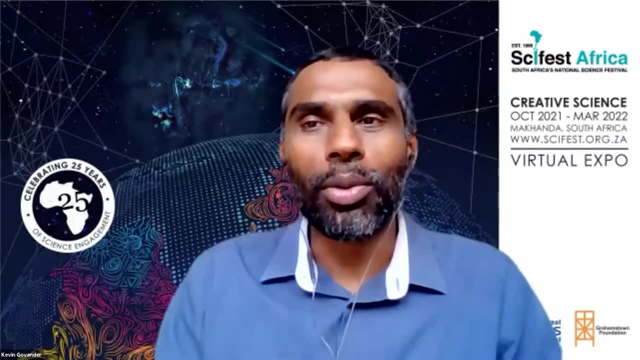 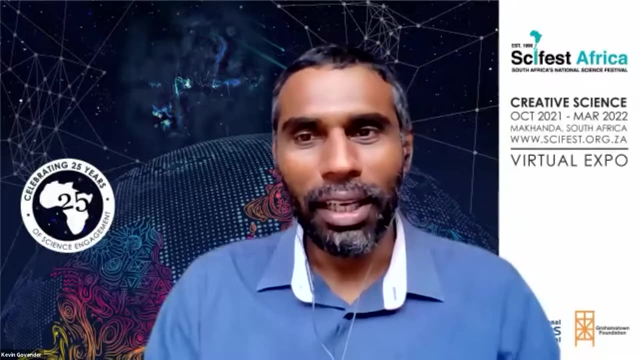 and the important words that Anya said at the beginning. we have a lot of challenges in this world And we as a science community have a lot of challenges in this world And we as a science community, as the future science community, as those that are interested in science, have a role. 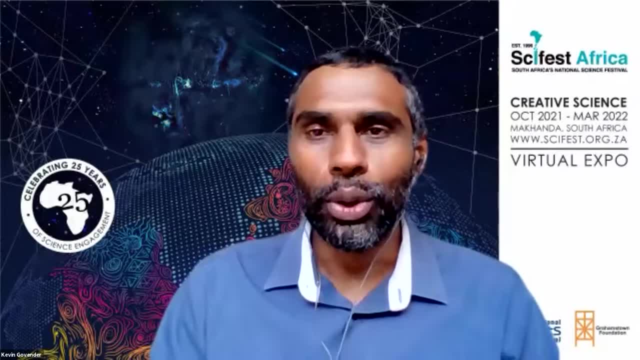 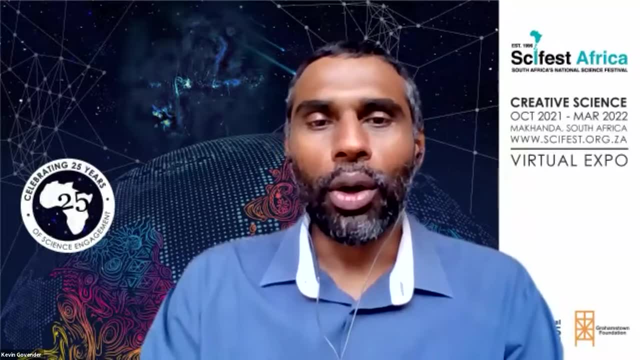 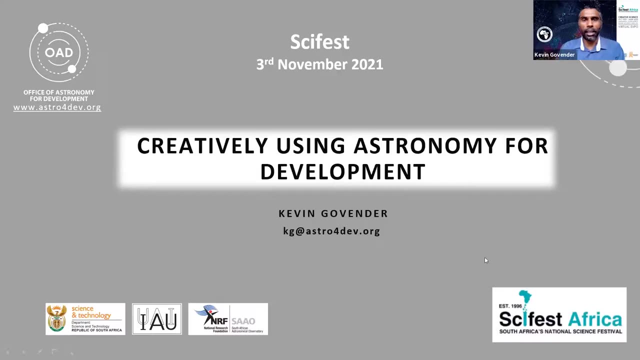 to play And what is it that we can do to be innovative about using our science to impact positively on development? So I'll talk from our perspective as the Office of Astronomy for Development. This is a project that we've been working on for a very long time, and it's been a 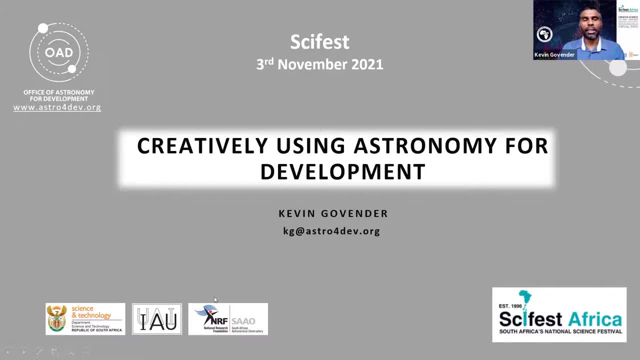 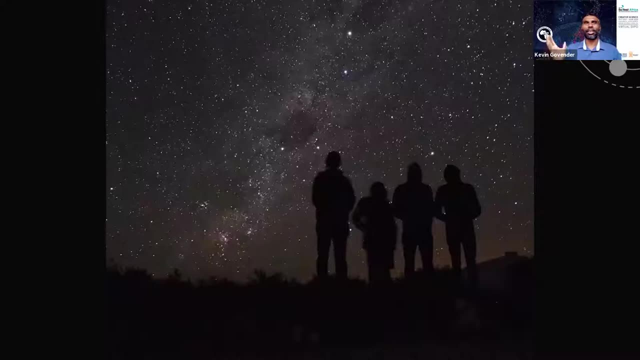 long time. This is a partnership between the International Astronomical Union, the South African National Research Foundation and the Department of Science and Innovation, And I'll give you our perspective of how we try to creatively use this field- astronomy for development. But let's start at the beginning. What is this thing of astronomy? 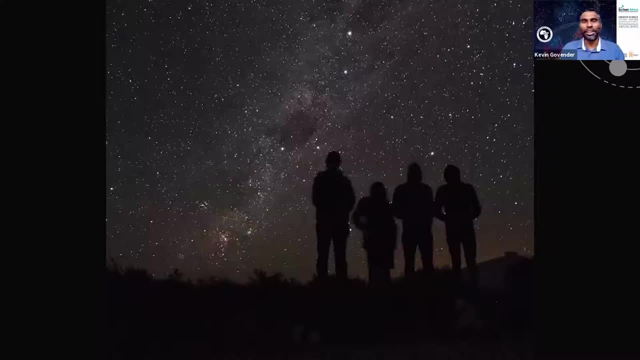 and how is it linked to the challenges we face? Well, astronomy is really about exploring. You know, this is an image of people looking at a clear night sky, And if you haven't been to the Northern Cape Province in South Africa or other, you know really. 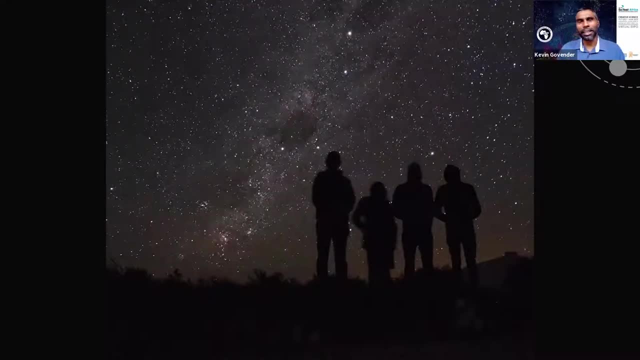 dark sky places, you know, far away from city lights. it really is an experience And I would encourage you to get out there and feel it for yourself, Because when you get a clear sky like this, you really feel the reality of being in space, Because that's where we are. 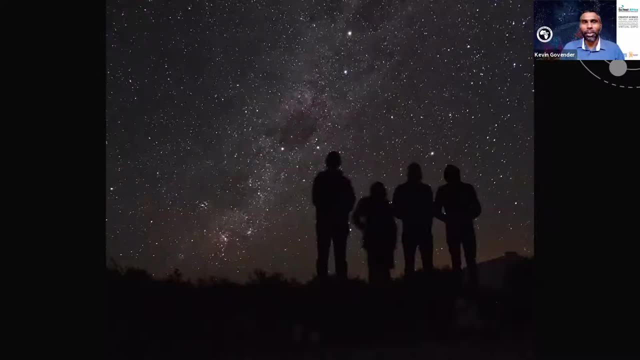 right, We are on this planet- Some people refer to it as Spaceship Earth- And we are looking out into space. But that out into space, that's where we are. We are in space. We are on this rock that's moving around one of those stars, And we see these thousands of stars with our naked eye. 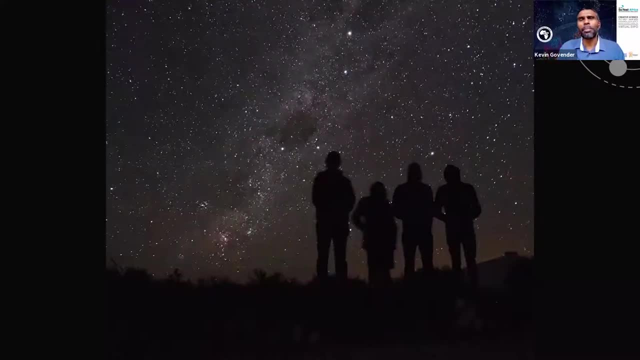 With telescopes, we see millions of stars. With bigger telescopes, we see billions of stars, And astronomy is about exploring. It's about trying to figure out. what are those things, What are those stars? What are galaxies, What are black holes? Where did the universe come from? 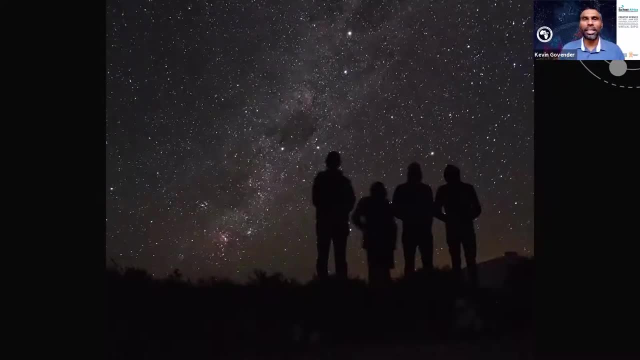 Where is it going? And this exploration is something that stretches our capacity to think, stretches our minds. Those stars that you see when you look up at the night sky, all of the stars that you see, are so far away that no spacecraft that we have today can get us there in a reasonable time. 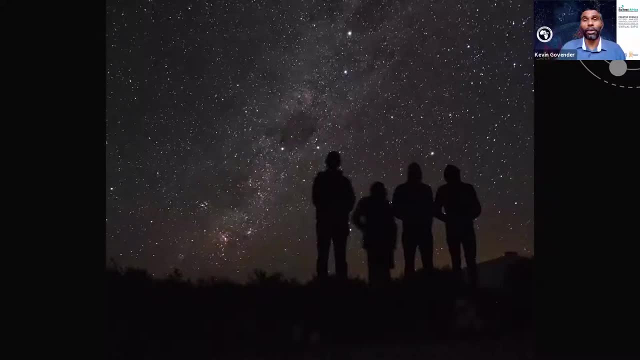 In reasonable time, I'm talking the nearest star- will take like 70,000 years for us to get to. So how do we explore things that are so far Well? we have to be really creative. We need to figure out: okay, let's, let's catch the light that's coming from these stars and let's try and 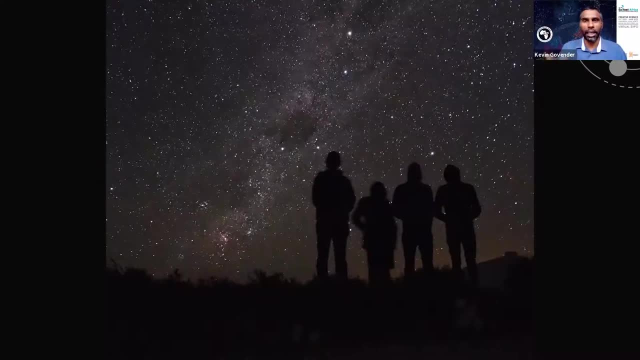 figure out: uh, you know how far they are, what are they made of? uh, how hot they are. are they moving towards us, away from us? and all this we can do just by, just by using our imagination, using our creativity, and i want to give you an example of, of, of, of, of a really cool uh um story, that that. 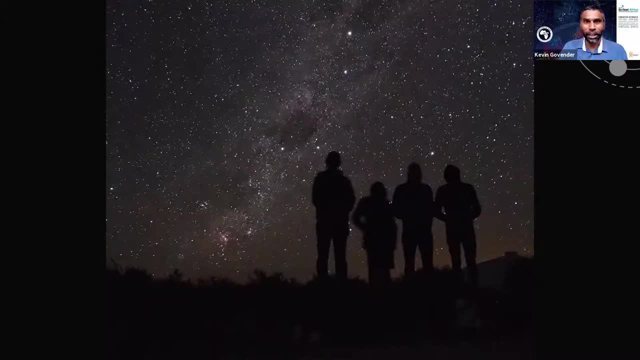 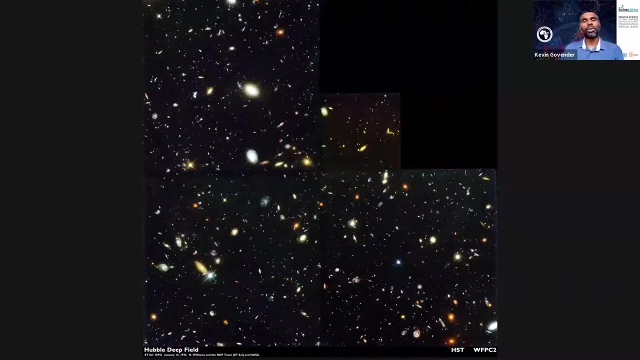 uh, that's close to us, at the, at the oed. this was the image taken. uh, uh, the the. this was the hubble deep field image. so this is an image taken by the hubble space telescope and it was taken over a period of 10 days. and what they did was they pointed the telescope at a part of the sky where 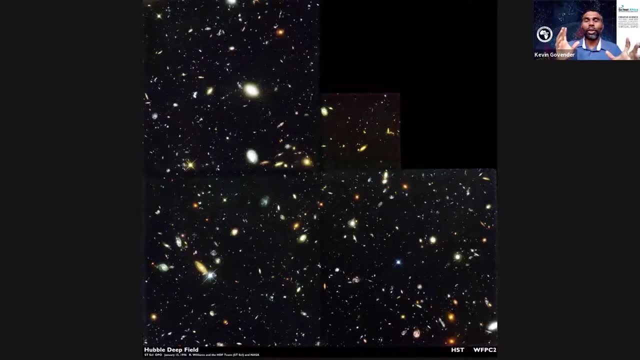 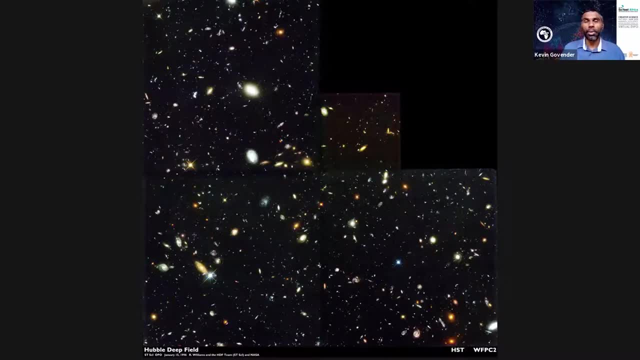 of the international astronomical union and at the time he was in charge of the space telescope science institute, so they were in charge of the hubble space telescope and uh. so bob williams was one of those that helped start this office of astronomy for development and i asked him about. 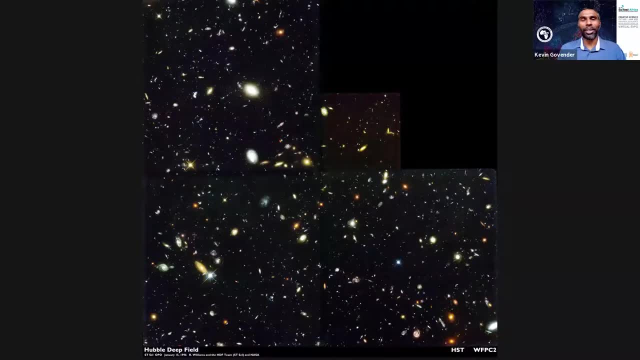 this, and you know he was telling us the story uh uh uh about, uh uh, like what gave him the idea to look at a dark part of the sky? because what he did was he used his discretionary time as the director of the hubble space telescope. uh of the space. 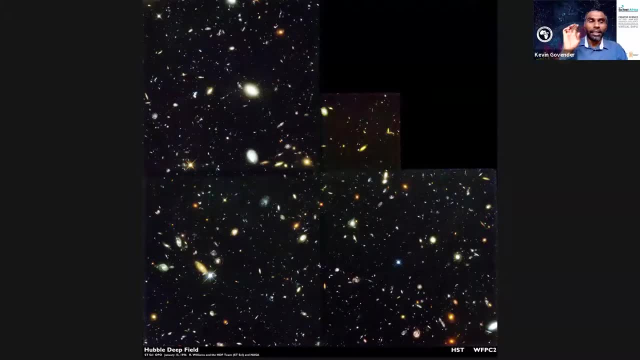 telescope science institute, um, and he used his time to give 10 days. i mean, this is a huge instrument, it's a super expensive instrument and any time is super valuable, right? so he said, like all his colleagues were saying: you're crazy, you, You're not going to observe anything. 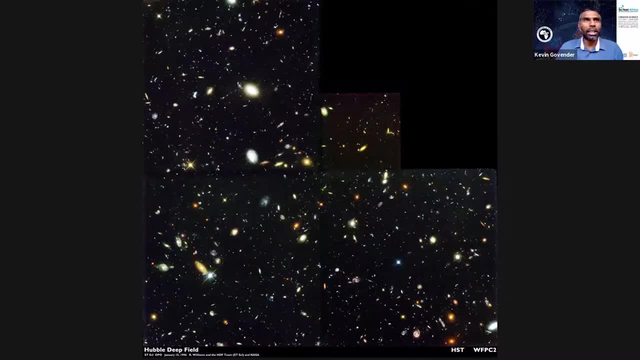 Why are you wasting this telescope time looking at a dark patch? He said. well, when he was a kid, you know, he used to use a telescope and just he loved looking at dark parts of the sky because with a telescope you'd see stars that you can't. 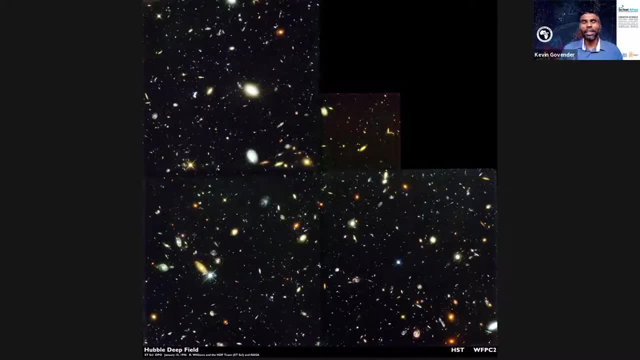 see with the naked eye, And it was that curiosity that drove him to use his influence to point the Hubble Space Telescope at a dark part of the sky. And this is what they found Now in this field, in this picture that you see, there's something like 10,000 galaxies. 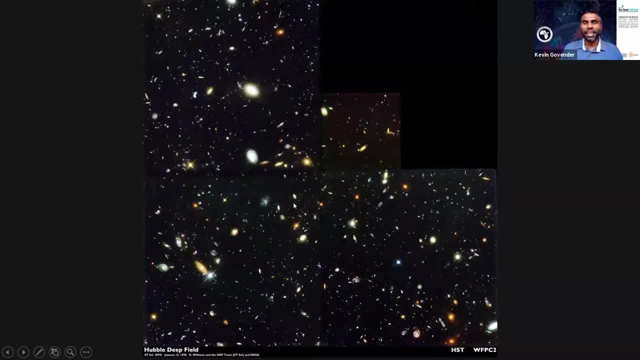 Every little smudge you see, here is a galaxy. What's a galaxy? A galaxy is made up of, like our galaxy. the Milky Way galaxy is made up of about 100 billion stars, stars like our sun. Our sun is one star. 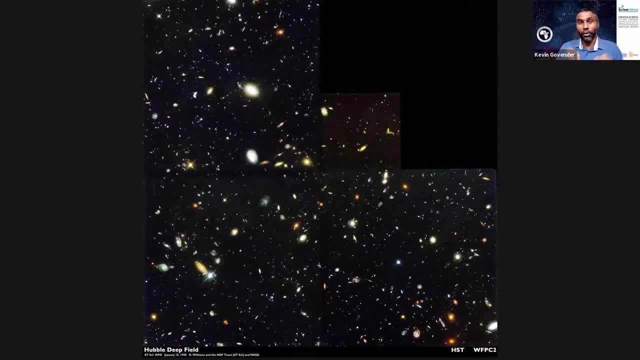 A galaxy has hundreds of billions of stars, of suns like ours, And here you have 10,000 galaxies in a tiny, tiny part of the sky. How tiny is this part of the sky? Imagine if you take a little, take a needle, and you look through the eye of the needle. 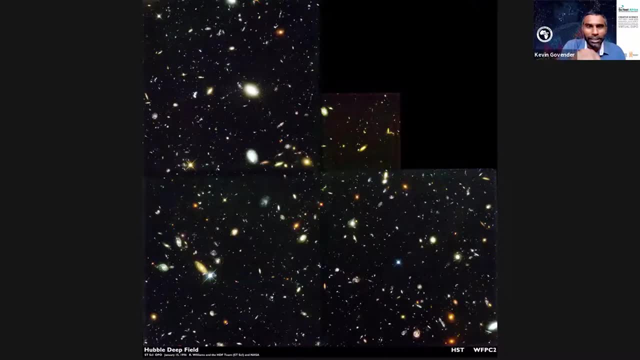 That tiny piece of the sky that you see through the eye of the needle. that's how big this piece of sky is, And they found thousands of galaxies in that tiny piece of sky. So when we look up at the sky, you know, when we see the sky with, you know all these stars. 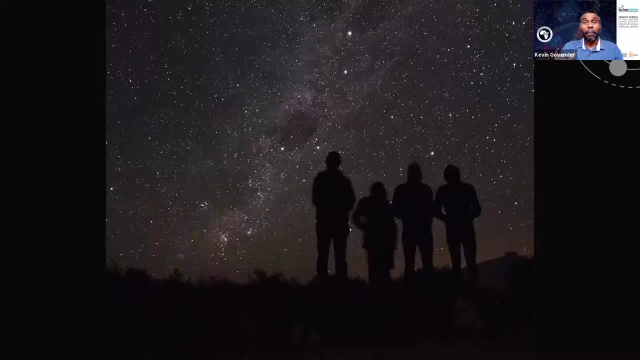 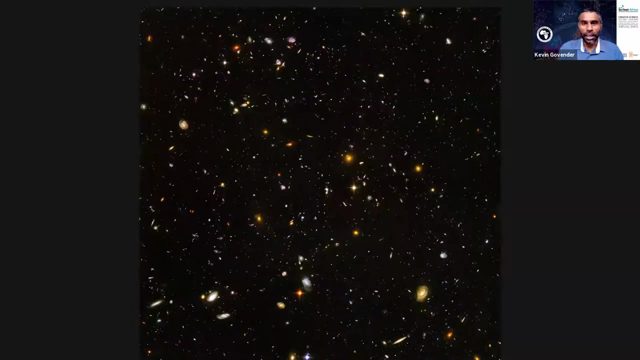 and you know, the Milky Way across the sky, And remember that there is so much more out there that we can't see with our naked eye. And that's what these, that's what astronomy is about. It's about exploring. This is the current, this is the next generation, called the Hubble Ultra Deep Field. 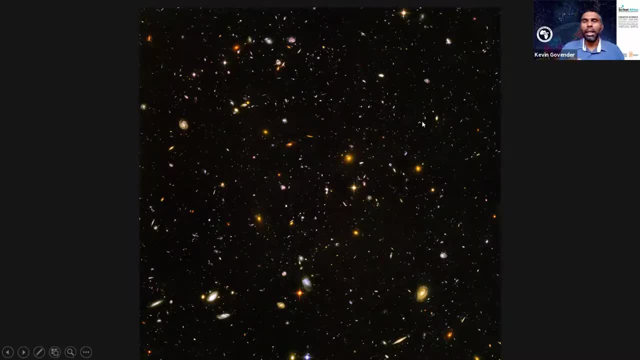 And every little smudge you see here is a galaxy. There are billions and billions and billions of galaxies out there And remember every galaxy has billions. There are billions of stars, stars like our sun, And every one of those stars could have planets around, planets like our, like Earth. 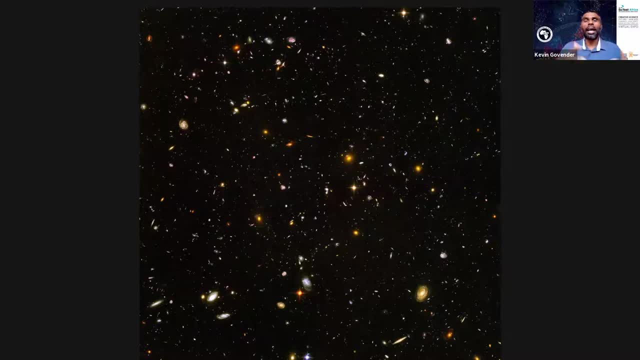 Astronomy is about trying to figure all this out. It's about trying to ask these big questions, You know: are we alone in this, this huge universe? Are we alone? Are we? are there life forms out there, different kinds of life forms? 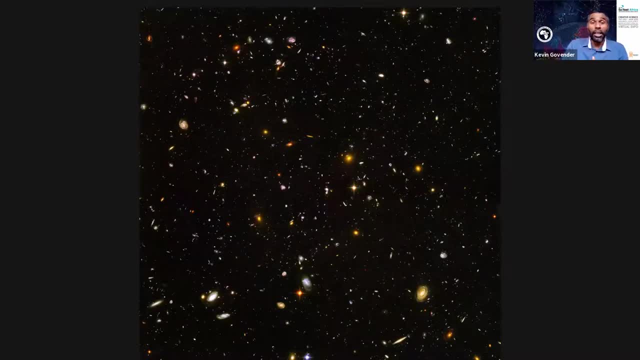 If so, where would they be? If so, how would we communicate with them? Because the light takes millions of years to to to travel to us. These are, these are all the challenges that we get in astronomy. Now, this is a picture of Bob Williams. 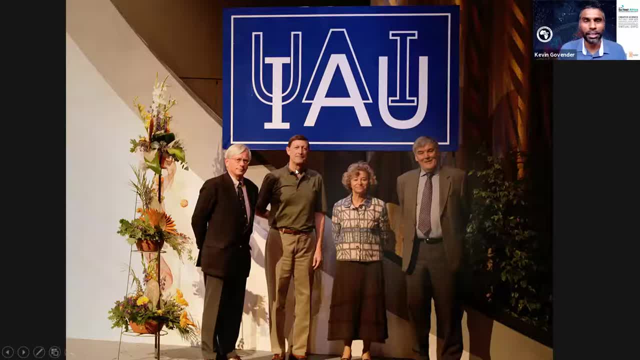 And you know it's a- I'm putting it here as a tribute to him- And this was Ian Corbett Both. he was president. Ian Corbett was was the general secretary when the Office of Astronomy for Development was formed. 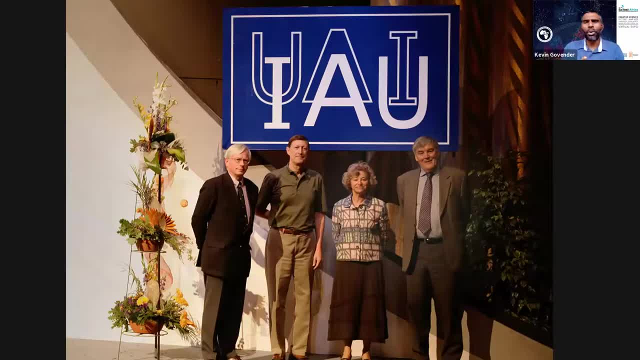 Now they should be credited. They should be credited with the idea of asking the question. how can we take this field of astronomy, looking at things millions of light years away, so so out of reach? how do we take the strengths of this field and apply it to human development? 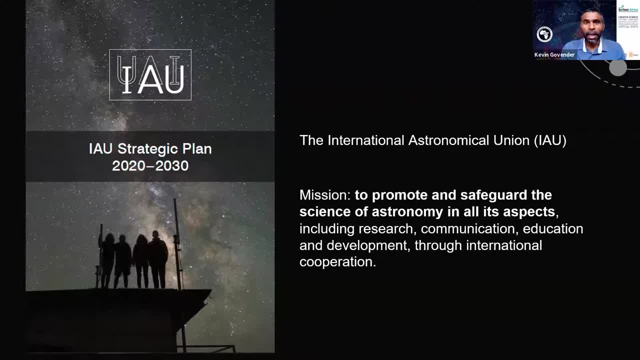 apply it to the challenges we face on this planet, And that is where the International Astronomical Union took the lead in this area. Now, who are they? They are basically the custodians of astronomy knowledge, so their mission is to promote and safeguard. 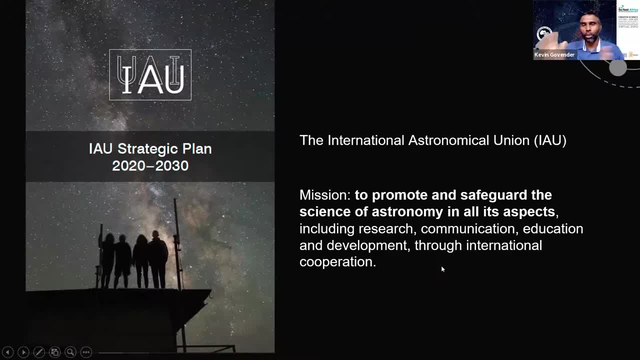 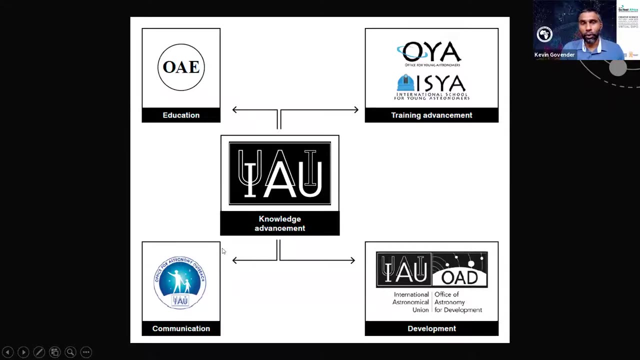 the science of astronomy in all its aspects: research, communication, education, development. now this international astronomical union established a strategic plan, so this is the current one that we're on and one of its four offices. it has four offices: one dealing with outreach, one dealing with education, one dealing with astronomy training, and one of its four. 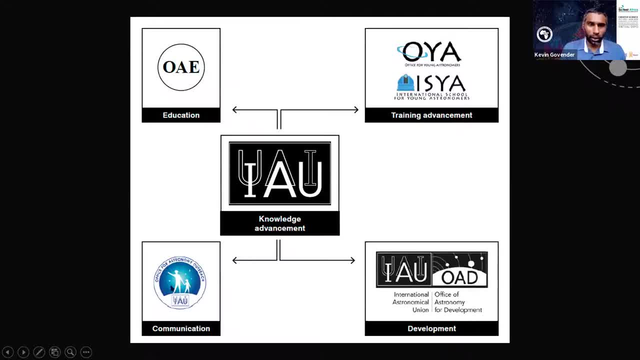 offices is the one based here in south africa. so the outreach office is based in japan, the education offices is based in germany, the young astronomers office is based in norway and ours is based in cape town in south africa. now, these are all international offices and our office is 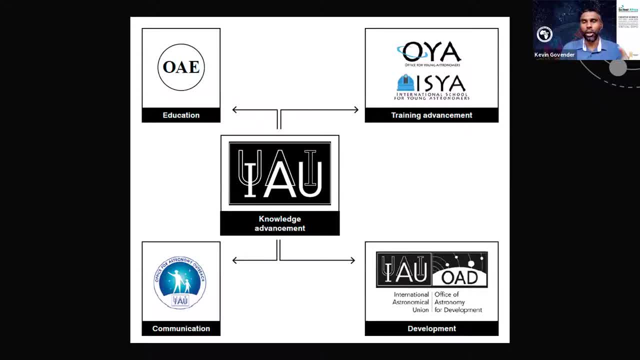 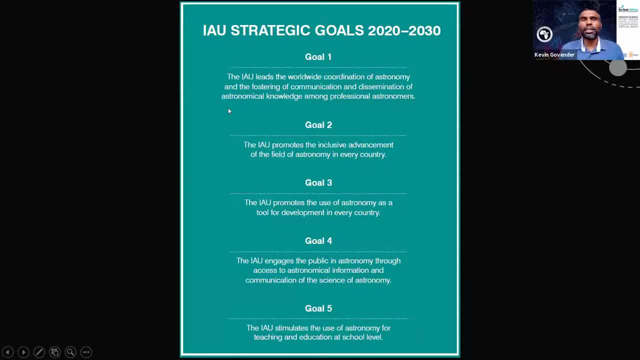 dedicated to, to, to using astronomy to impact on development, and this strategic plan has specific goals, and- and these goals vary from you know- growing astronomy as a field, communicating astronomy with the public, using astronomy to stimulate interest in science. and our specific goal is about using astronomy as a tool for development. now, what are we talking about here? astronomy has 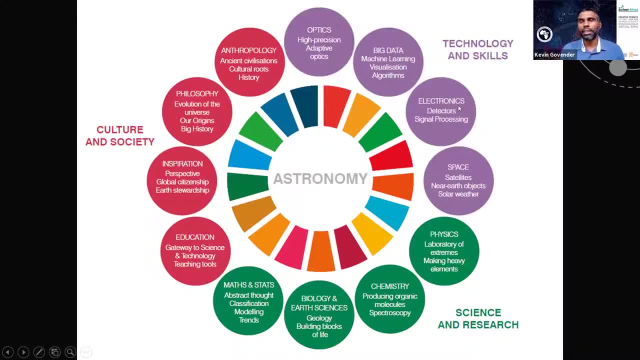 connections to lots of different areas, but it's technology and skills, uh, because you know to do astronomy, we need, uh, high precision optics for big telescopes. we need to use big data, we need super sensitive electronics. uh, there's also connection with space. um, then, on the science and research side, well, if you're 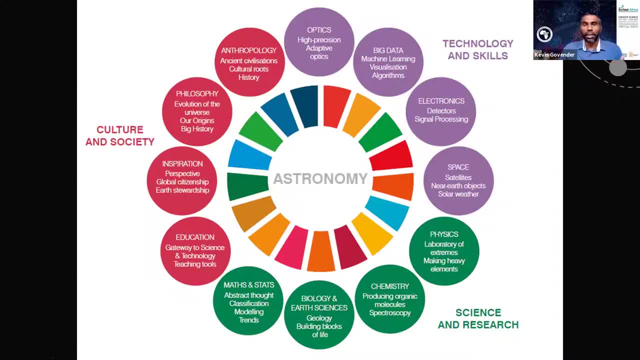 going to explore the universe, you need to uh work with other fields. you need to know physics and chemistry and biology. people give a life elsewhere. you need to know biology, uh. and so astronomy connects with all the different areas of science and research. but, importantly, astronomy also connects with culture and society, and this is 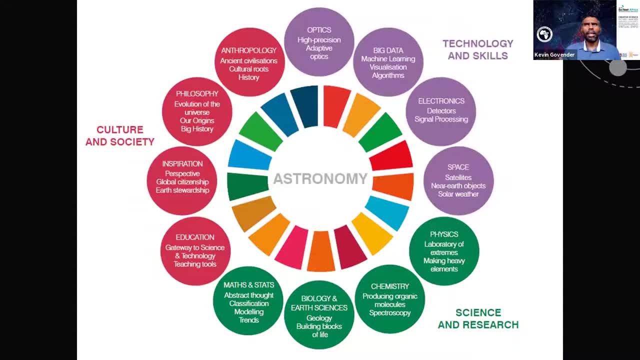 where, um, you know there's, there's the the cultural side of astronomy, where we want to use the connection that that we, as you, as human beings, have with astronomy. now, you'll find that almost any culture anywhere in the world has some connection with astronomy, and astronomy is a. 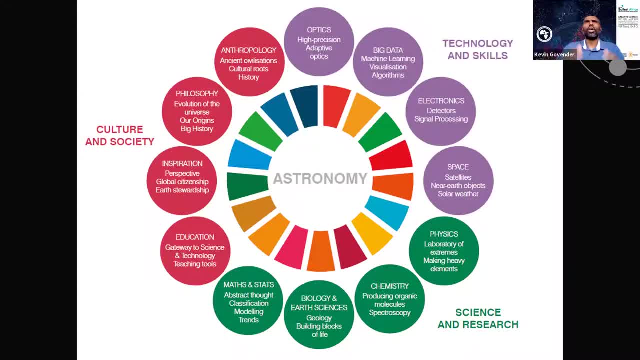 very important part of the history of astronomy. in fact, you know, uh, you look back, you know, to our ancestors. uh, even if, uh, the science of astronomy was not developed, there was curiosity about what are those things in the sky, what are stars, what are eclipses, what are seasons, and, and people have 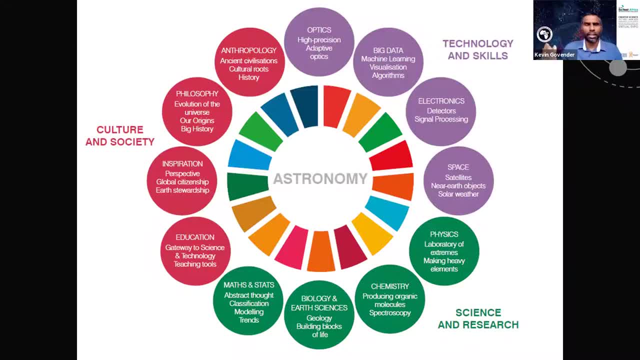 come up with different explanations over over centuries. um, astronomy today is is basically doing a similar thing. it's about asking questions and asking questions and asking questions and trying to figure out, with the best ways that we have at the moment, what is going on out there. and 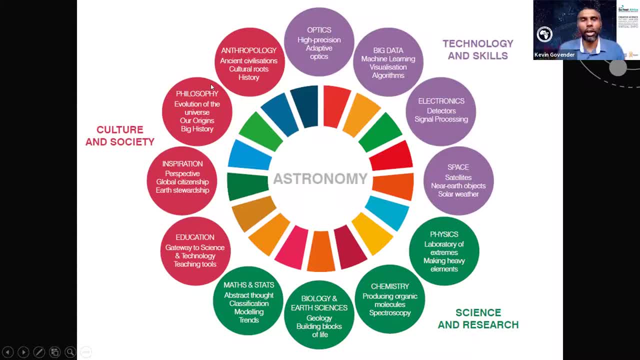 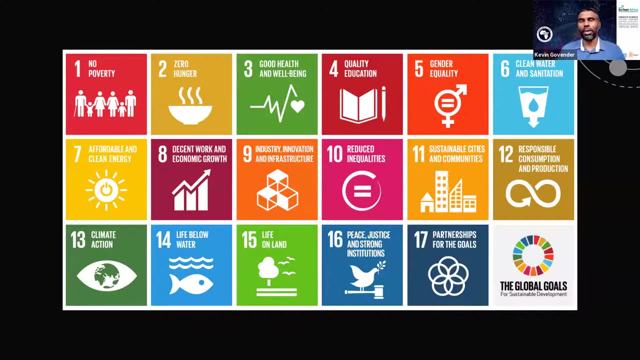 so that that inspirational and cultural aspect of astronomy, how do we connect that with the technology, with the science, and look at astronomy in all its aspects and see how it can impact on development? now we talk about the sustainable development goals. why do we talk about it? you know. 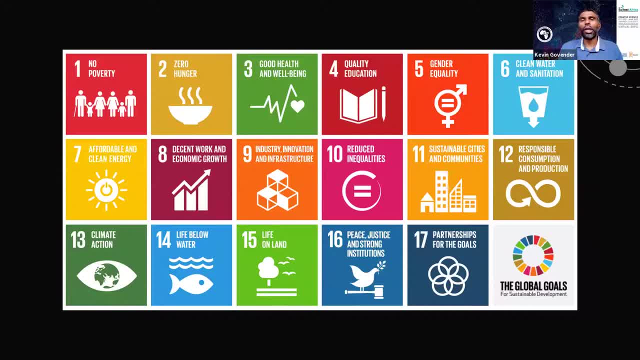 simply put these: this is the closest to a universal definition of development, and, i should say, agreed definition, because this was driven by the united nations. it was something that, uh, you know. the question was asked: how do we rally the world together, how do we rally all the countries to, to, to improve life, to make the world? 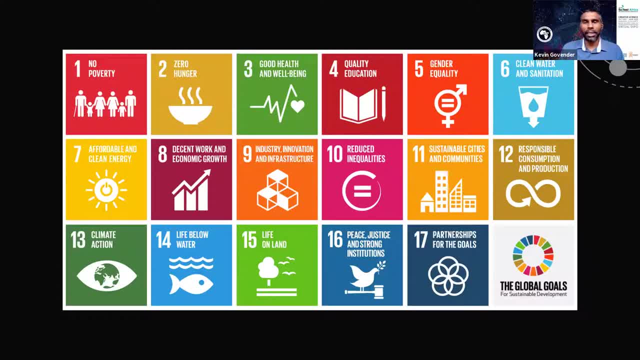 a better place and these are the goals that, uh, that the united nations, through this process, came up with. so we use this as a guideline. but you know it, it's, it's fairly complete, it's fairly, uh, broad, but at the end of the day, we're saying that the idea of this is: let's, let's get on the same page. 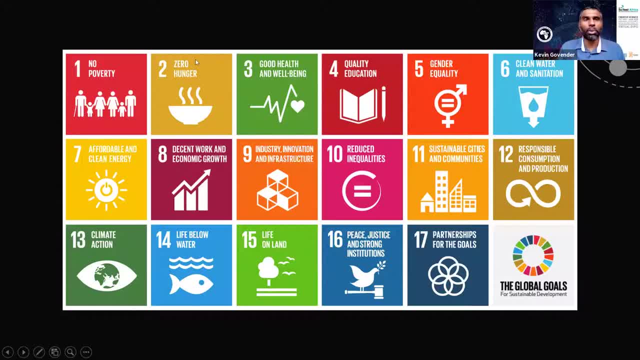 as what we mean by development. you know, we all want no poverty, we want zero hunger. uh, we want quality education, reduced inequality, so it's all things that we, as society, want, and so, um and so, with this, uh, uh, we try to ask the question: how can astronomy impact on all this? how can astronomy impact on? 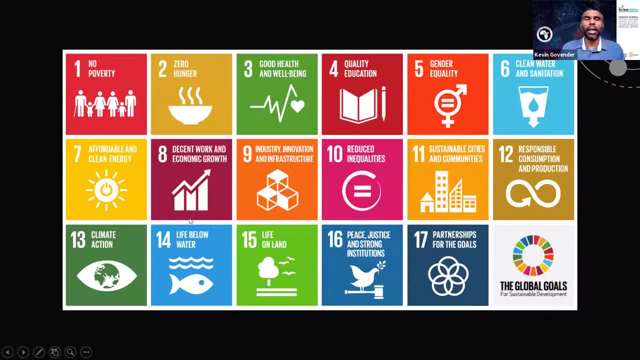 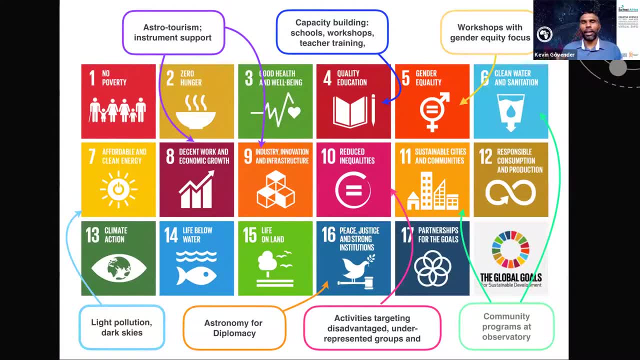 quality education. how does astronomy uh impact on economic growth, for example, and those uh ways in which uh astronomy is used? that's where, you know, we come to the idea of, like, creatively using our science to impact on development, because this doesn't necessarily have to be only uh, you know. 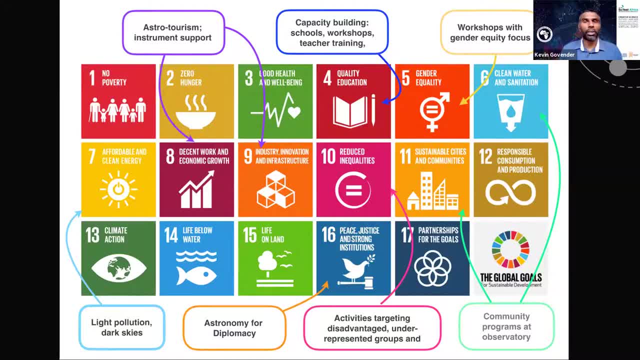 restricted to astronomy. This is something that could be applied to any field. how can- how can, mathematics benefit all these different areas of development? how can chemistry benefit all these different areas? So you know I speak from our experience in astronomy, but it's something applicable to any science, From astronomy, for example, you know, astrotourism is something that impacts on decent work and economic growth. 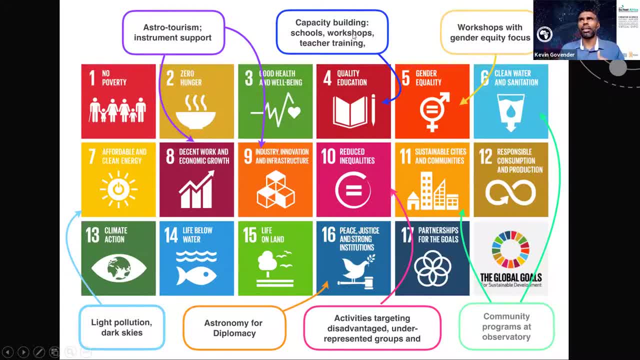 If we talk about capacity building, schools, training people on big data skills and so on, it impacts on quality education. We can use astronomy for diplomacy, for example, where we impact on bringing countries together around astronomy. When you're on a planet and you want to observe the universe, you need to collaborate with the institution internationally. 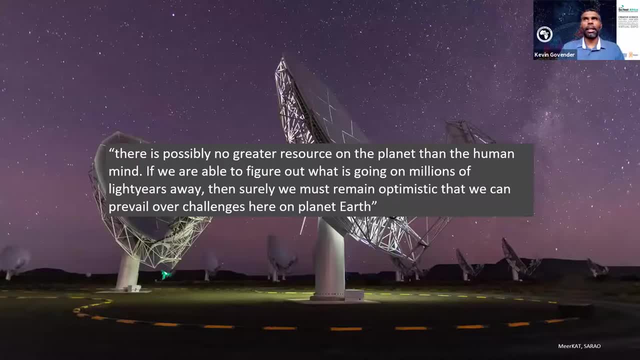 So let me pause here, because when we try to impact on the world, when we try to make the world a better place, this is sort of the philosophy that we go by: is that there's possibly no greater resource on this planet than the human mind? 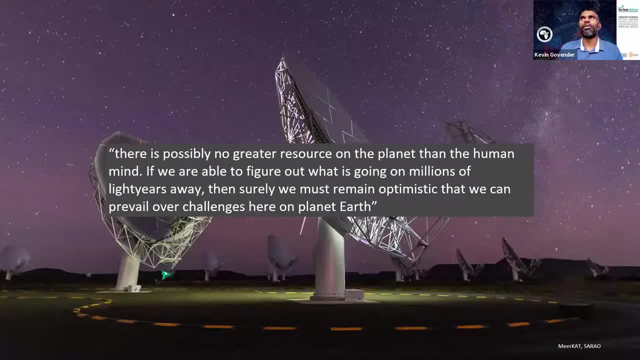 The human mind has. you know, if we use it, the collective human mind, the human thinking, the human mind, if we use it well, then we can do amazing things. And if we are, you know, in astronomy, if we're able to figure out, you know what's going on millions of light years away, then surely we must try to figure out how we can prevail over challenges here on planet Earth. 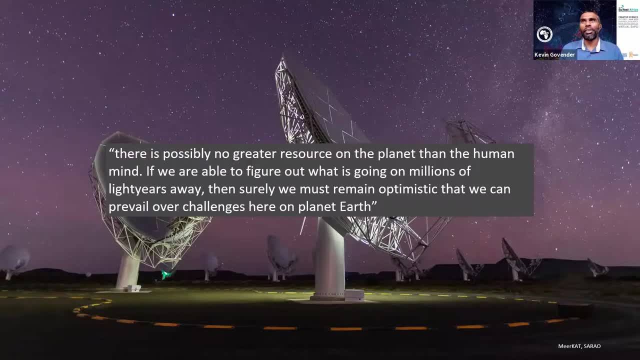 The human mind can also be used in a very negative way. you know, If people influence people towards violence, towards you know sort of negative things, then that drifts us in the other direction. So, in terms of where we are at the moment, 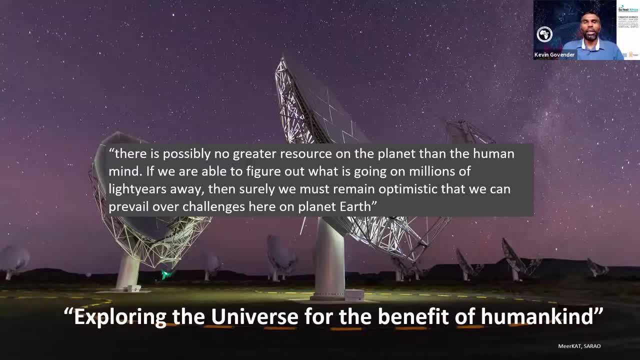 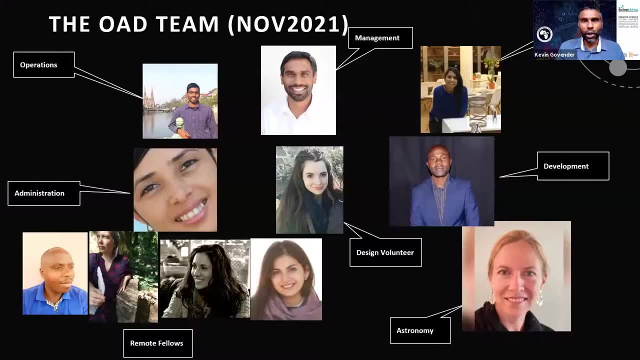 the simple principle is that, within astronomy, how can we explore the universe for the benefit of humankind? So let me give credit to our team. I mean we have a team based in Cape Town. we've got remote fellows based in different parts of the world. 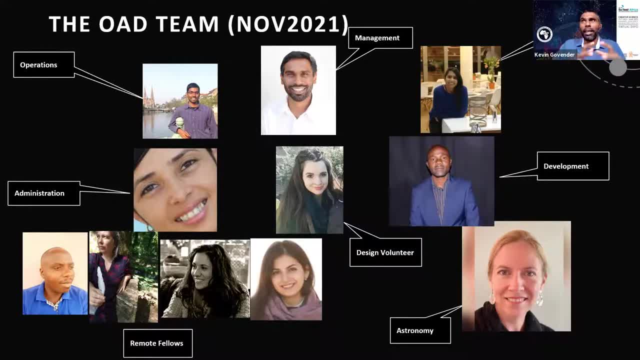 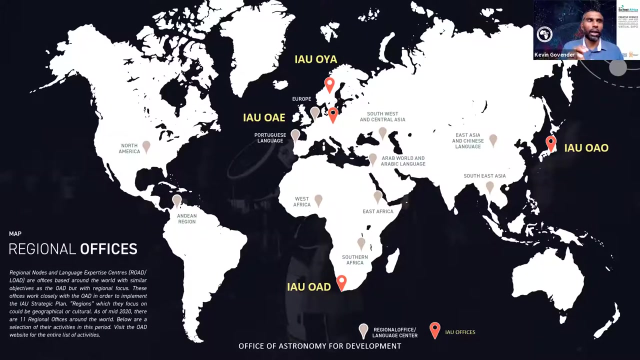 and everything that operates. the whole machinery of the Office of Astronomy for Development, or using astronomy for development, relies on this team- And a lot of these slides also come from my colleagues- And internationally, the structure is built on our regional offices. 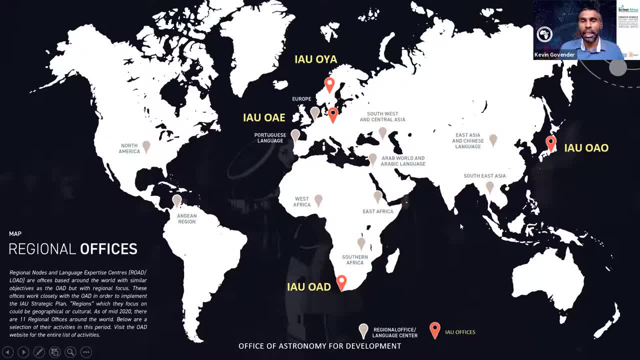 So we have, we've now established 11 regional offices around the world And each of these offices, they're basically sort of coordination points for astronomy, astronomy for development activities within their either geographic region- like you know, East Africa- or a language region. 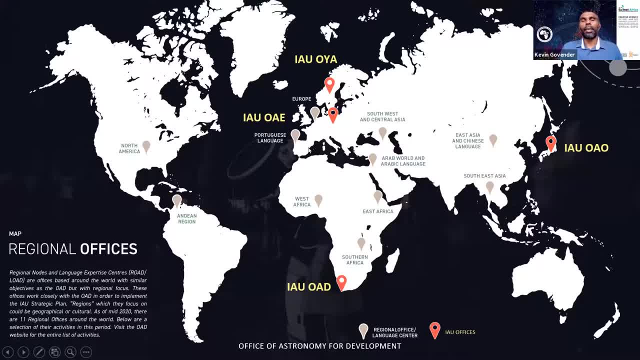 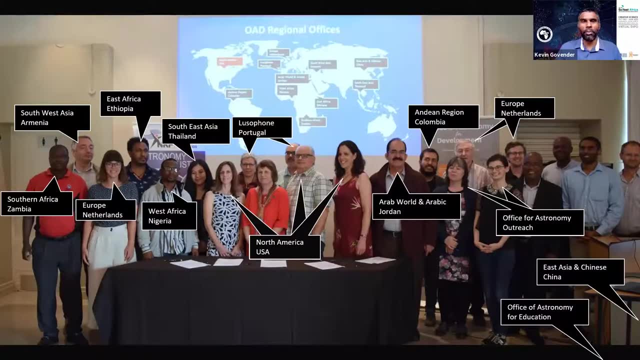 For example, the Portuguese language office works with Portuguese speaking countries around the world And these 11 offices form sort of the backbone of our activities globally. This was the last in-person meeting we had before the pandemic struck. It was in Cape Town when we launched the North American Office in January 2020.. 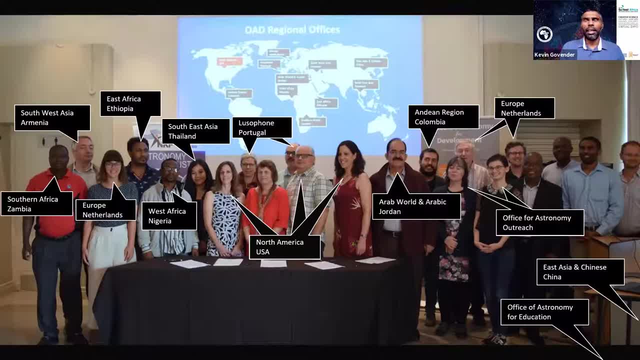 And you know, I should really say that an important lesson that we've learned over the years is that you know, I think, our country, South Africa- I'm South African- and our country has really got it right with our motto. 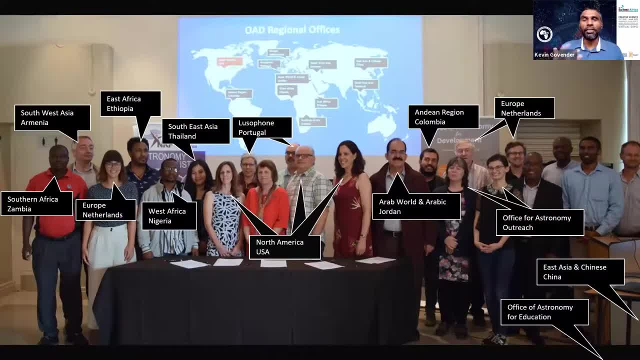 Ike, Tara, Ike, You know there's strength in diversity, There's unity in diversity And we find that globally, that you know, when we bring a diverse group of people from all around the world, you know ideas come from the Arab world. 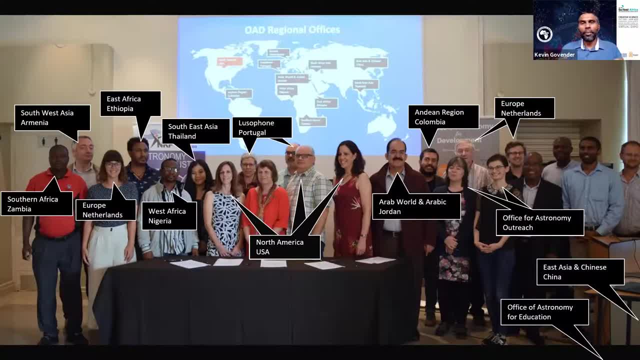 and ideas come from the East Asian region, and the European office brings something to the table and the South American office brings something to the table, And together we can put our heads together and our ideas together to make magic happen, as my colleague would say. 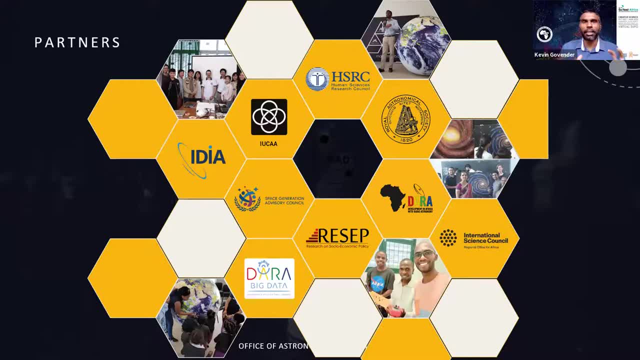 We also have several partners, So we look for partner organizations And this is important because if you're going to be creative about using your science, you have to be humble about it. You have to accept that you know you don't know everything. 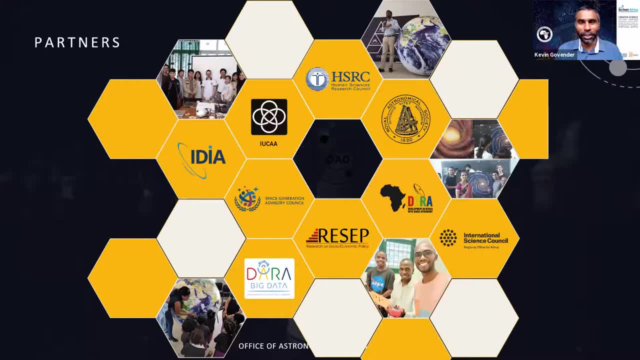 And if you want to apply your science for development, do you really know enough about development? You know in our field. you know we explore the stars. So what do we know about people? What do we know about challenges on the ground? 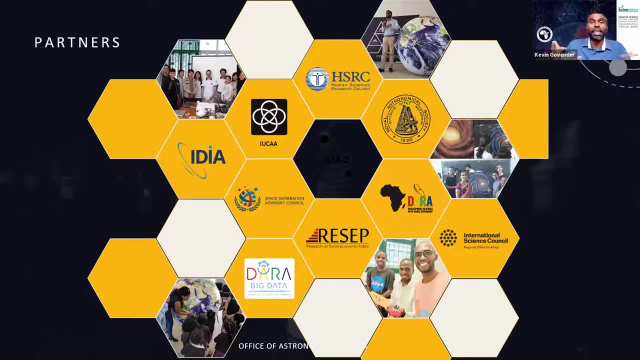 Some of us might have experience. but you know how do we make that connection? And we do that through partnership. So we've got, you know, partners from development, from the development economics field, from the space sciences, from the social sciences and from various astronomy institutions. 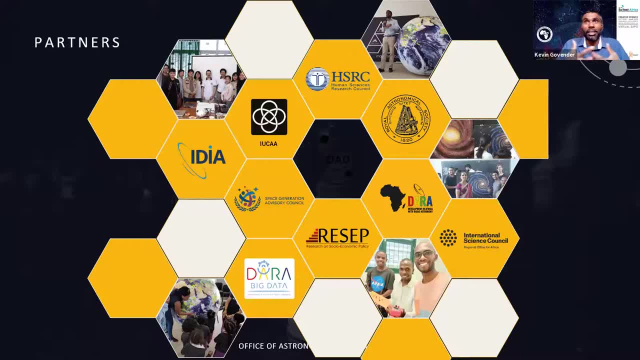 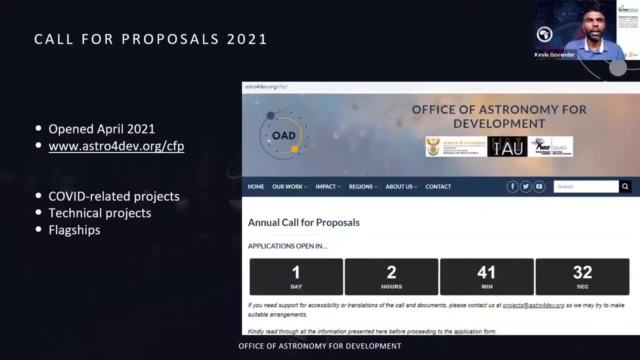 And this is something that gives us, gives us strength- is to constantly be open to partnerships beyond our own field of expertise. Now, when we say, you know, use astronomy creatively to impact on development, one of the biggest moves that we made. 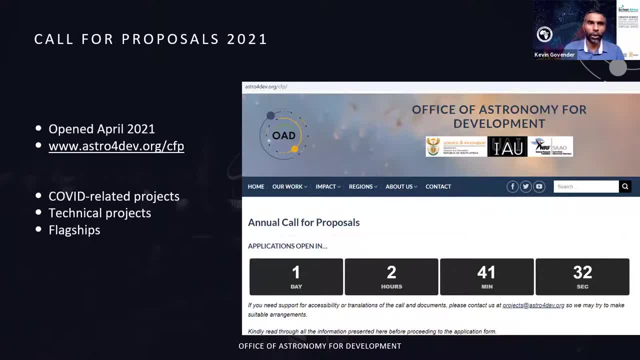 and it was a decision taken early on in the existence of OED- was to say: you know what? We don't know everything. Let's throw it out there and ask anyone anywhere in the world to give us their ideas about how they can use astronomy. 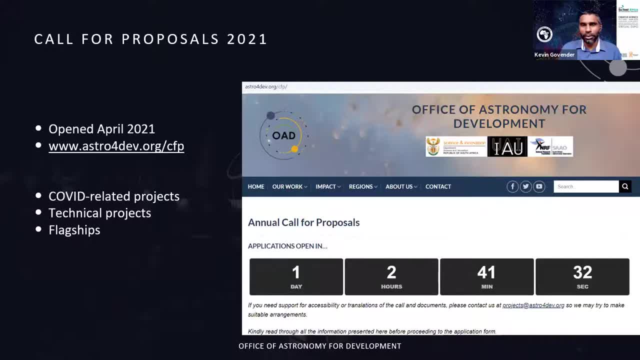 to impact their local communities or their environments, because they know their environments, They know the challenges that they face, And so they give us a proposal and we give them funding to implement their projects. So we have a call for proposals and it's been running every year since 2012.. 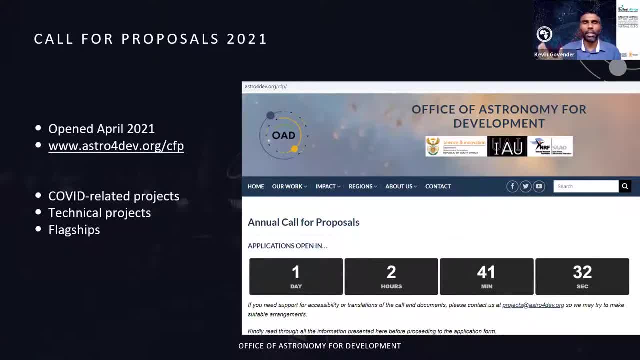 And this call for proposals is basically open to anyone, anywhere. It doesn't have to be astronomers, because we're talking about using the science of astronomy for development. It means that if someone outside astronomy, if someone in the education field, wants to use astronomy in some way, 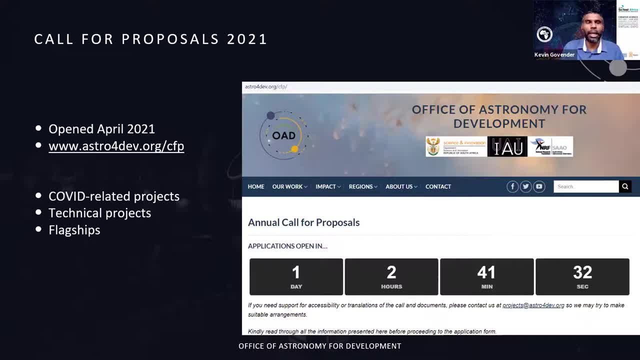 they can apply for funding to do that. And this is where you know the bulk of our activities go is in terms of getting people around the world to come up with ideas and we support them in implementing that project. And so, as Anya mentioned in the beginning, 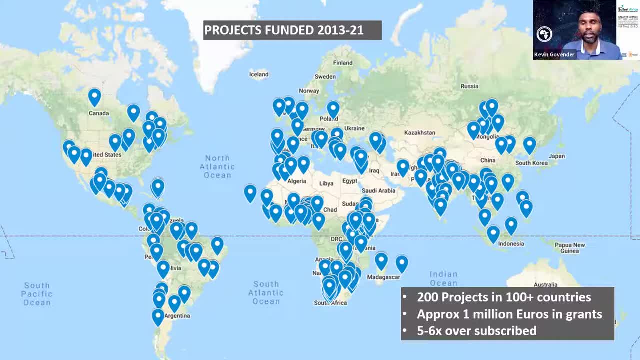 the projects funded so far. we've had about 200 projects reaching over 100 countries- well, audiences in over 100 countries. About a million euro was spent so far from the International Astronomical Union, But what's interesting is that it is constantly oversubscribed. 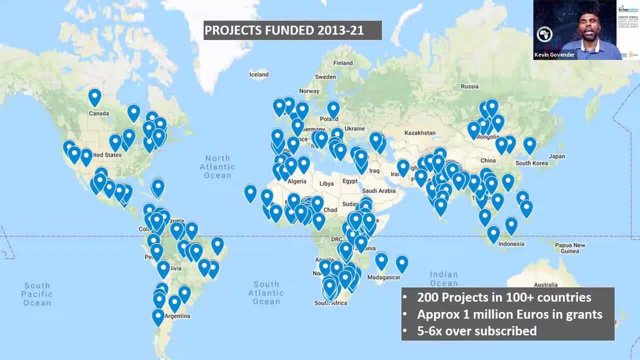 This call is constantly oversubscribed by five or six times. It means that you know there's always this demand. People have many ideas of how to use astronomy for development, And this is something you know we'd love to see in other scientific fields as well. 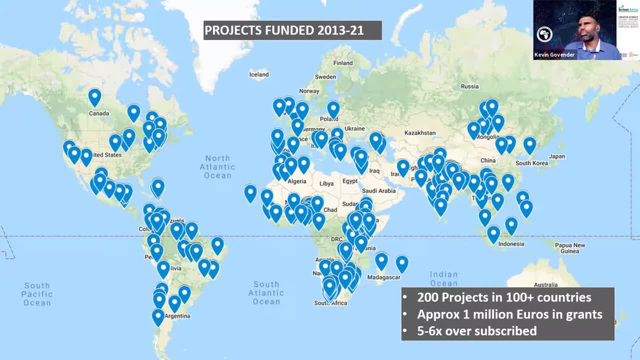 If you open up your field and you say you know, come up with ideas as to how you can use this field, this field of science, to impact positively on your community, to impact on the Sustainable Development Goals, see what ideas come up. 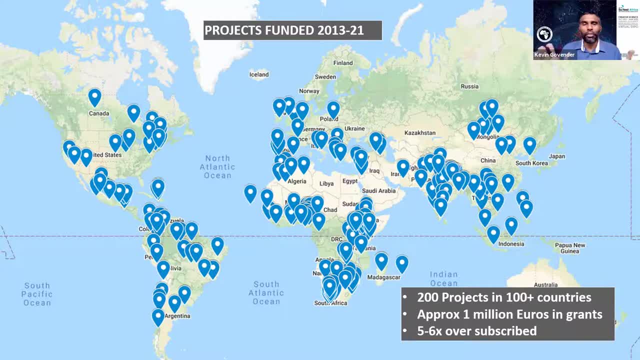 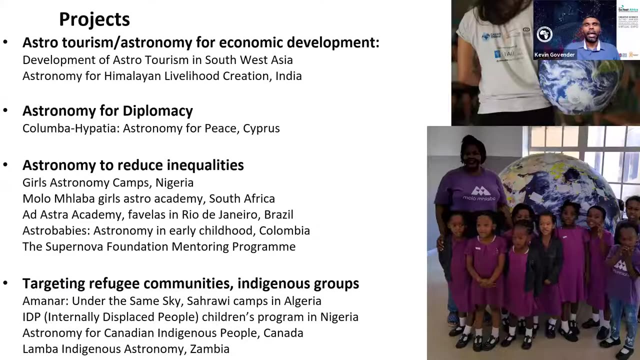 Because what we found is that we wouldn't have thought of half the ideas that people came up with, And it's those ideas that have enriched the idea of the whole principle of astronomy for development. Now I'll give you some examples so you get a sense of it. 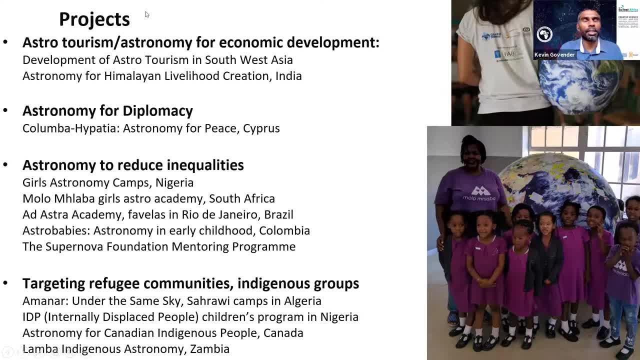 So some types of projects that we've supported: Astro-tourism. So how do you use astronomy for economic development? Using astronomy? you know the clear night skies, the fascination that people have with astronomy. Well, it happens that most clear skies are in very rural areas. 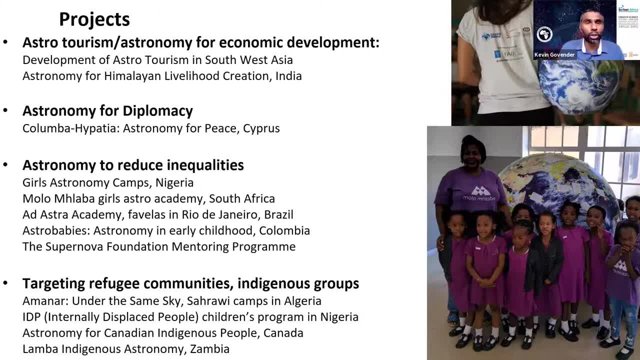 So how can we impact on those rural communities? by stimulating tourism and, in that way, economic development in the region? So each of these titles below are projects, And you can find all this on the OED website. Now, astronomy for diplomacy. 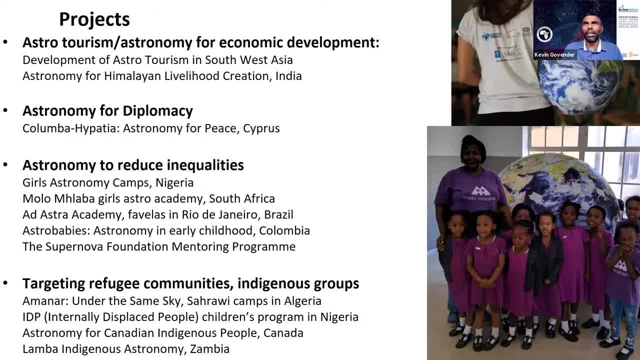 So, using astronomy and the perspective of, like you know, we all live on this planet And if you know that we are only on this planet- there's no other planet we can get to- We have to go to, We have to live together. 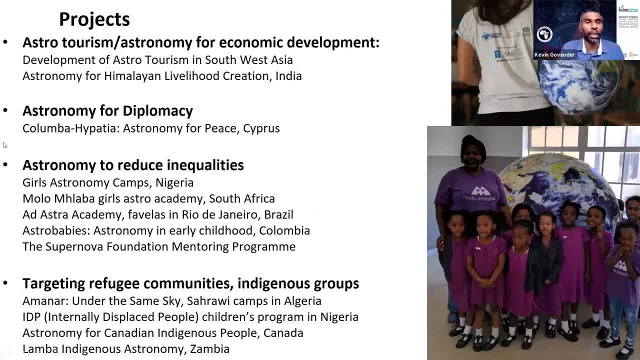 How can we use that for diplomacy? How can we use that to bring people together? Astronomy to reduce inequality. So, using astronomy to bring people together, whether it's marginalized groups or communities in different parts of the world, Astronomy is something that is fundamentally supposed. 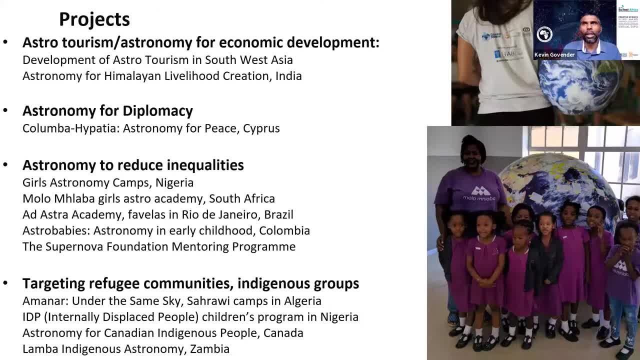 to be accessible. You know, everyone can look up at the sky, You can look up at the moon, You can look up at the stars. You can look up at the sun, You can look up at the moon, You can look up at the stars. 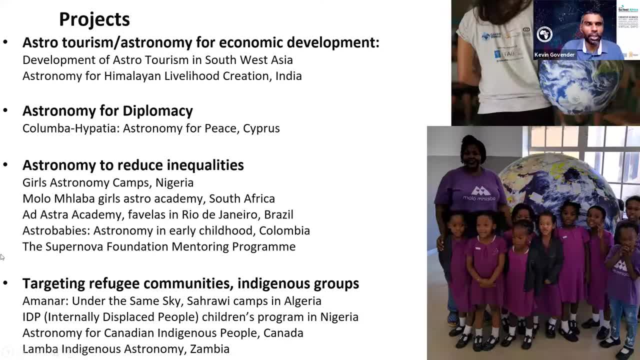 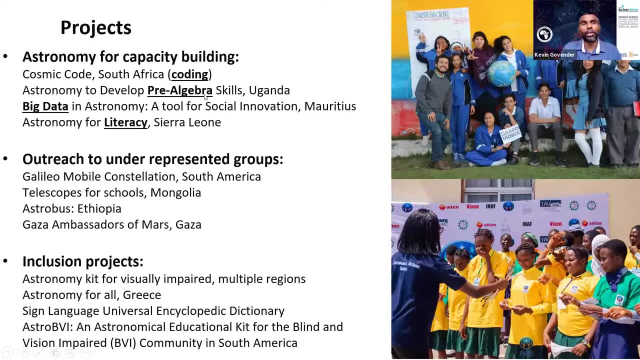 And so how do we bring people together around these topics? We've had projects targeting refugee communities, indigenous groups. We've had projects looking at using astronomy for capacity building, So coding skills, big data skills, even looking at literacy. We've had astronomy projects reaching out. 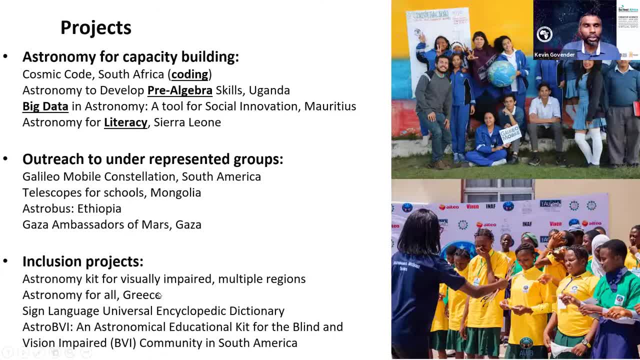 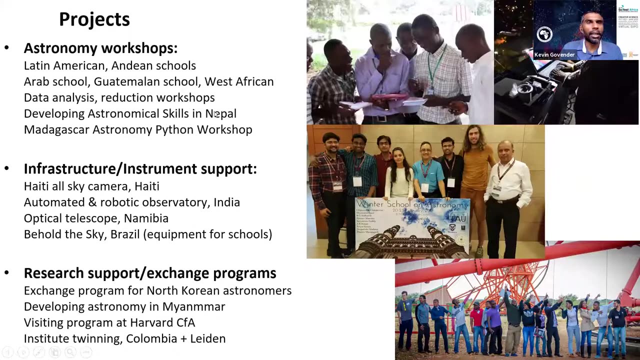 to underrepresented groups, Inclusion projects using astronomy for the visually impaired. So how can a person who cannot see, how can they experience the night sky? And so we've had projects like that, projects looking at sign language for astronomy. We've also had sort of university-level workshops. 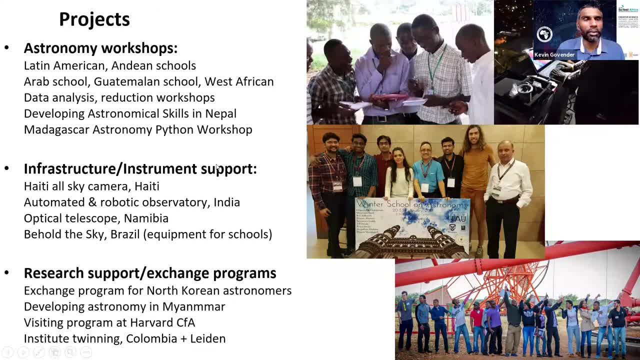 looking at skills, We've had skills development at university level. We've supported infrastructure like small telescopes, CCD cameras, instrument support that stimulates capacity building and research. And then we've had exchange programs, where we support the bringing together of astronomers, scientists from different countries. 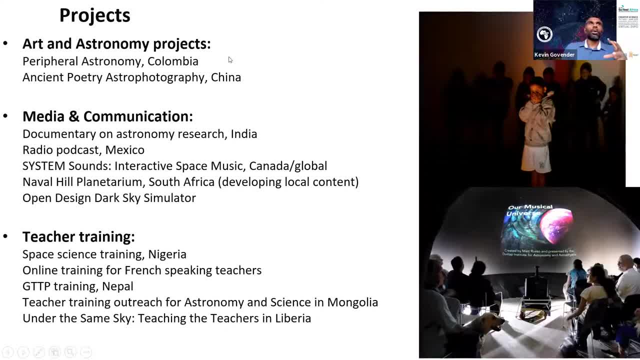 So we've taken art and astronomy projects. So using art with astronomy to inspire people, Media and communication- Astronomy is one of those fields that somehow attracts a lot of public attention. And then teacher training projects as well. Now, from all these projects, 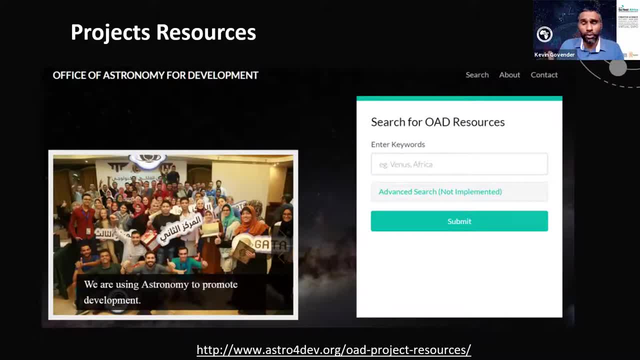 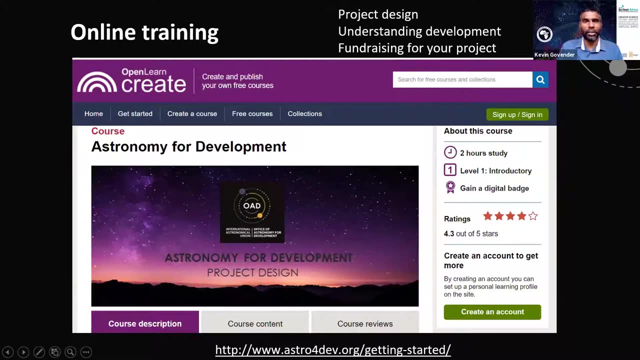 each of these projects will have resources, So we've taken resources from all the projects and put it onto a database so that other projects can now build onto these resources. We also have online training. So, in terms of how do you develop a project around astronomy for development? 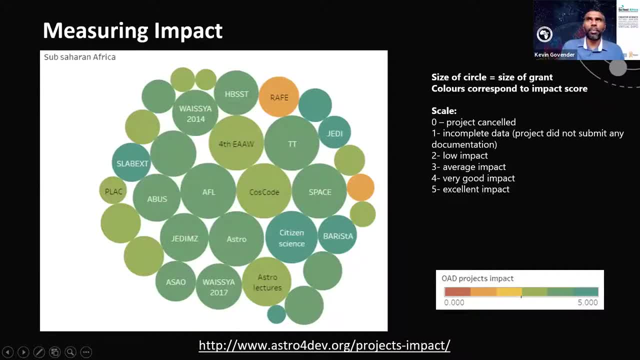 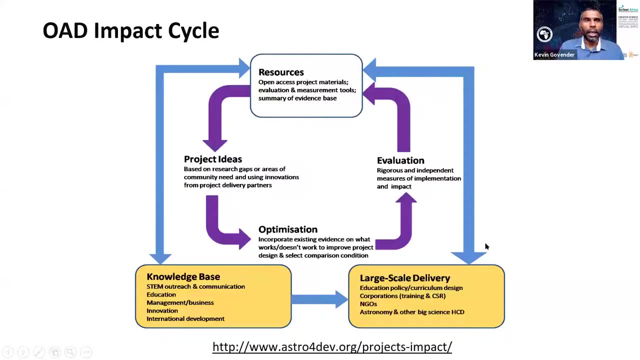 And then we've had some reviews of what the impact has been thus far in terms of using astronomy for development. So what's the impact of our past projects? So you'll find all of this at the website below, astro4devorg. Now, when it comes to impact, you know, 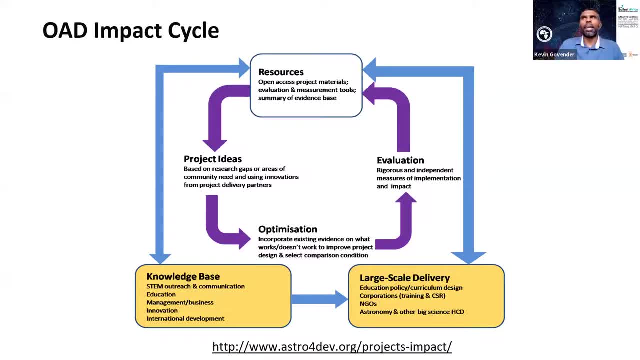 when we talk about using any science for development, you know, big question is: are we actually making impact? And so what we've developed is this impact cycle. So these project ideas that I said come from all around the world. Well, we have a phase now where we try to optimize. 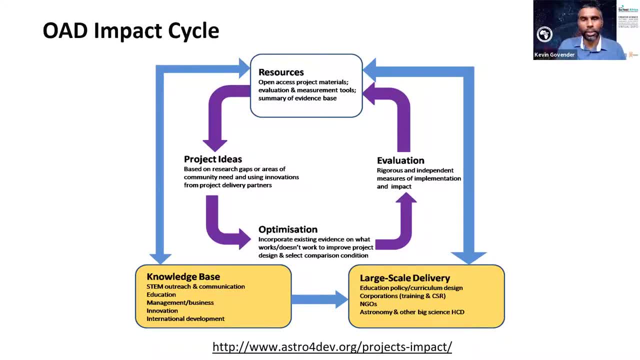 those projects. So there's two stages in our proposals process And then we allow for a space for projects to build in evaluation into their projects And once this is done it feeds a resource bank that then goes into a broader cycle. But basically, new projects build on the resources. 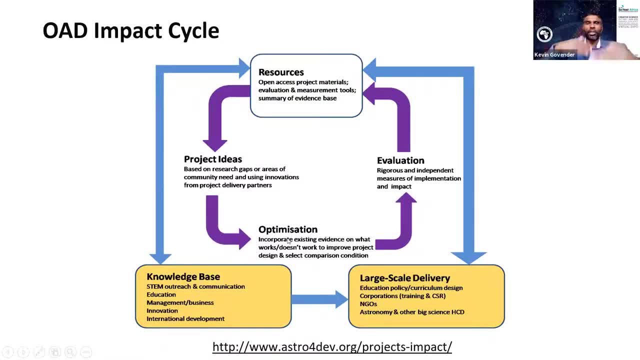 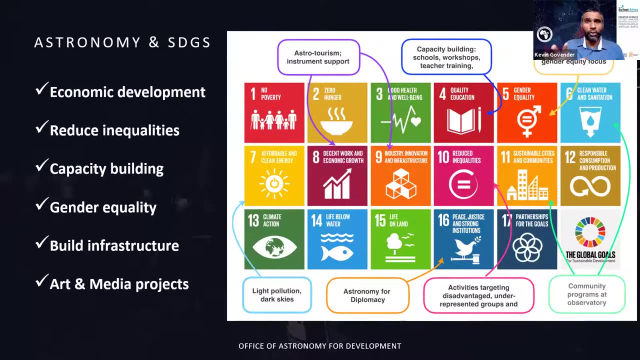 developed by past projects. So you constantly have this positive impact and a positive feedback loop And ultimately, these resources should feed a broader, large-scale delivery. Now that's where we get the idea of: you know, let's take the best of what we have. 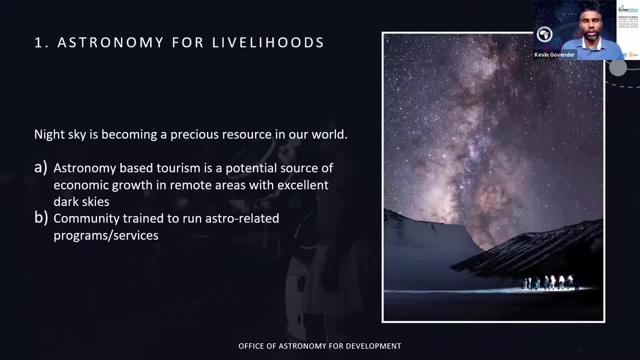 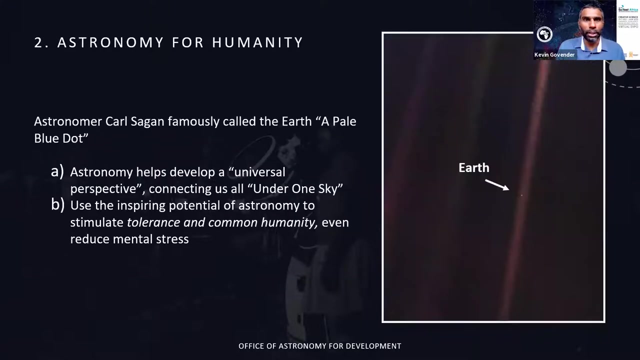 and let's now develop flagship projects. So I'll now mention three flagship projects. One is using astronomy for livelihoods. I mentioned about the tourism, So this is now trying to benefit rural communities from tourism, to stimulate tourism And that tourism brings income to rural communities. 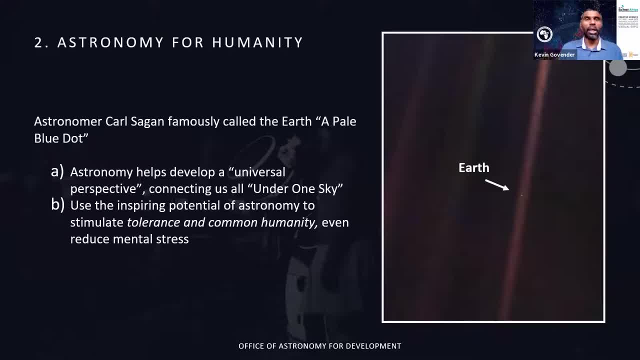 The second one is about using the inspirational aspect of astronomy. So we look at, you know, the inspiring power of astronomy and see how we can bring people together and stimulate a sense of tolerance and common humanity. And a big aspect of this is how can we potentially use this? 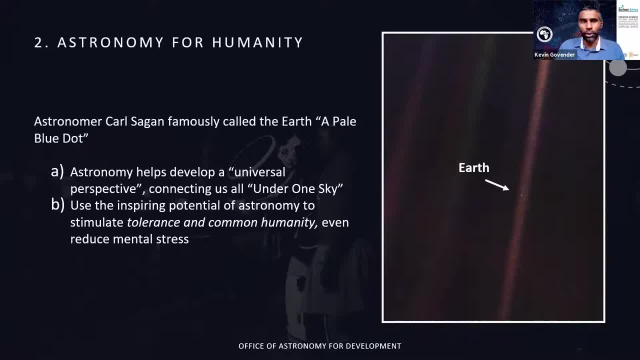 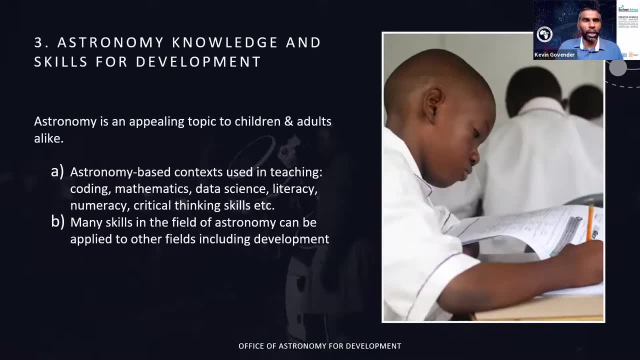 to reduce mental health issues as well. Then astronomy: using astronomy, knowledge and skills for development. You know, astronomy is something where there's big data challenges that we tackle in astronomy. How do we use that to stimulate capacity development in that area? 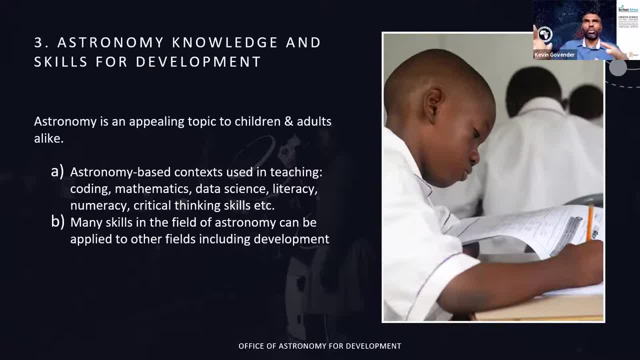 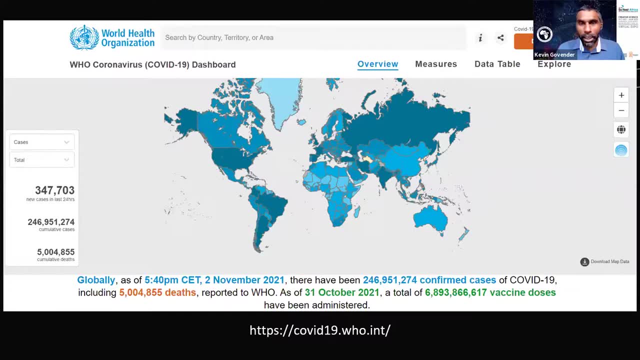 So these are now these flagship projects which we're trying to, you know, pull out of these many projects that we fund and then grow those, And then the pandemic hits. So you know, we can talk about SDGs and all these things. 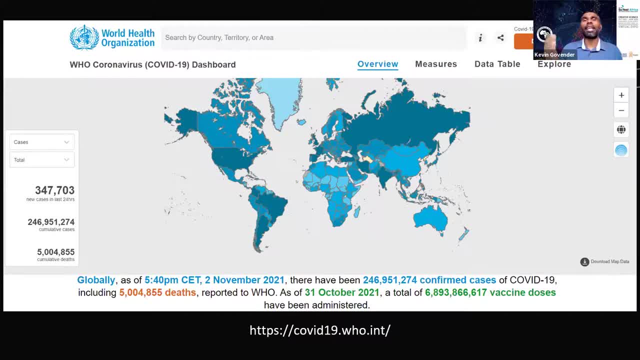 but you know, at the end of the day, we're facing very current challenges And the pandemic was one of those situations where, suddenly, our projects can't be implemented. Suddenly we find ourselves. well, you know, we're planning all these events. 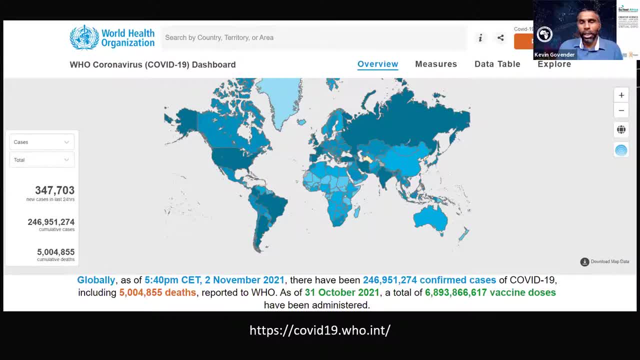 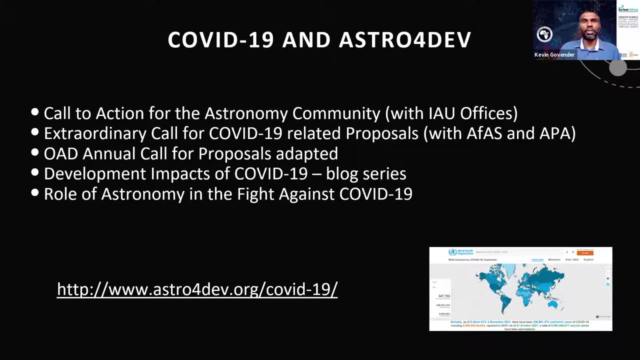 and activities. but it can't happen, And so we quickly sort of adapted our whole call and we changed things In 2020,. last year we had a special call for proposals that asked specifically for projects related to the COVID-19 pandemic. 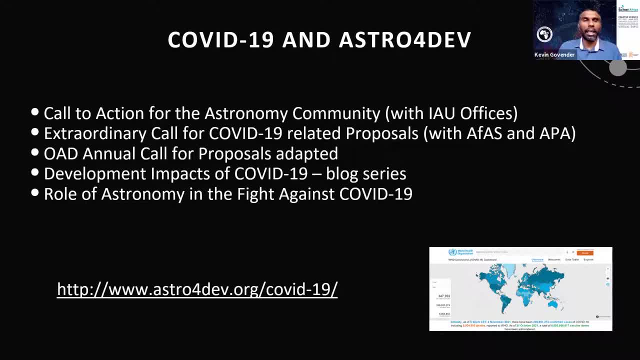 And that was done amidst, you know, several other activities where we adapted our projects. we adapted our annual call, we looked at the developmental impacts of COVID-19, we had a fellow do a blog series on that- and look at the role of astronomy in the fight against COVID-19. 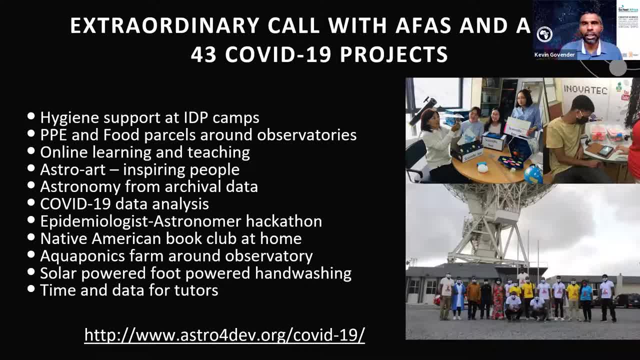 And so this extraordinary call. we partnered with the African Astronomical Society and African Planetarium Association and we had 43 COVID-19 related projects And these dealt with. you know some of the challenges that we face, whether it's using PPE, online learning. 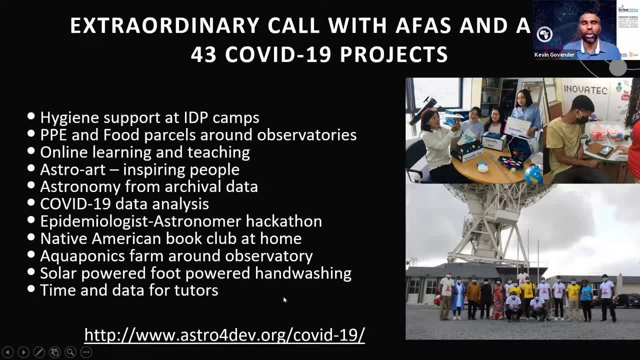 even using seeing how astronomers could help with the analysis of epidemiology data. So you know, as challenges hit us, we need to ask the question: how can our field contribute? And asking this question widely to the community, globally, is a way of bringing out these ideas. 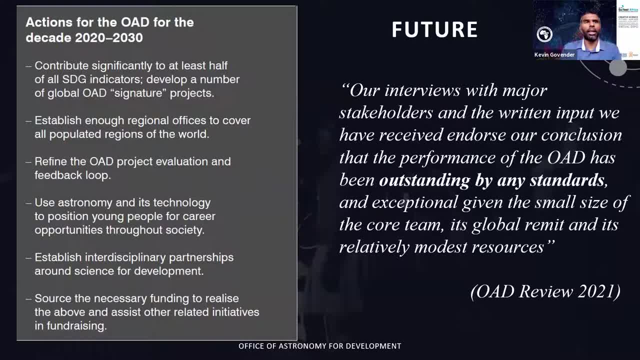 So I'm going to just jump to the future now. So where are we going with this? So, in the International Astronomical Union Strategic Plan, there's very specific goals that we're talking about when we talk about using astronomy for development, And you know so far. we had a review in 2021,. 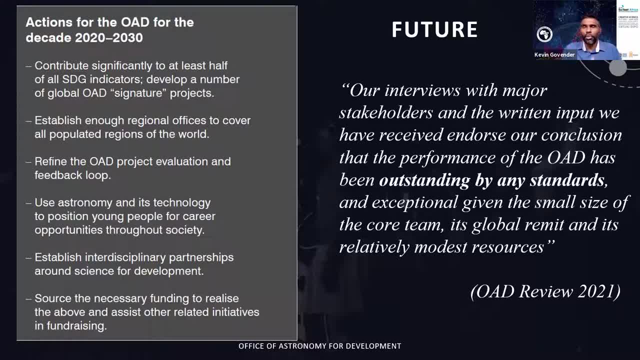 and the work of the OED has been lauded. as you know, the words they used were outstanding by any standards, So we're on the right track. We have now. we're now in a stage where we've managed to develop this idea. 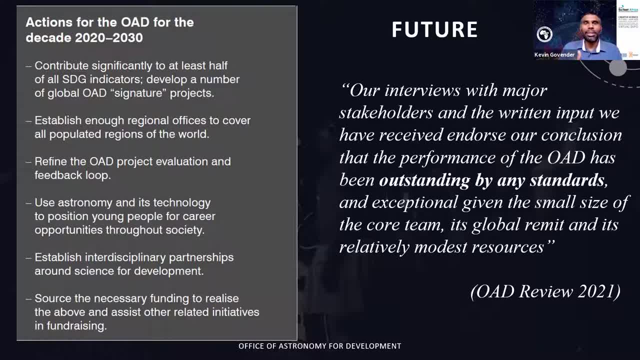 of astronomy for development. We've managed to stimulate a global community, And now how can we take this to the next level? How can we raise, you know, millions of dollars, euros, rands, to make big activities happening, to make big activities happen globally? 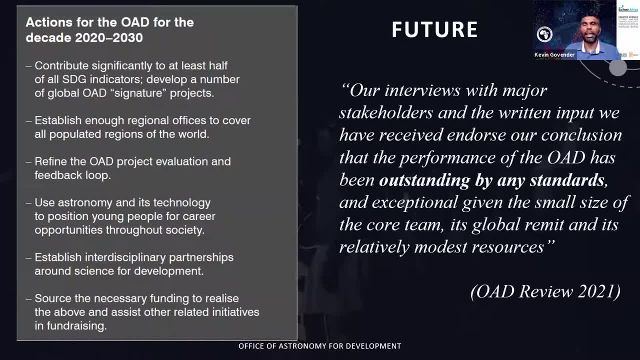 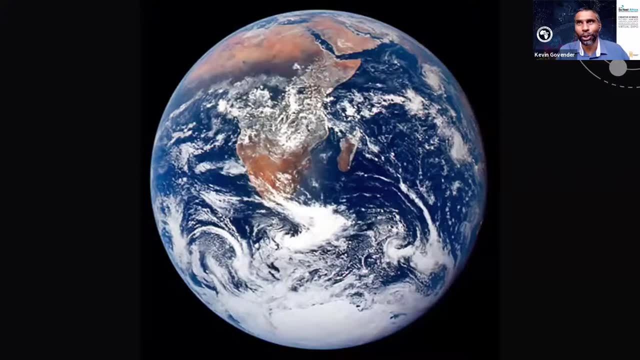 And we use the structure of our regional offices and in that way try to have the biggest impact on development. So I'm coming to the end of my time, So I want to just pause a little bit and sort of reflect with you that you know talking about science for development. 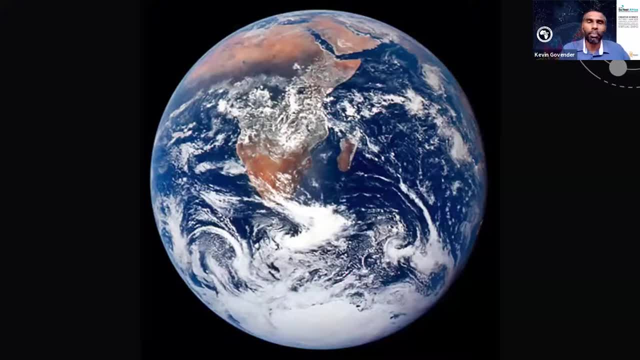 talking about how we can play a role in making the world a better place. it's important to sort of reflect on our place in this world And this image that was taken by chance actually from one of the Apollo missions, you know. 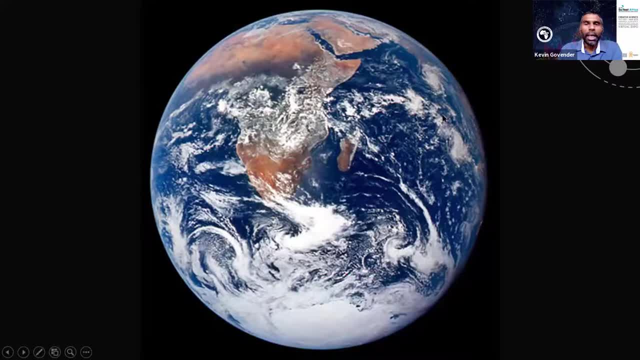 it's one of the most widely shared images, called the Blue Marble, And it gives you a sense of the fragility of our planet. The atmosphere, the entire atmosphere that sustains us is a really thin sheet around the edge of this Blue Marble. 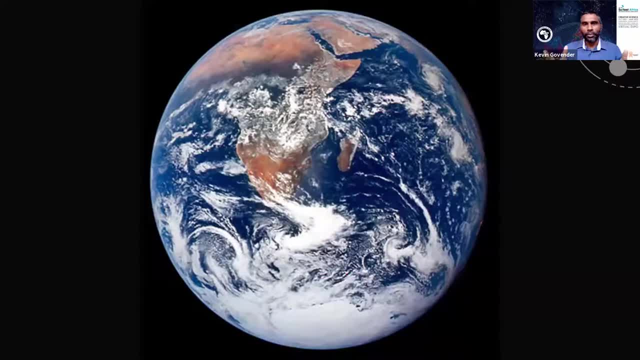 And we're on this planet together. So how do we, how do we as individuals, contribute to making this world a better place? Well, this perspective that astronomy gives, that you know knowing of where we are in the, you know, bigger scheme of things, 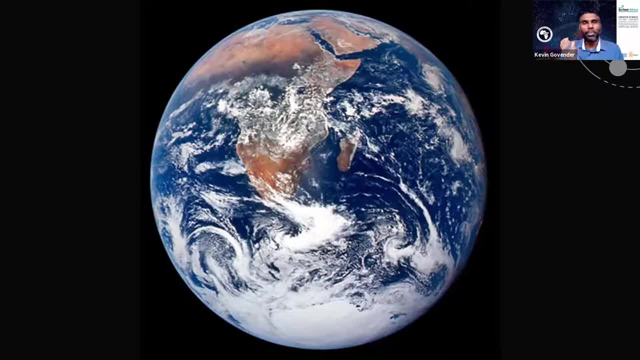 this is a perspective that is worth spreading. It's a perspective that you know all people need to realize: that when you look at the Earth from space, you don't see the country borders, You don't see skin color, You don't see political affiliation. 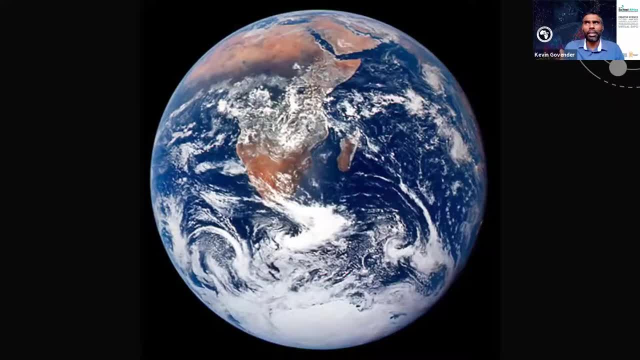 These are things that we've created as human beings. But you know, more importantly is what we have the potential to do as human beings. We have the potential to reverse climate change. We have the potential to stop the conflicts that we have around the planet. 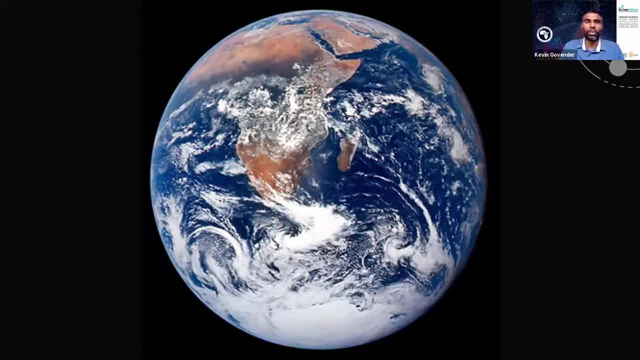 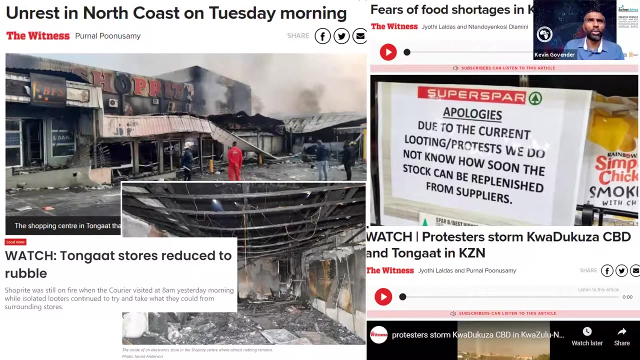 We have the potential to create technologies that will make this planet better. And when we see on the news, you know the challenges that we face. you know you all would have followed the unrest that we had in South Africa earlier, a few months ago. 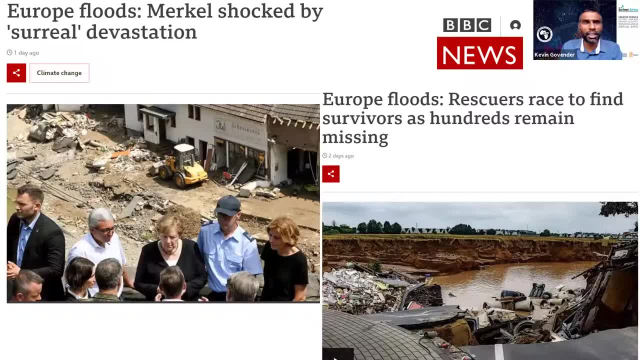 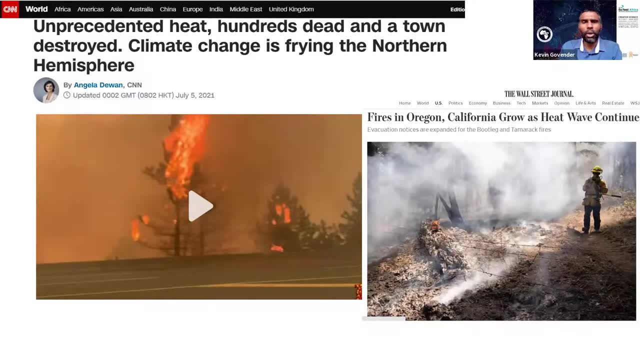 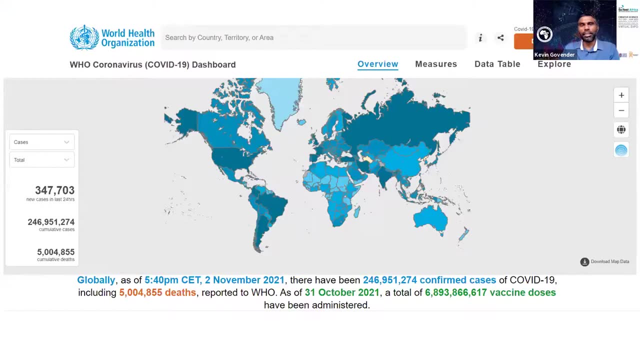 in Europe. they've been struck by floods. There's been unprecedented heat waves in different parts of the world. We are facing so many challenges as humanity, But if we don't see these challenges as something that needs to bring us together, like the pandemic, 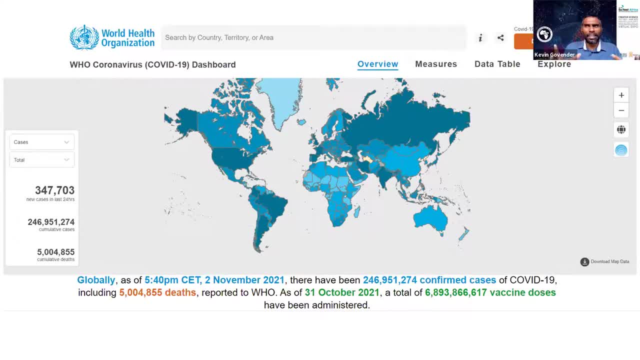 and the pandemic which you know really should have brought the world together. it didn't necessarily achieve that. You know, we have this huge inequality in vaccines And we have to ask ourselves why? Why, when we see these challenges. 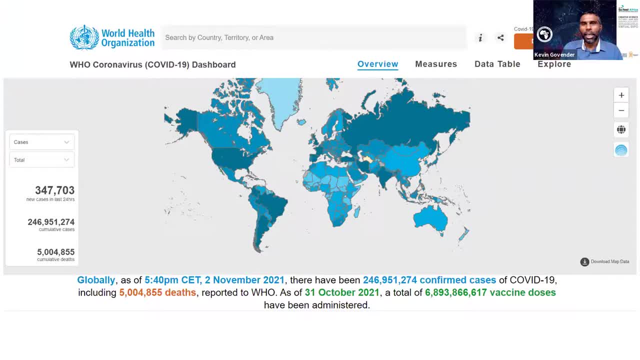 we are not more empathetic towards our fellow human beings And maybe, maybe astronomy could be that that could bring us that perspective that we need to be able to work together to be able to overcome the challenges and see the challenges faced by our fellow human beings. 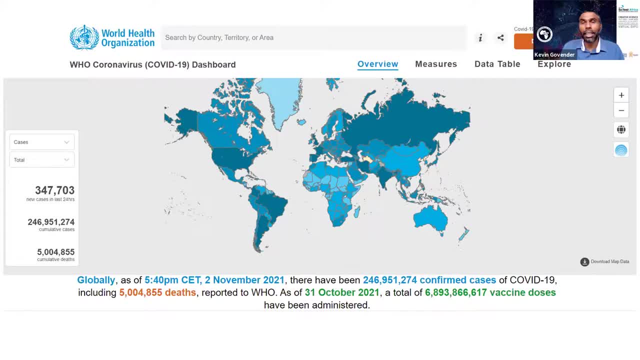 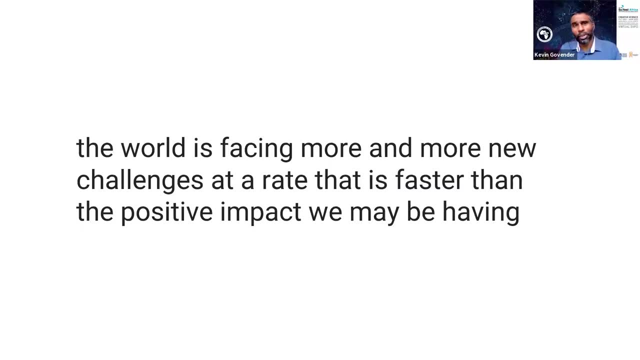 as challenges that we face, And these challenges are coming at a fast rate. You know the world is facing more and more new challenges at a rate that is faster than the positive impact we may be having. So we need to, we need to step up our game. 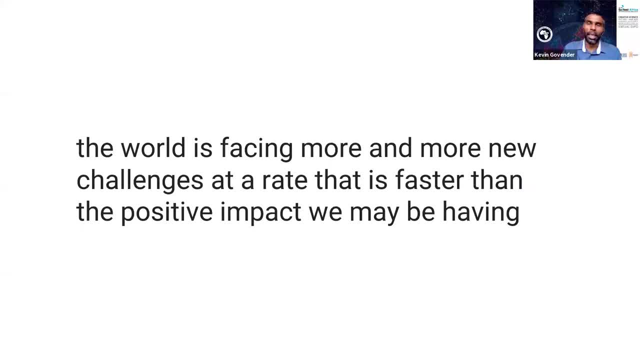 And maybe you know, if we can rally our sciences together, we will be able to overcome the challenges that we face. And if we can rally our sciences together, then we can, we can help to keep up with the pace of the challenges that we are constantly facing. 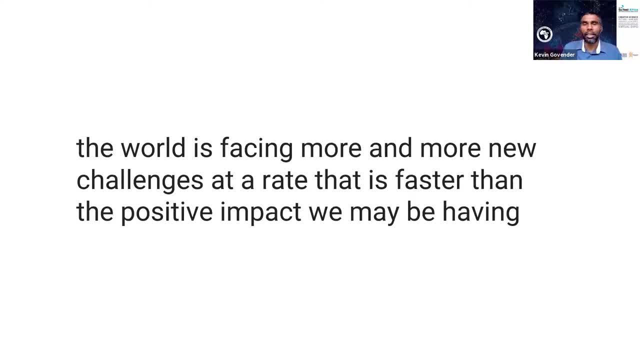 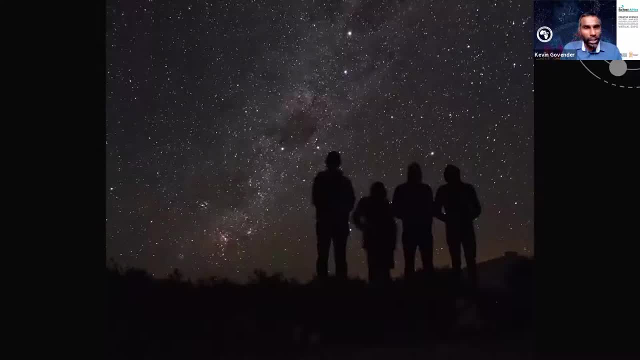 and will face as the climate changes, as society has changed, And so you know, when you look at the sky again, and you see that, that you know this, this space that we float in, float in, and you see that it's changing. 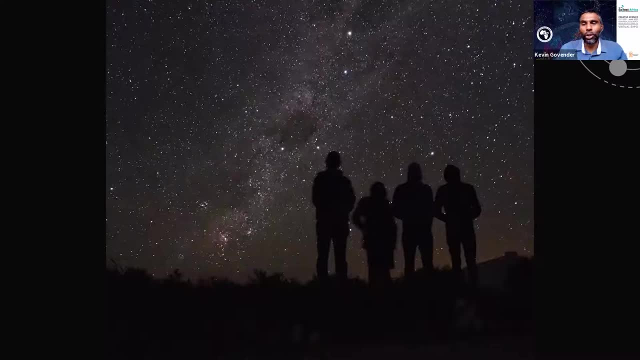 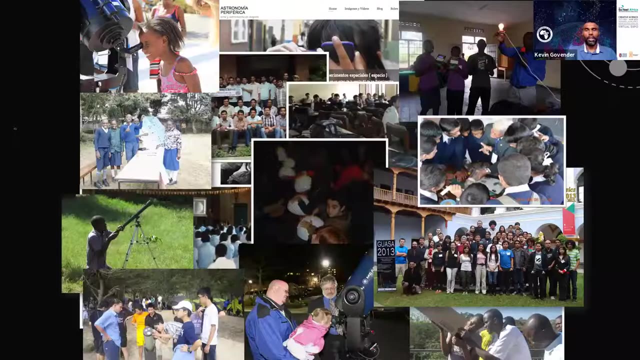 Think about what the Earth would look like from space And think about what role you could play and your field could play to make the world a better place. So with that you know- just to acknowledge that you know- a lot of the work that we do. 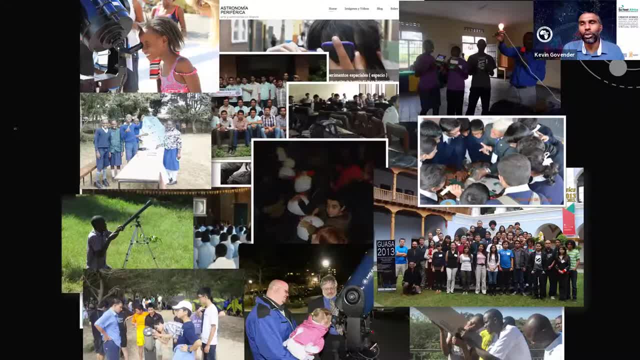 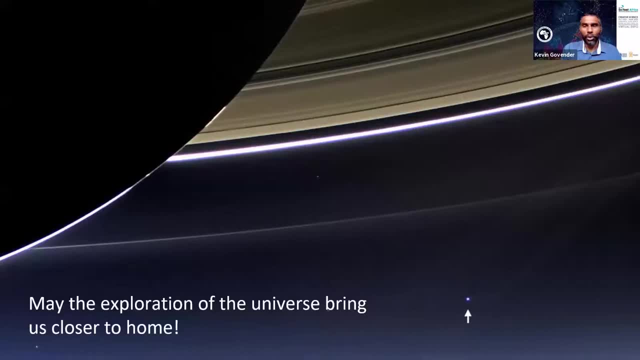 well, all of the work that we do in terms of the astronomy for development credit goes to the projects that we support around the world and our regional offices. With that, I'll leave you with this message. This is a picture taken by the Cassini spacecraft. 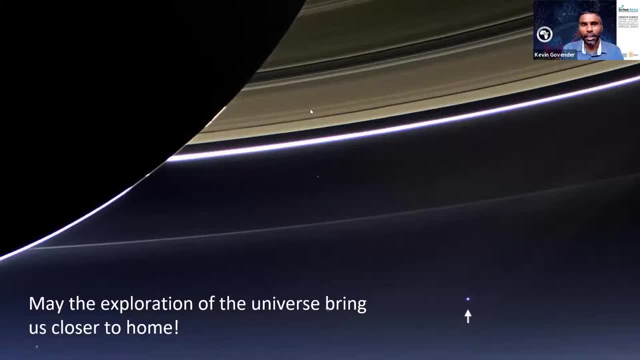 And that is planet Earth. This is when the spacecraft was near Saturn. It took this picture of planet Earth And it was promoted as the day. the Earth smiled And, you know, people on Earth were asked to look at Saturn and smile. 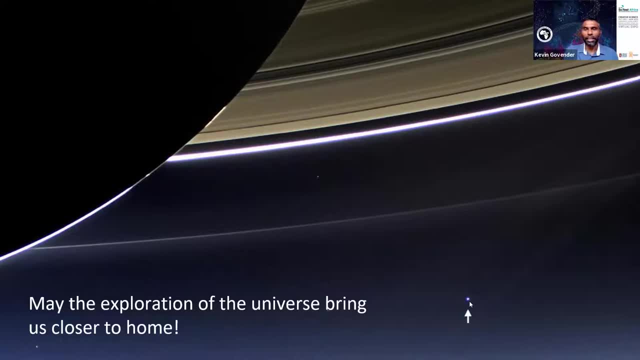 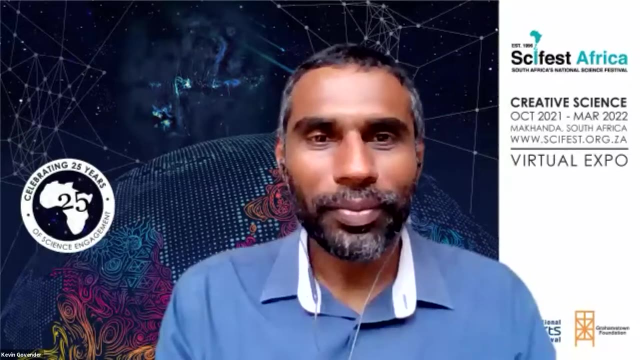 And this Cassini satellite took this picture, And that is our planet. That is everything that we have. So, as we explore the universe, let us keep our feet on the ground. Thank you very much. Thank you very much, Kevin, And it's always such a delight listening to Kevin. 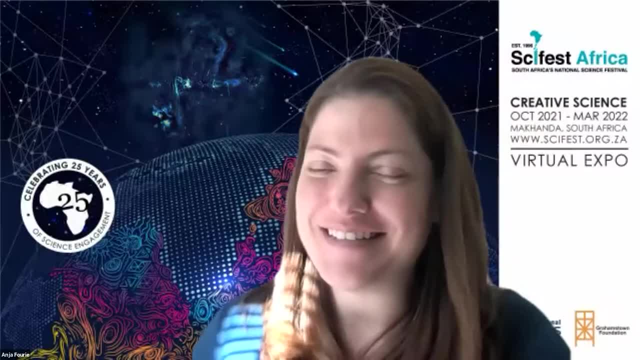 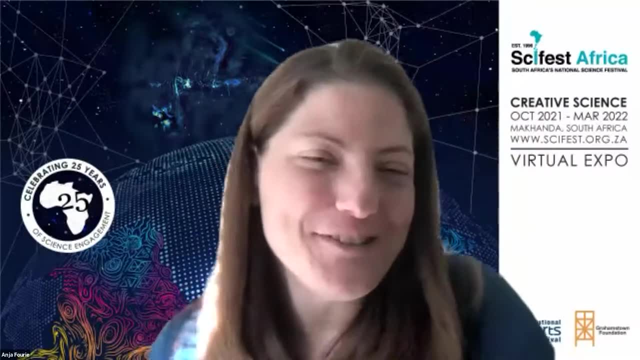 because you know, it just speaks to my heart and the work that I do. And you know, even after hours, Kevin, you know, just one session with you is always enough to inspire someone to keep doing what they're doing. 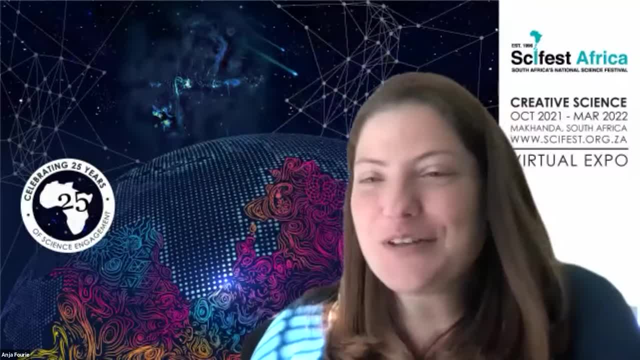 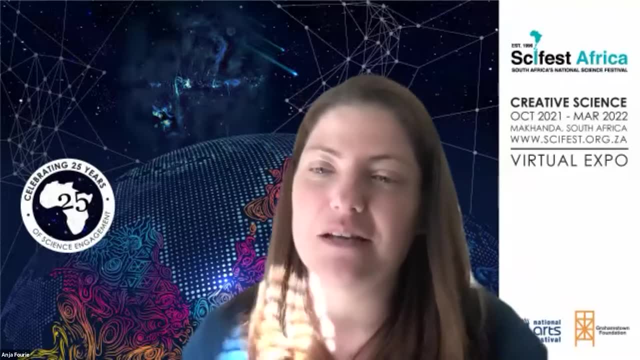 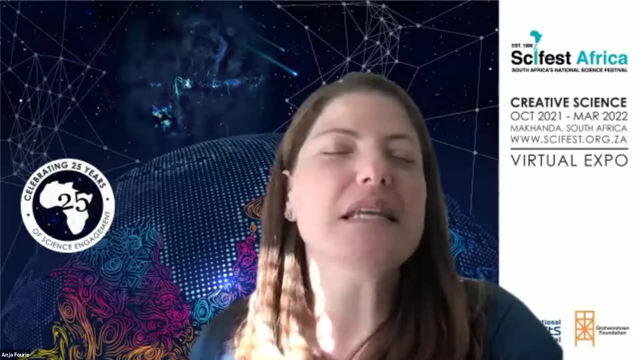 So I'm going to go over to some questions. So you know, Kevin, those of us who work in science, you know often, especially if we, sort of, you know, want to work in development, or we can see the value, 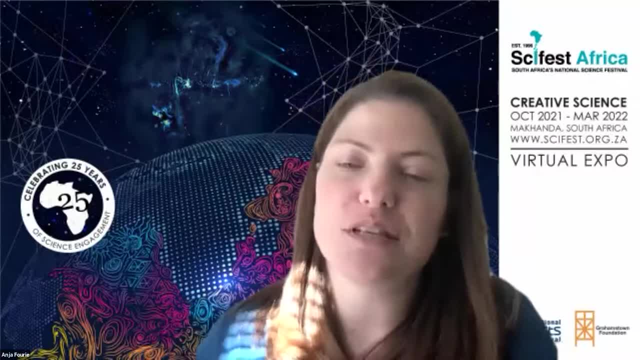 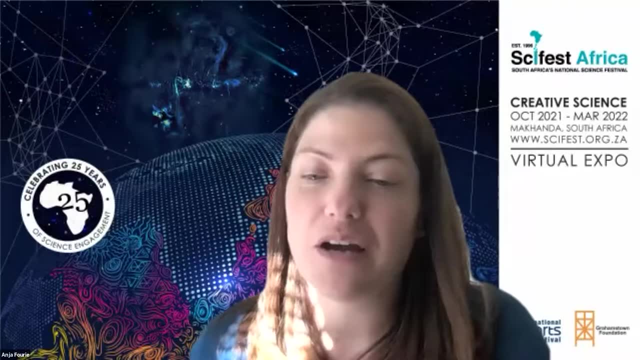 of the science. you know that we are doing and how we can use that for development. But sometimes we work in environments, you know, with scientists, or you know people who have been around for a long time And they're very focused on their science. 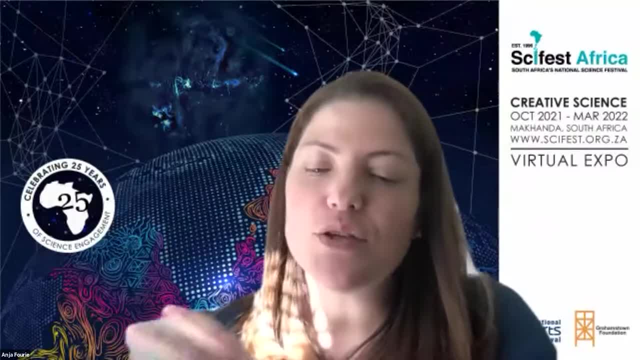 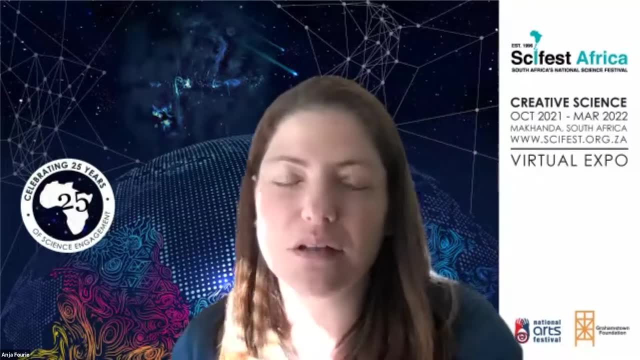 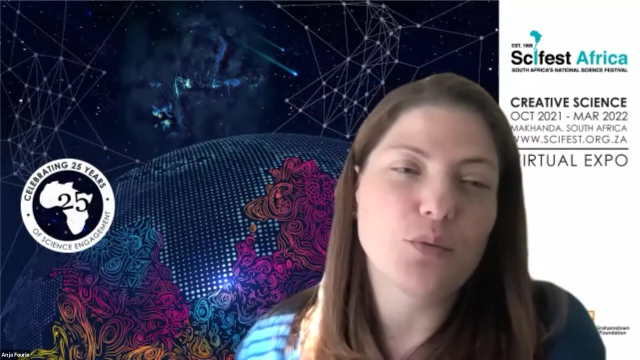 very focused on their research, And so using that science or sort of sometimes thinking outside the box of how to use it for development, is not part of an organisational culture. What is your advice, or what are your recommendations, you know, for audience members who work? 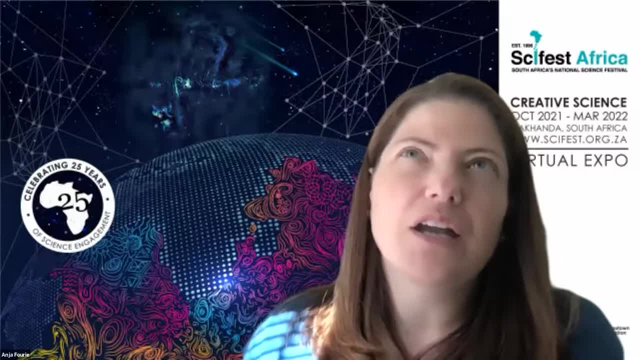 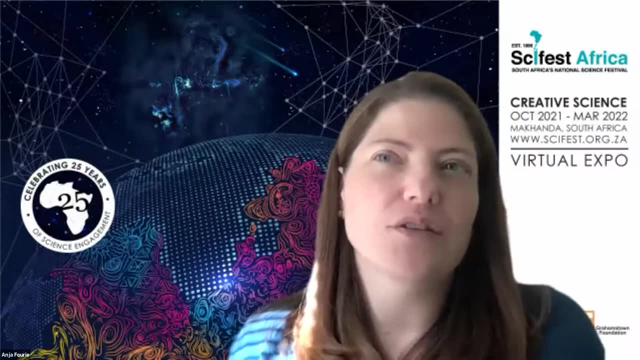 in that kind of environment. How do you? you know how do you motivate other staff members, or you know how do you persuade them to just look a little further and try and use what they're doing for development? That's a great question. 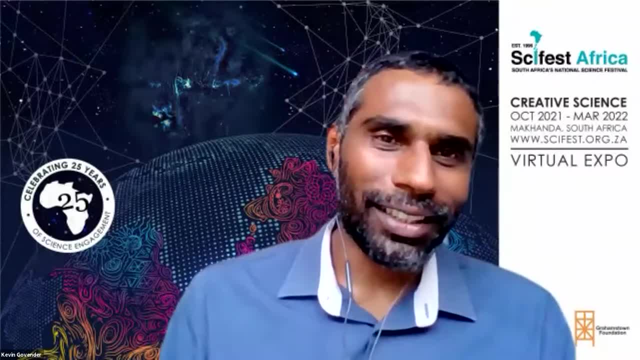 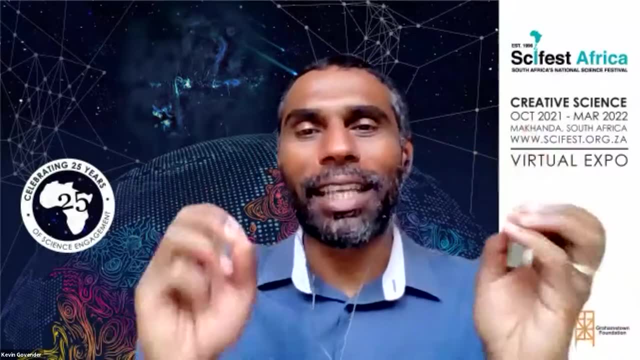 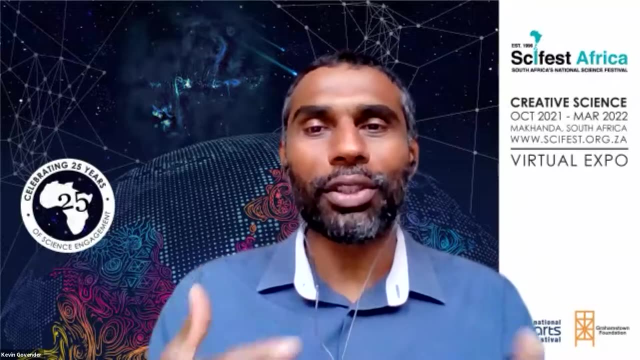 I think it's important to realise that the world is changing in favour of a science that has impact. So you'll find more and more nowadays that there is a demand from funders of science to organisations that they need to show what they're doing. 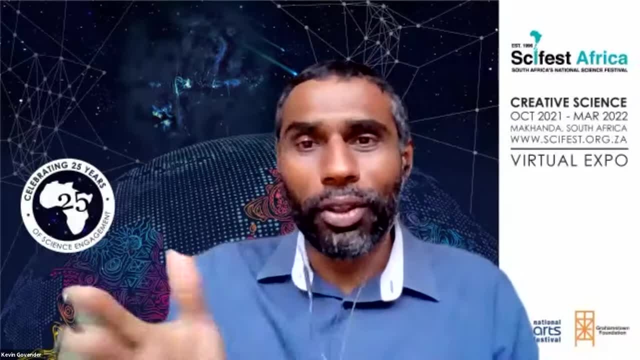 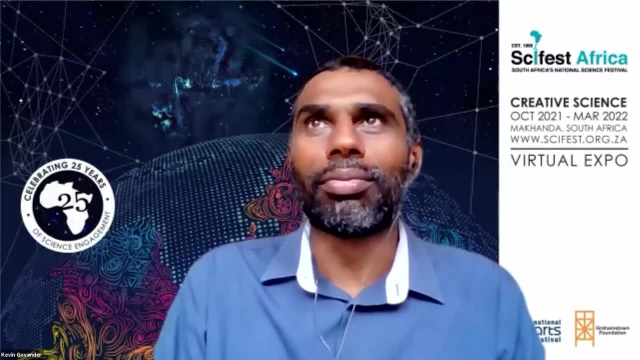 They have societal impact. Now, this has been coming for a few years now, but you'll find it more and more where you know it's not just about you know, sitting in a lab somewhere and doing your science and not worried about the impact. 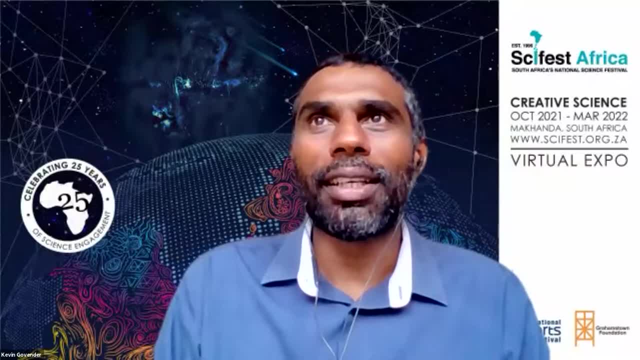 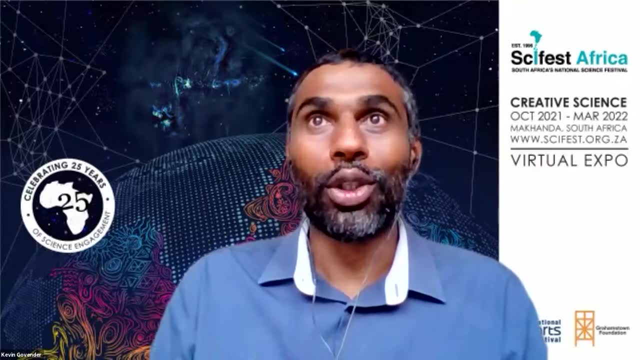 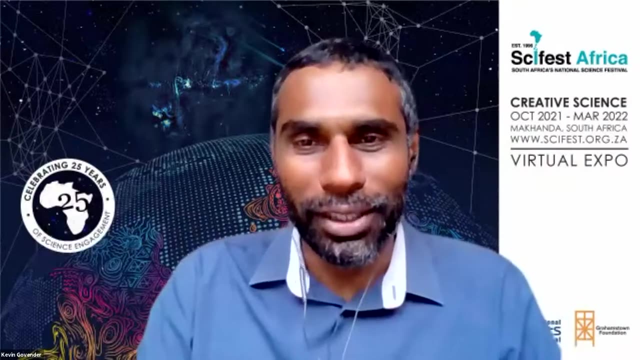 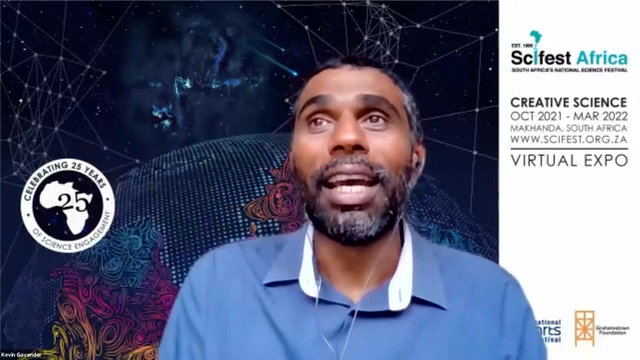 that you're going to make More and more as the pressure on governments increase to use funding to address these topics, these challenges. they pass on this pressure onto the scientists as well, And so those scientists or those environments that you find yourself in, people, in those organisations. 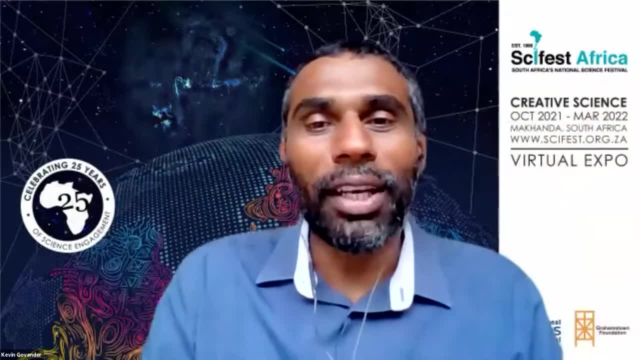 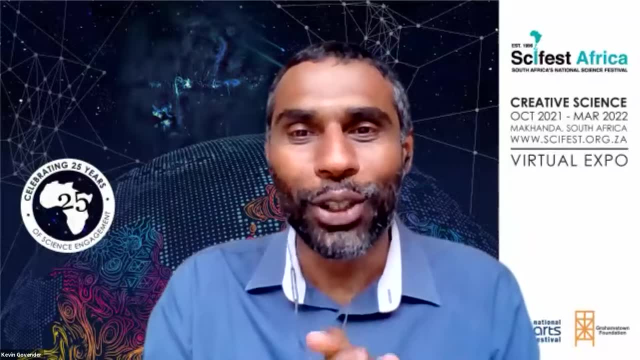 if you go to your organisation heads or whatever and say you know, what can we do to impact on society, the chances are they're going to say, yes, please help us because we need to come up with these things. That is where we are at the moment. 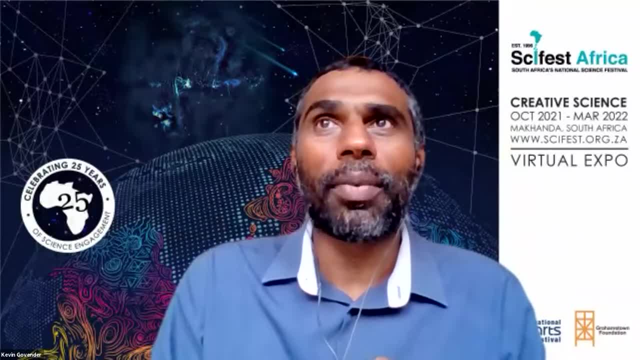 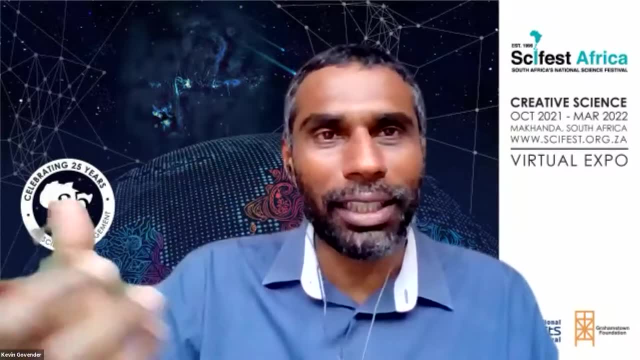 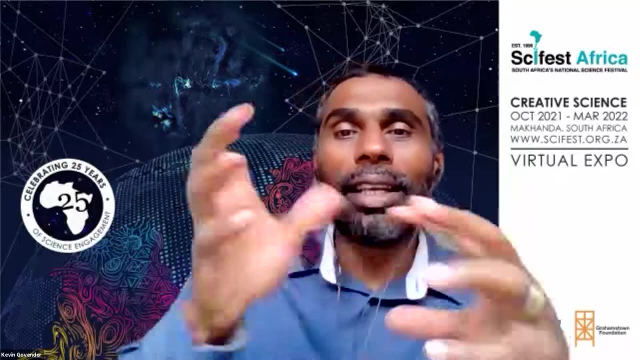 It's a very positive place, But you know the National Research Foundation, for example, which follows the National White Paper on Science and Technology, all of these policy documents you find in South Africa at the moment is really looking at science for development. 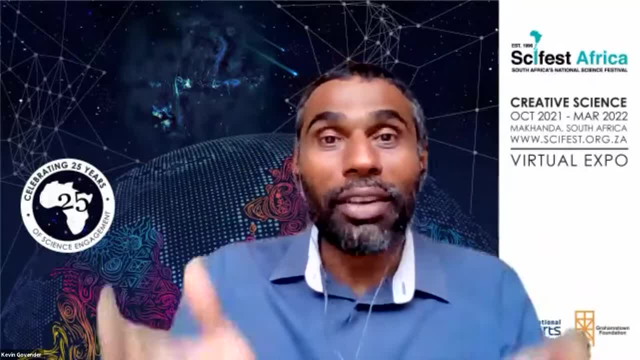 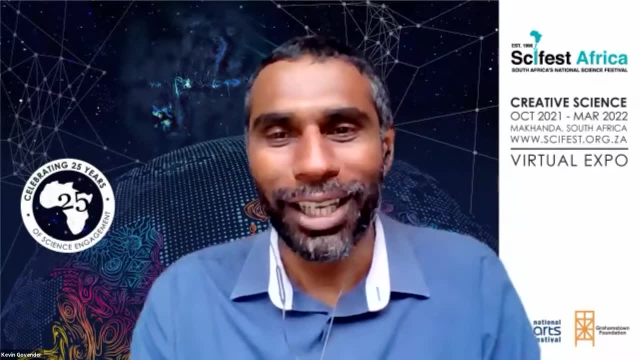 How can science impact on society? So it's a good environment for you to start your conversations within your institutions, because the chances are they are going to be very happy that you started it, Very eager for some ideas on how to do that. Thank you very much. 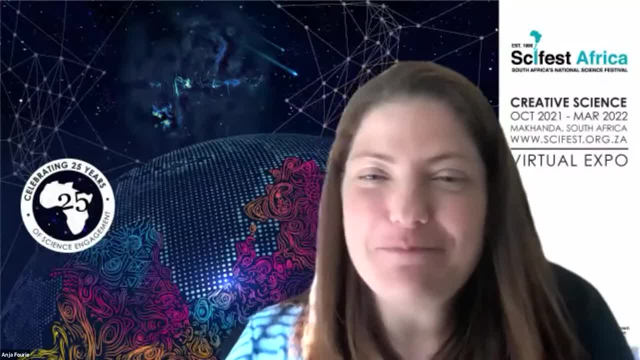 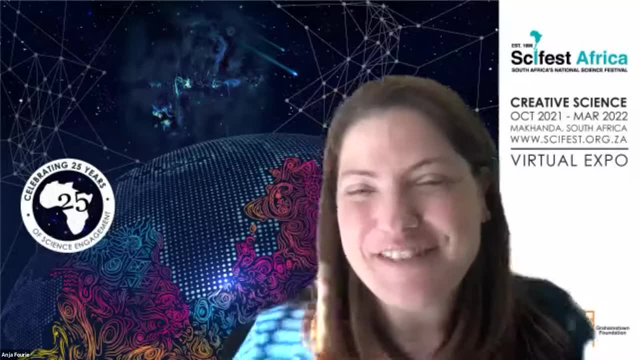 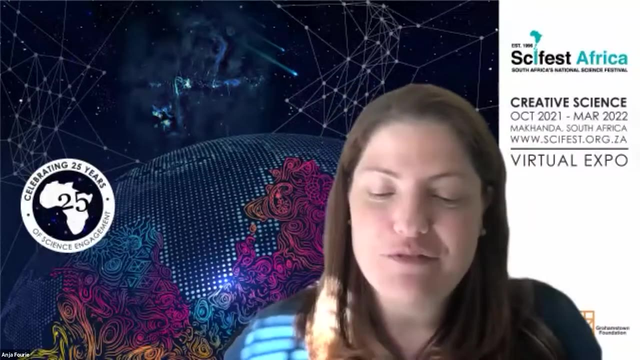 OK, So a comment from our friend Daniel Matsupola. Great presentation, Kevin. Your energy vibrates up there in the higher echelons of energy vibrations, And it's good to hear from you, Dan. All right, So you know, at the NRAO we've moved to, you know. 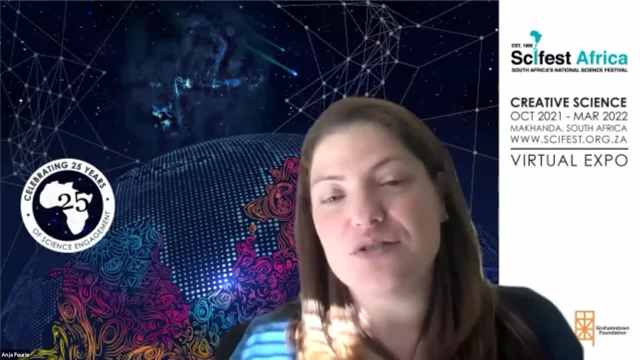 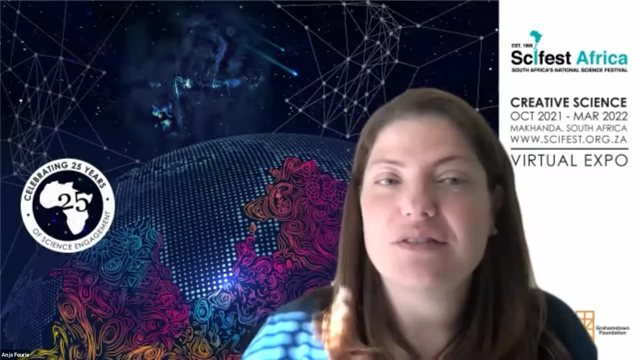 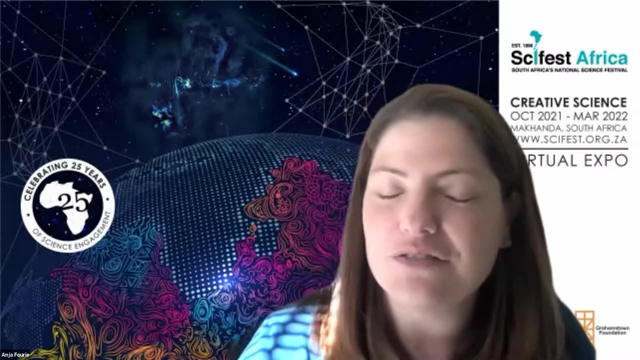 where we try to train or teach every single student who comes through the NRAO in project management. they very quickly learn- is that you know you can design the world's best project, but if there's no need for that project, you know really you designing, as we always say, a white elephant. 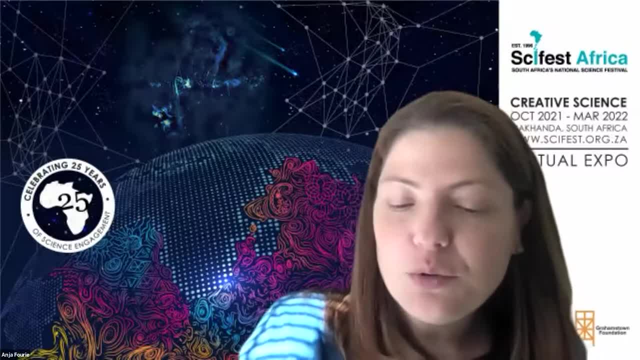 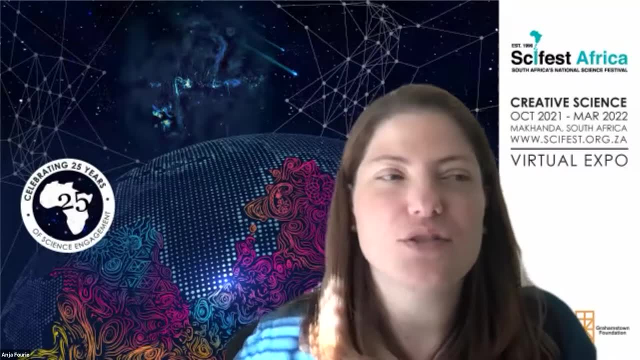 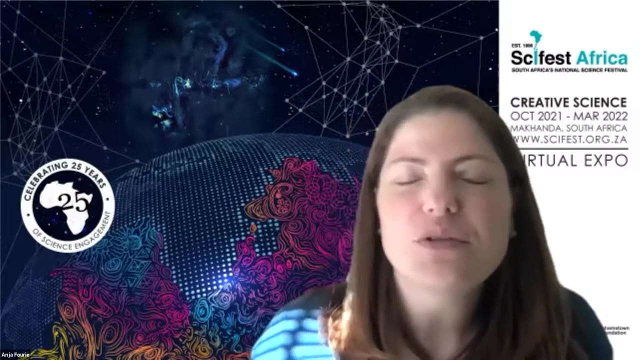 um, for, for you know, audience members who would like to design a project but, you know, aren't necessarily connected to what is needed. um, you know, are there resources, international resources or regional resources? how would you suggest they go about? you know, finding out what that need may be? 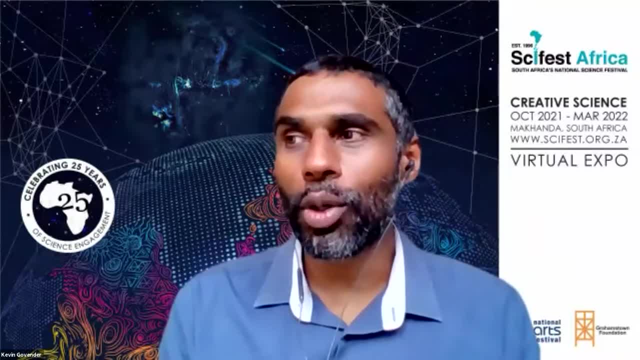 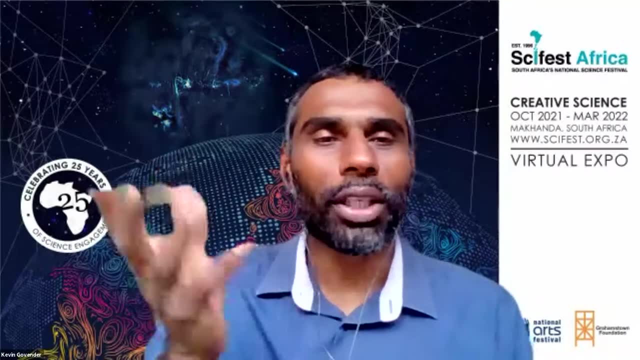 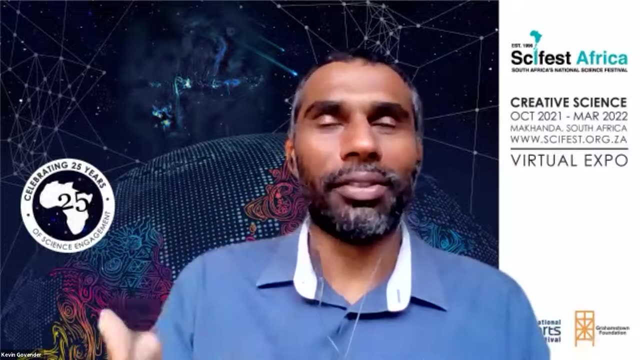 that's a. that's a great question. um, so one of the one of the aspects of our sort of online course to help people, sort of design project, is it's something called a needs analysis. it's you know, it doesn't have to be complicated, but if you're going to serve someone you need to know what they. 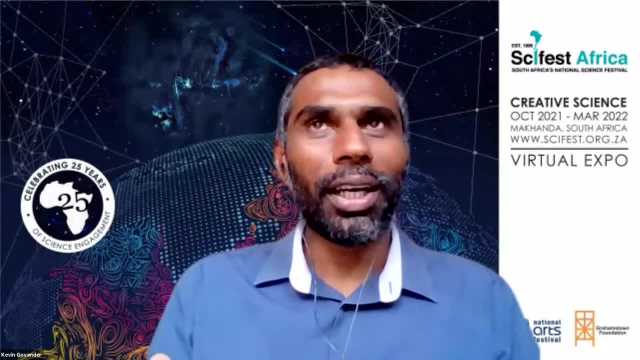 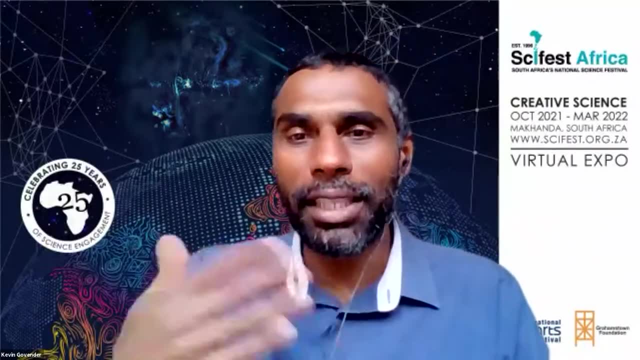 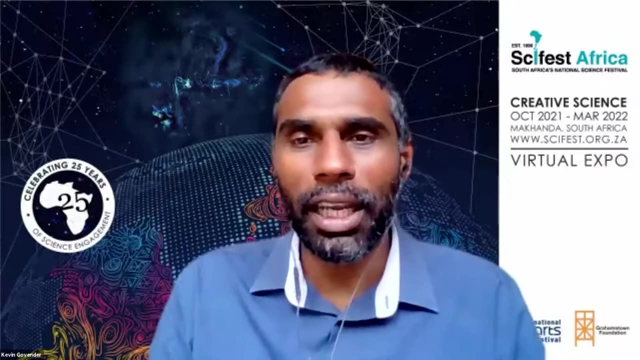 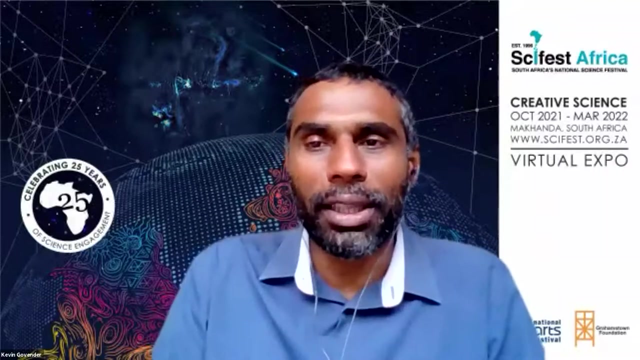 need and um and so um. you know a basic needs analysis, you know, can be as simple as a questionnaire or or engaging the audience that you, that you hope to target. so if you, if you want to run a, a workshop, a teacher training or something like that, before you design the project you need to engage them, you know talk. 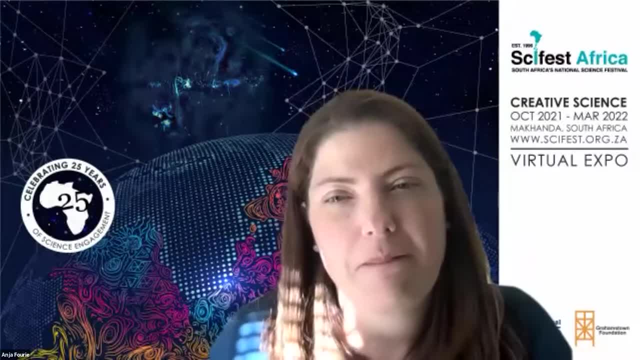 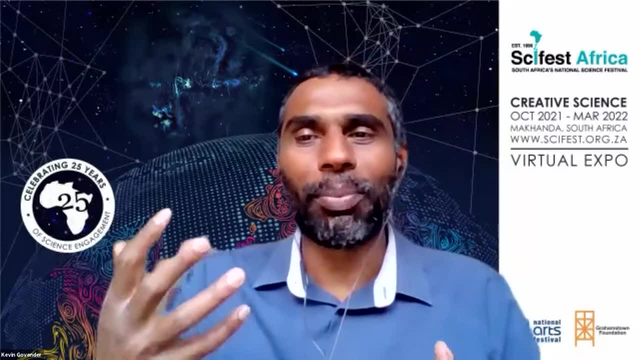 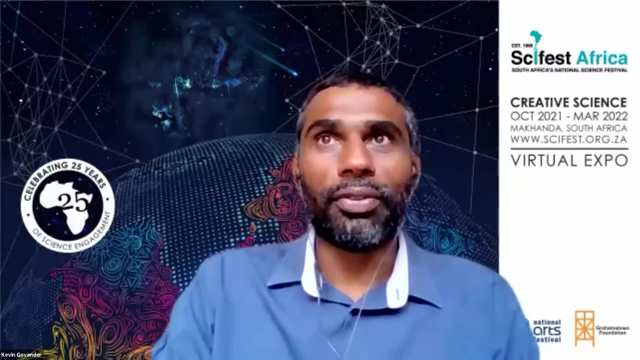 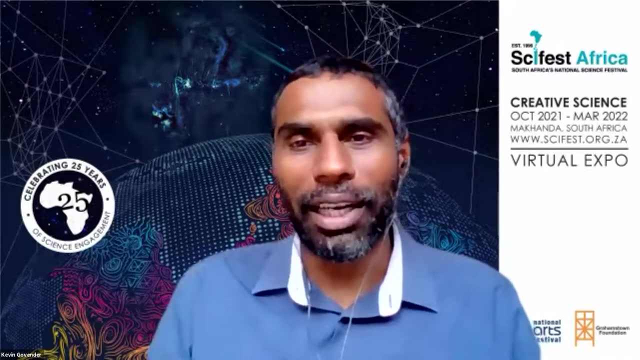 about what the needs are and uh, um, you know something that that anya actually taught me: this term co-design, you know, you, you, you sort of design the project with your target audience so that the needs are taken into account in terms of, of, of general resources. you'll find, uh, so, if you want to know sort of the state of. 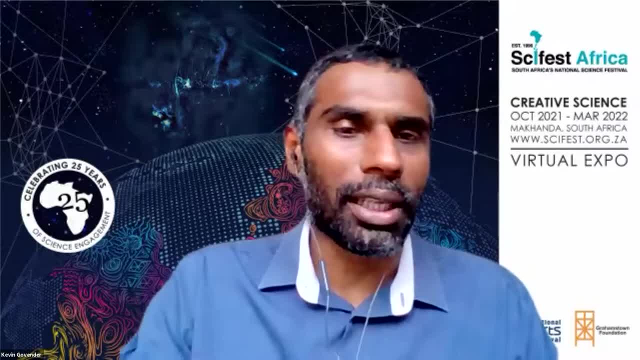 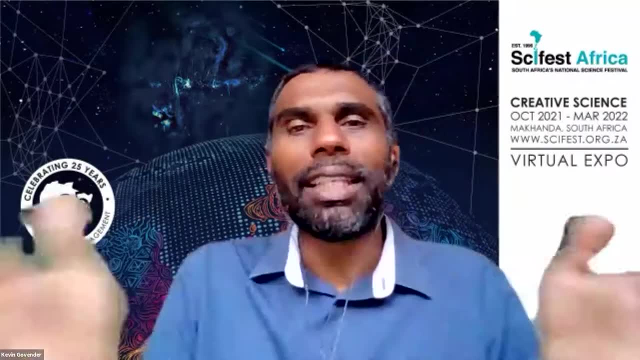 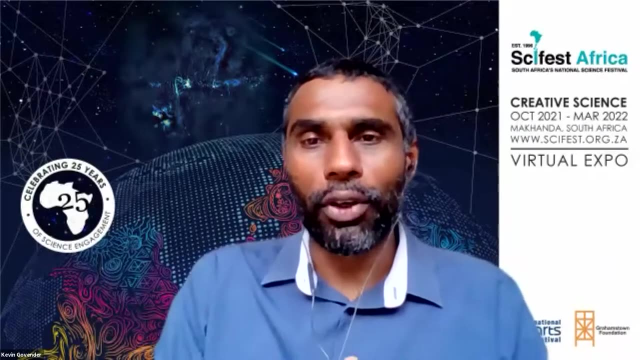 development. uh, uh, you know you you'll find resources in places like the world bank and international monetary fund uh in the united nations, where there'll be sort of analyses of uh the state of the sdgs in different parts of the world so you could look up the general data for for your 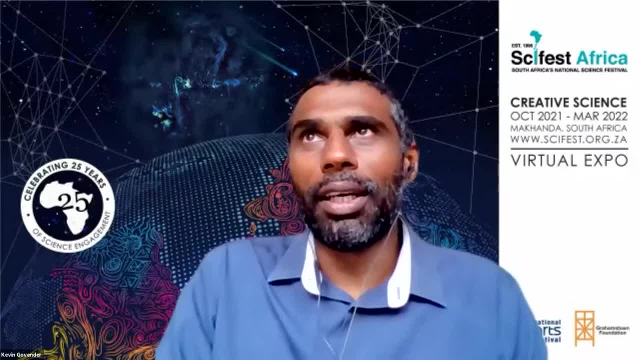 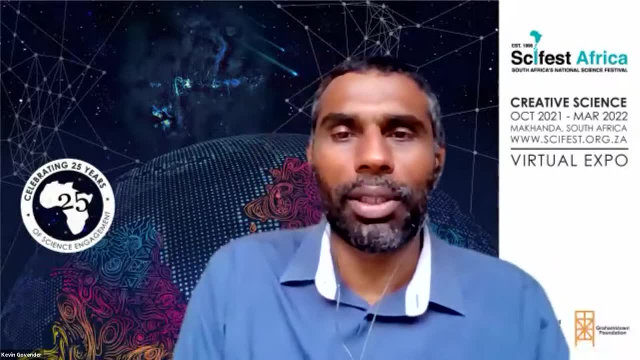 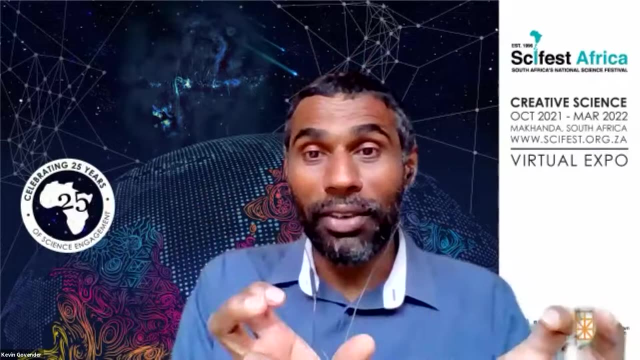 country and you know it might say: you know, uh, the level of of maths education is is low, and then you might want to target that or something. but there's some really nice resources if you look up the un sdg indicators, because the sdgs are only the 17, but behind the 17 there's hundreds of indicators which 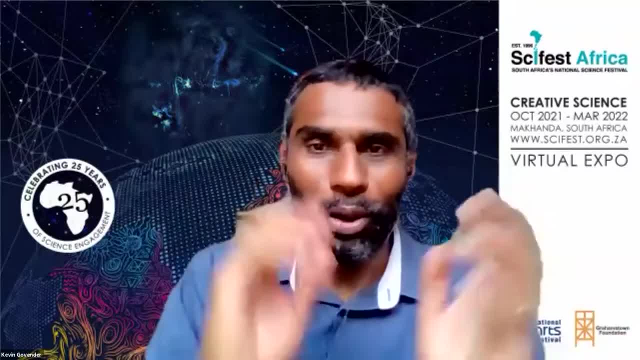 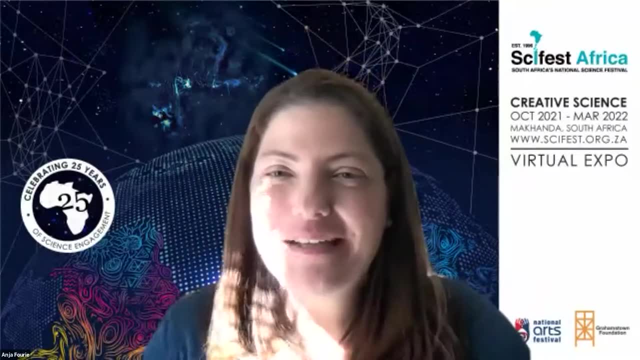 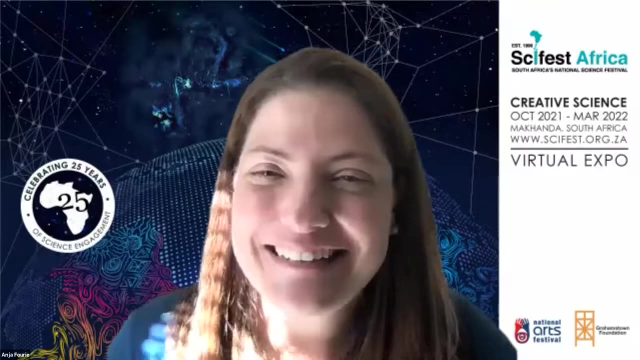 is a breakdown of those 17 sdgs, and then you'll you'll have a very good guideline. okay, now we have a question from kenneth mongero um, who's the president of fun and educational global network director at the science center kenya. good to hear from you as well, ken um, and kenneth wants to know, you know, do human? 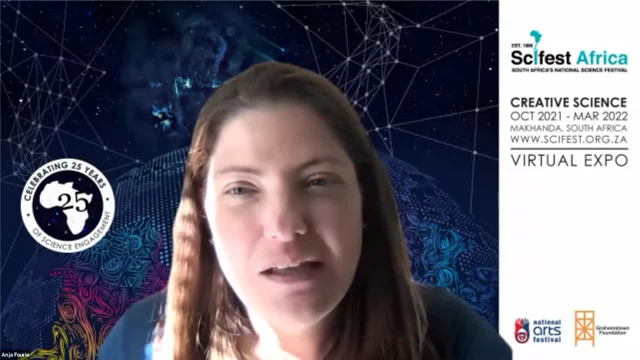 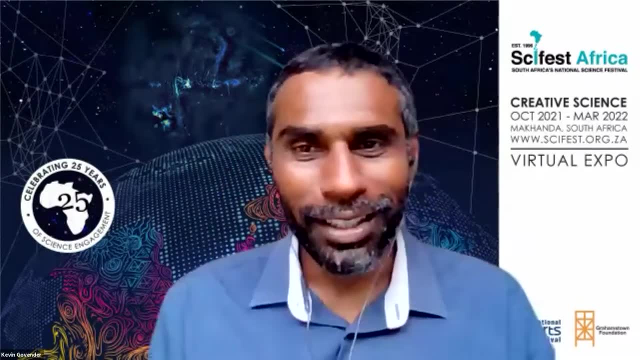 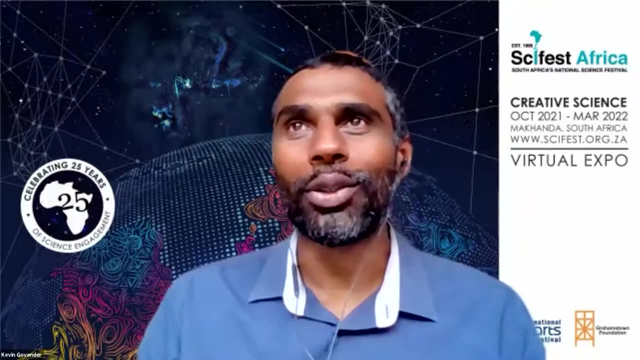 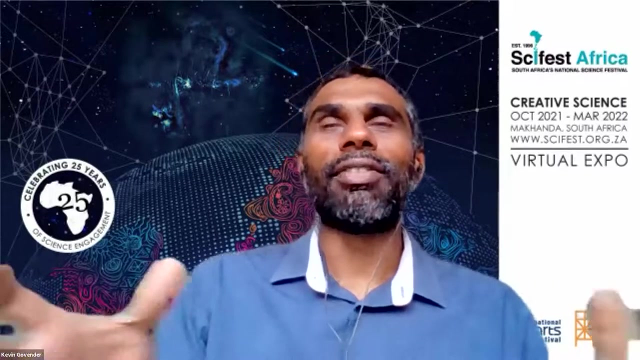 activities influence space, just like climate change, and, if so, what are the biggest problems and what can be our contributions to solving that? that's a that's a great question. you know, wherever human beings explore, uh, they tend to leave a mark. astronomy, as a as a field is, is, uh, is relatively passive in that we can't reach the. 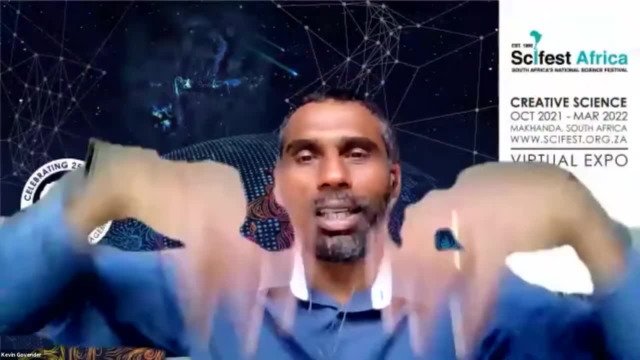 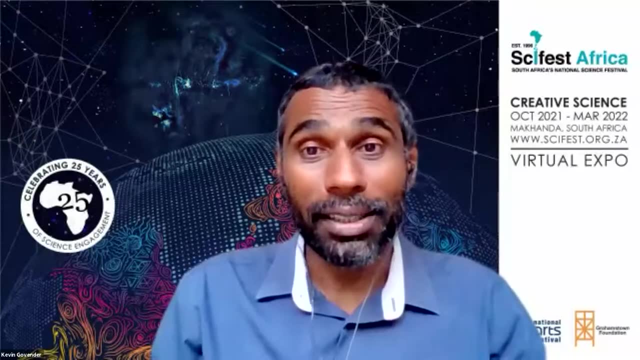 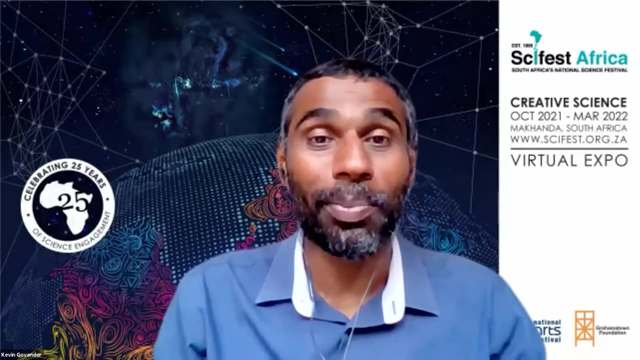 stars, to pollute them or something else, so we just catch the light that comes from the stars. but space- like exploring space physically, you know, putting satellites around planet earth and things like that- that has left quite a significant mark and the biggest challenge we have right now is space debris. it's that we've put so many satellites. uh, you know. 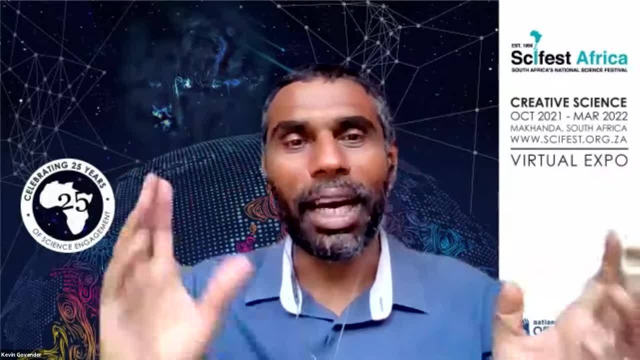 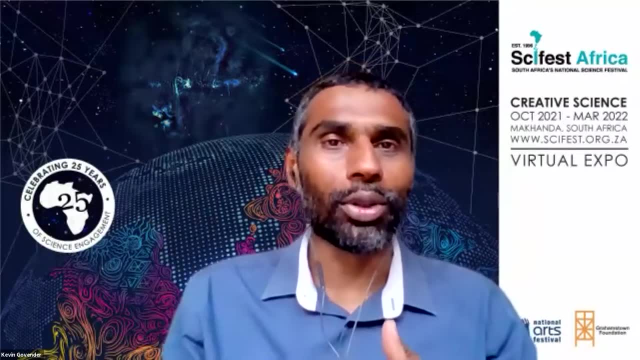 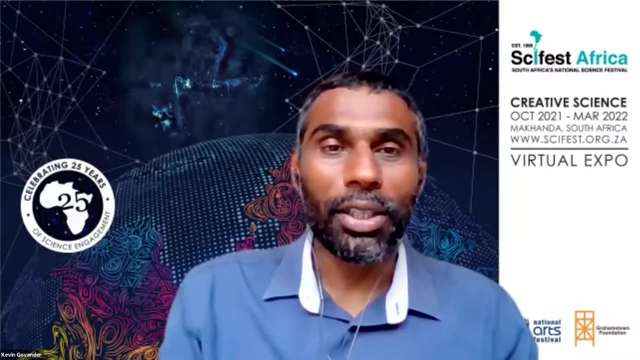 around this planet that you know when, when a satellite dies, or you know when it uh reaches the end of its life, if, if, if it hasn't been designed properly to sort of return to earth or burn up in the atmosphere, it just keeps on going around and this space debris is a huge 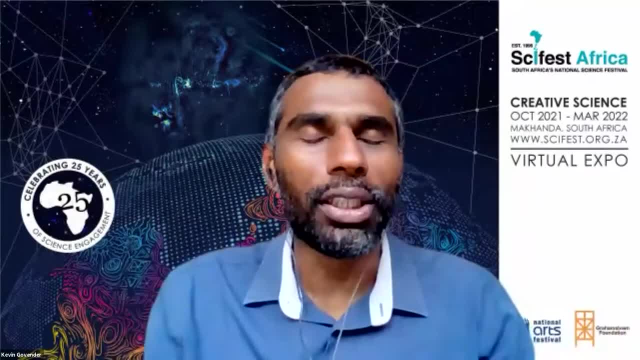 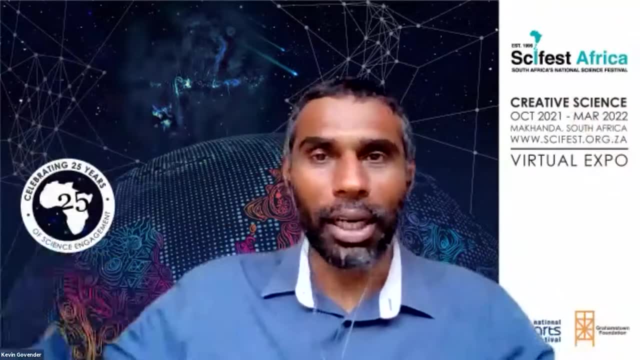 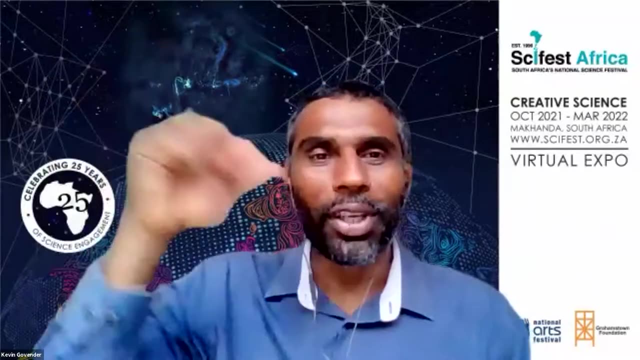 challenge and this huge there's like big communities looking at what to do about it. big space debris: you can track. you know, if something is as big as a car that's floating around, you can track those. but like, imagine, imagine a little screw. if there's a little screw, that's that's that's moving around the earth. 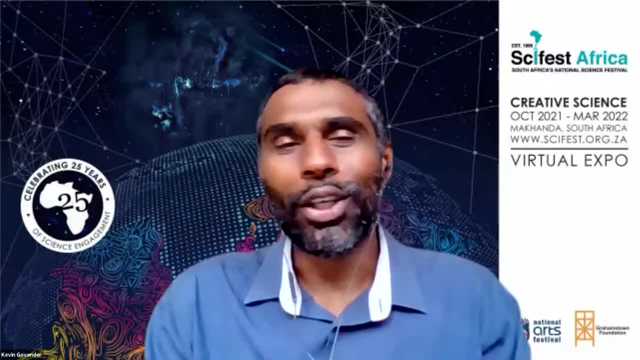 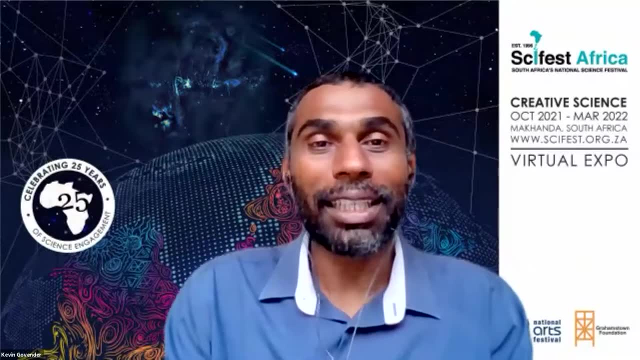 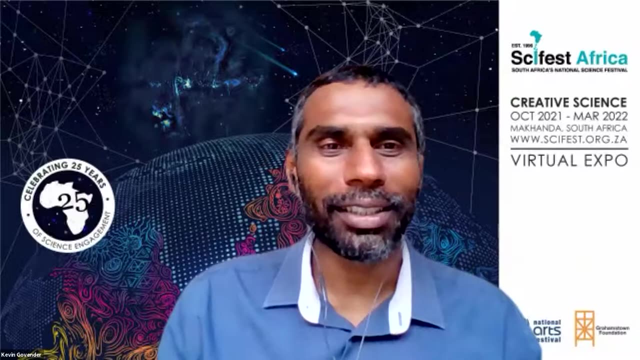 and then your astronauts go out there or you have, you know, your your dstv satellite and this little screw comes in. it's going to hit it like with the force of a bullet, so that that can be really, really disastrous. and i think there's a, there's a hollywood movie, i think it's gravity or something like that. 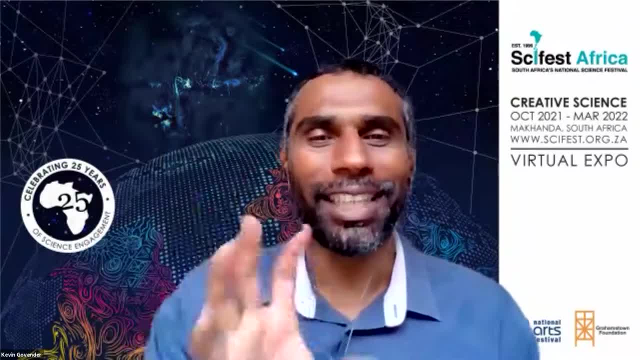 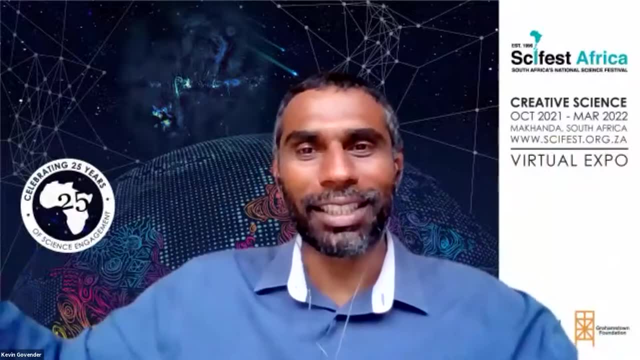 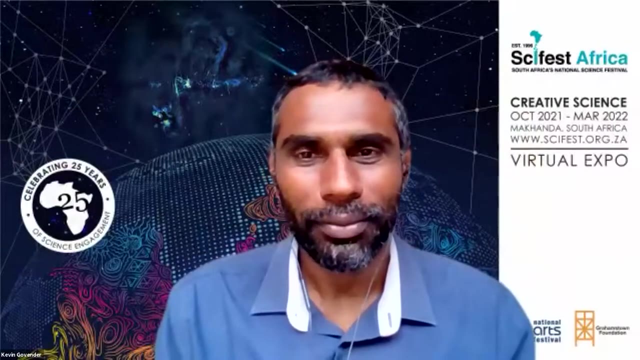 sandra bullock, i think. but you know, that illustrates us really well where, you know, one, one satellite hits another and then creates this, this chain reaction, and just the whole, the whole of our near earth space gets messed up. thank you, kevin. and then a very interesting question from numfundo fuzani. 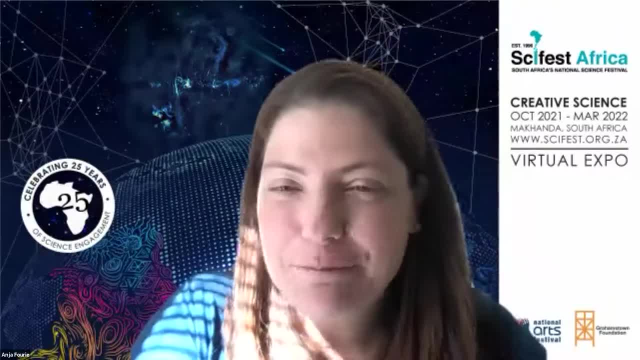 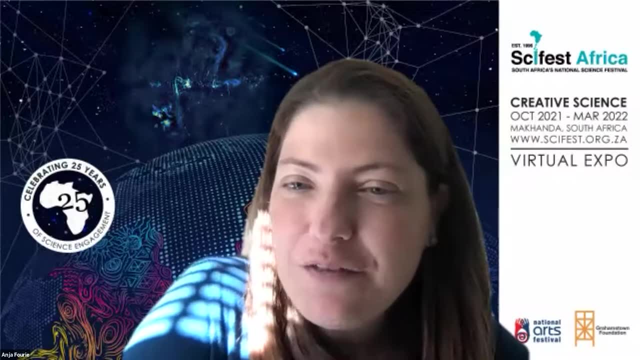 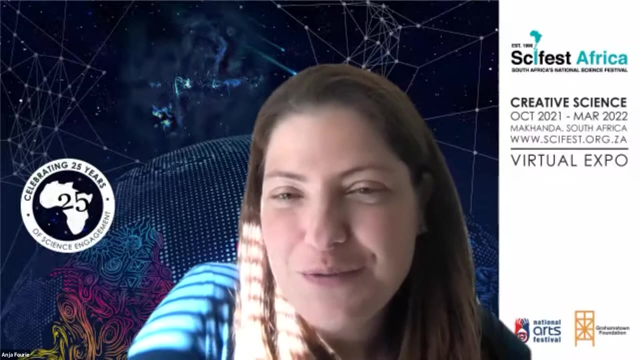 and i love this question. thank you for some presentation, kevin. to apply for funding, does one have to have an astronomy background or a certain standard of education, and if it's a post metric that has a vision in the field of astronomy, can he or she be funded? do you evaluate a vision before providing funds? 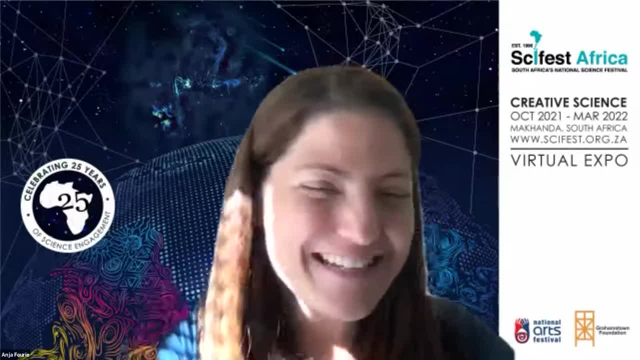 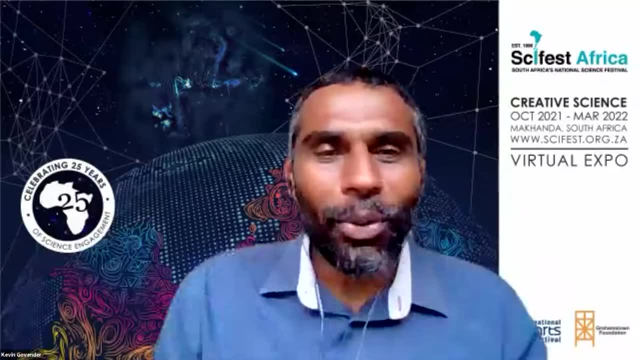 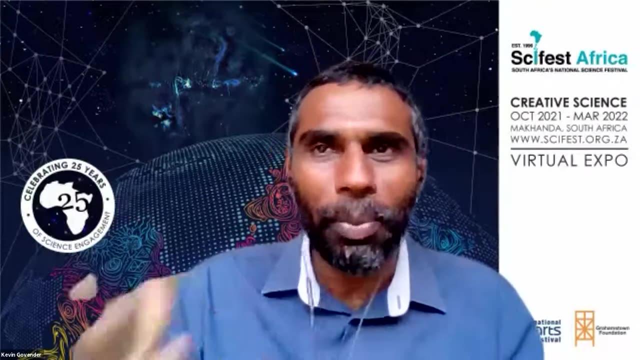 and i- and i just know what the answer is from iu oad and i get so excited- absolutely no restrictions. we want anyone anywhere in the world to be able to apply. so anyone that that has an idea to use astronomy in some way to impact on your community, on your 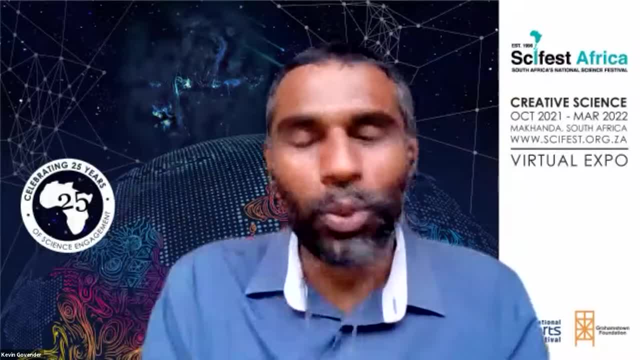 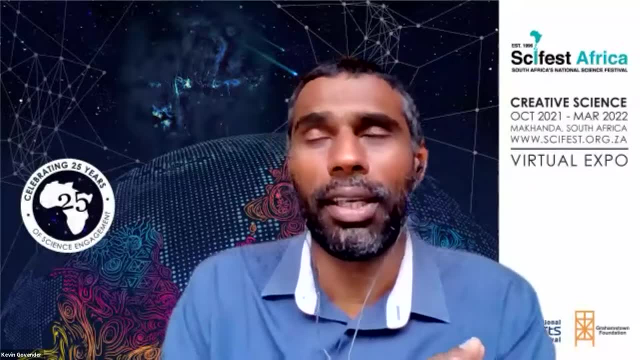 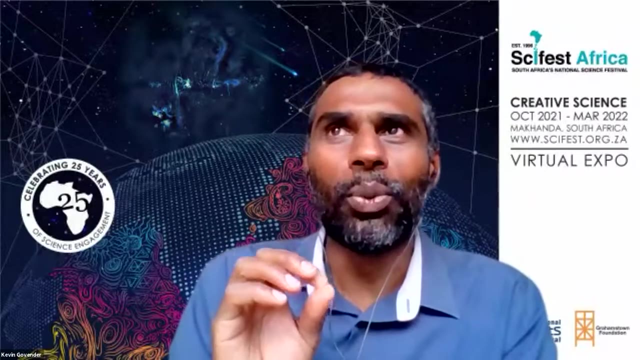 society impact on development. we, we would, we would be more than happy to receive your proposal. there's no, there's, no, there. there's no tertiary tertiary qualification required or anything. it's just, you know, what we want to see is that it's a good idea and it's an idea that can be implemented. 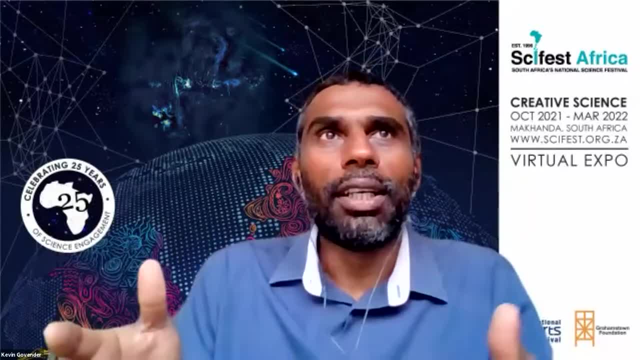 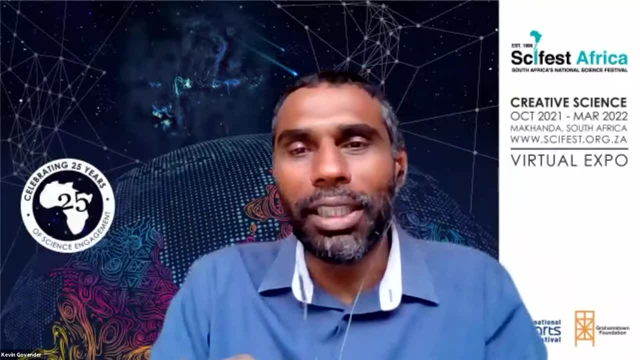 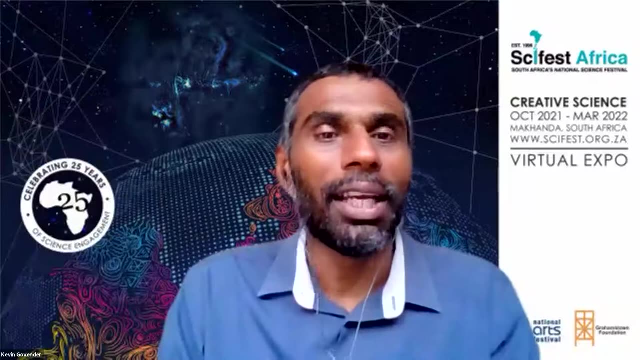 so so if you don't, you know, if you need to have, uh, someone with astronomy skills, you don't have to have the skills, you can just get someone on your team. you know who who has the skills. so so we try to build teams of people from different fields and you know the whole is should be greater than. 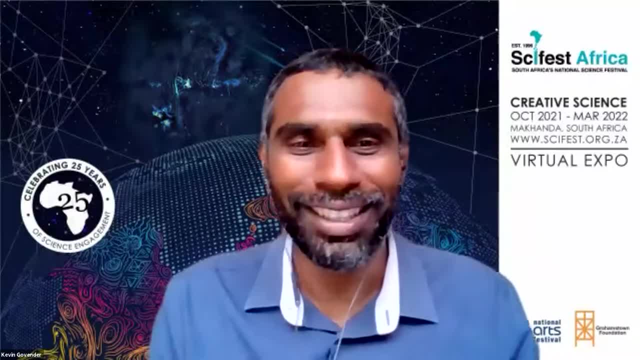 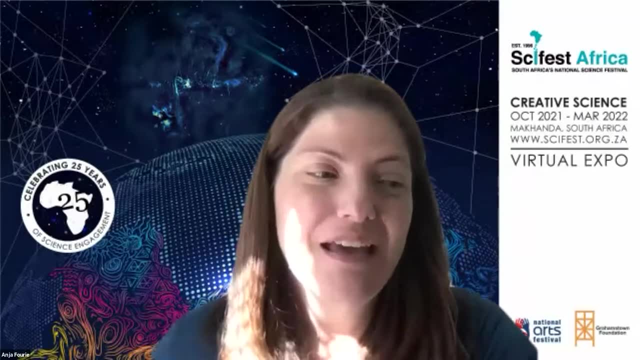 the sum of the parts, as, uh, george miley used to say: yeah, and i absolutely love that approach and i'm full of, because often what happens, you know, is that you're not going to be able to this topic or you want to keep your team really as cool, as incredible as it all is that you have. 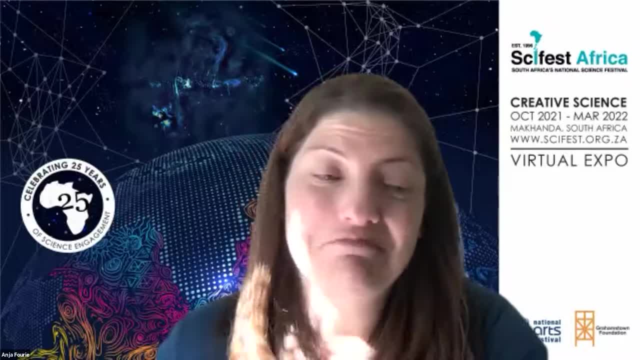 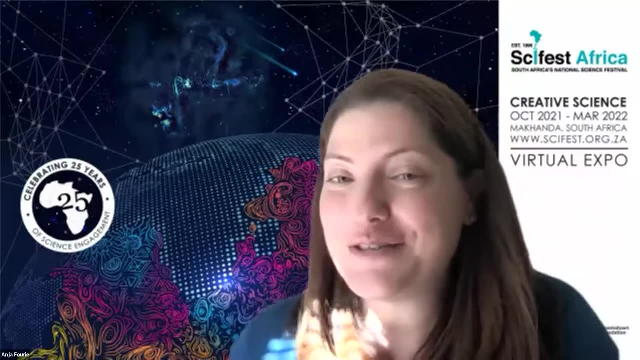 these very diverse groups that come together and you know three years later they establish very effective, you know, non-government organizations that do great work. so you know it starts with that vision and starts with an idea and three years later it you know it's really having an. 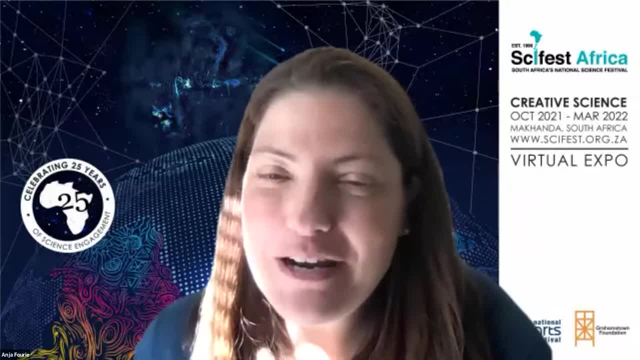 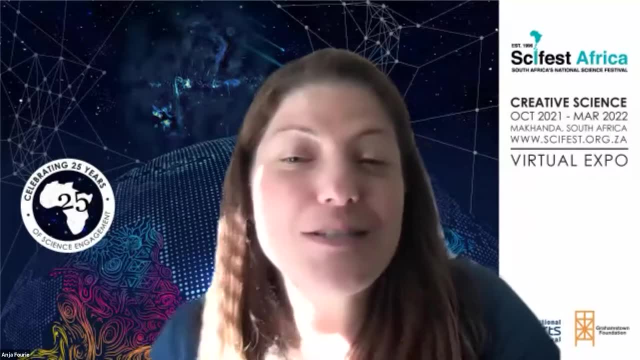 impact right um. next question, possibly the last, but we'll see if we can fit one more in um great Kevin, thank you for being part of SciFest. I am interested in your views on the current space tourism initiatives. We have seen very high profile business people and celebrities take. 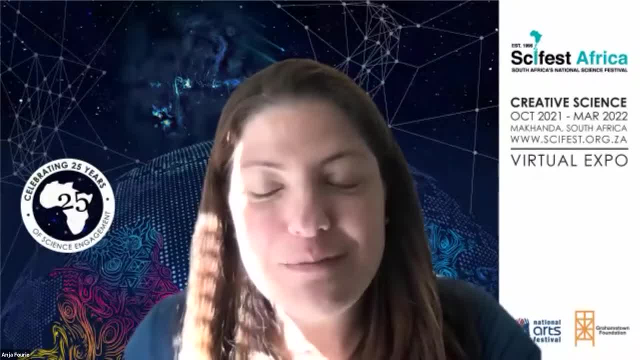 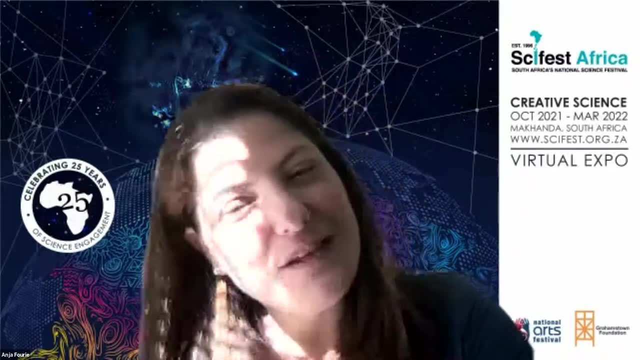 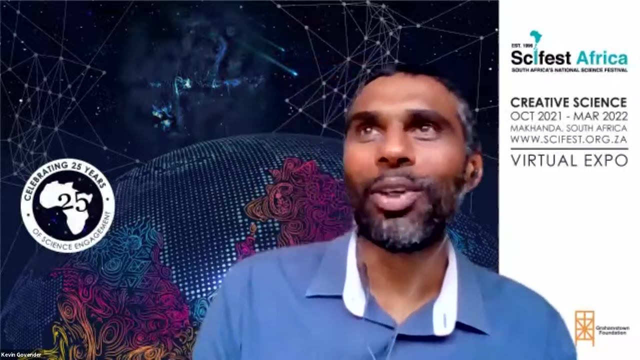 the opportunity to go to the final frontier. Tourism is generally regarded as an industry with significant potential for sustainable development. Is that true of space tourism? do you think That's a very, very interesting question, And I have my own opinions about it. 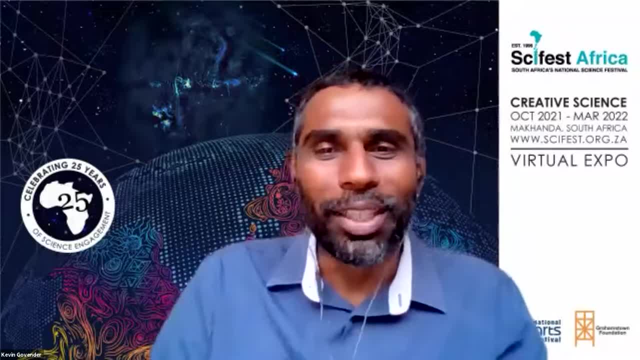 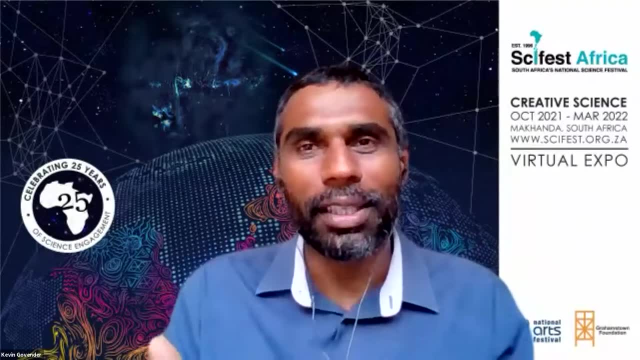 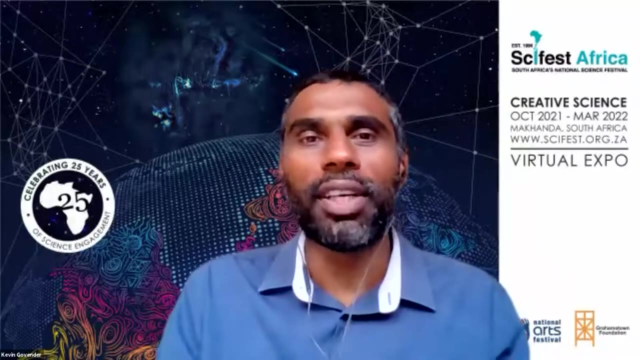 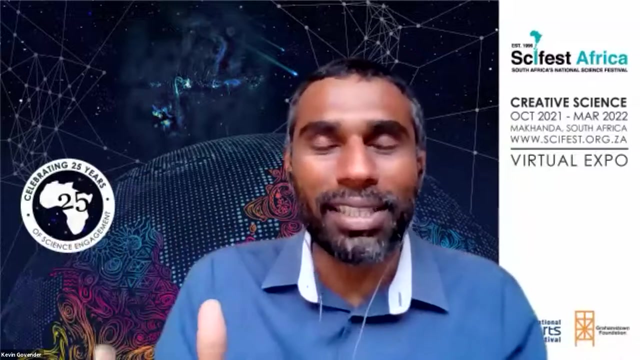 I don't know whether to be diplomatic or to be just brutally honest, But the exploration of space has stimulated a huge amount of technology around the world. But not just that. When we first sent spacecraft to the moon, when we first got into space, it inspired a whole generation of 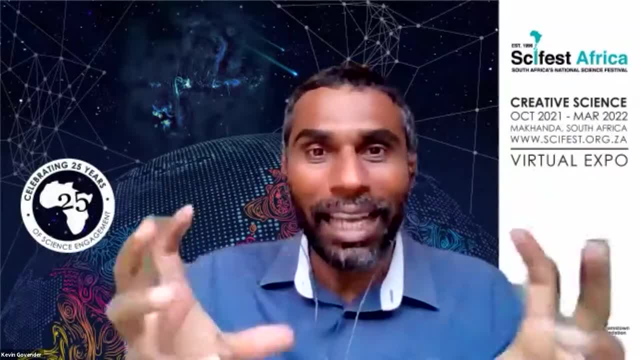 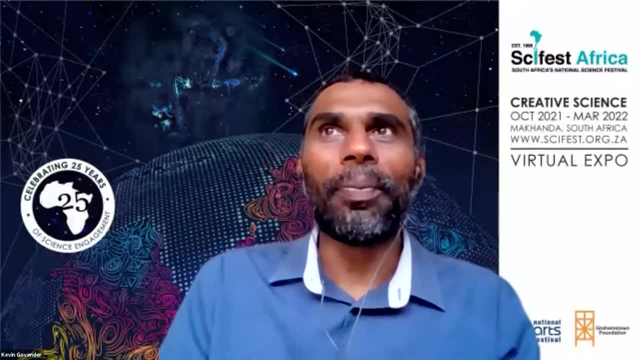 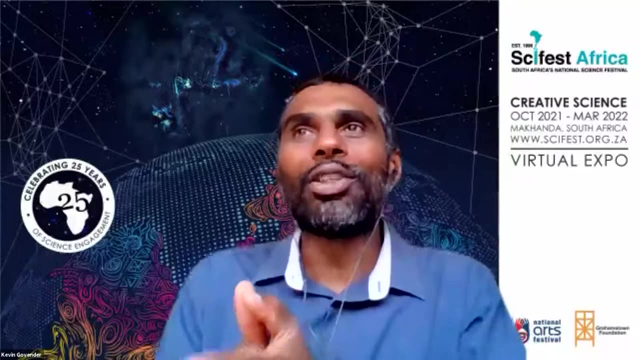 engineers, of scientists, And that is a great thing. And nowadays, with the space tourism industry, it is kind of questionable in that, you know, are we doing something new, Or is you know someone just putting a lot of money into, you know, doing what's already done, which is getting a rocket? 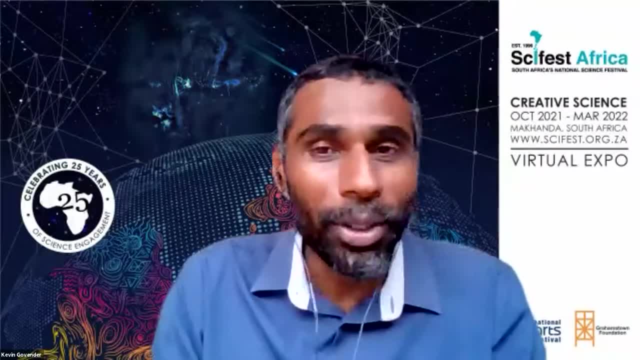 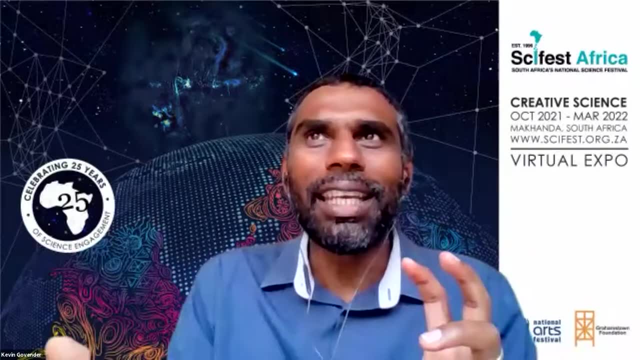 up there getting people up into space at a huge carbon cost, And it's like wealthy people who pay to get up into space. So, you know, is that really? Is that really a benefit to society? I'm not too sure, But it is something that keeps the enthusiasm around space going, So there could be a very positive impact on you know if it's done well. So I think if it's not just you know, a rich person's club that you know wants to go and have a joyride and come back- but it's something more if it's connected with inspiring people. 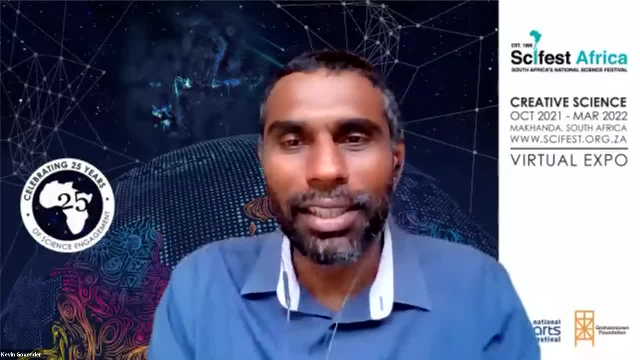 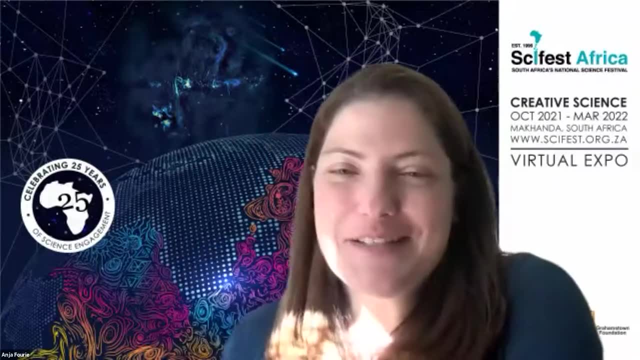 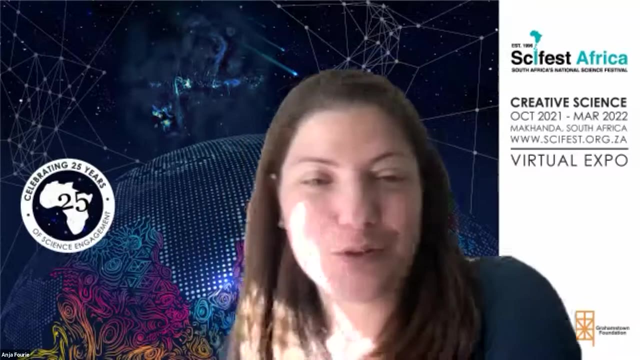 connecting, you know, connected with doing interesting research in space. I think it could have huge potential. Thank you, Kevin. All right, So one last question and then we need to wrap up. What advice do you have for young people you know, like Nomfundo, who you know really are? 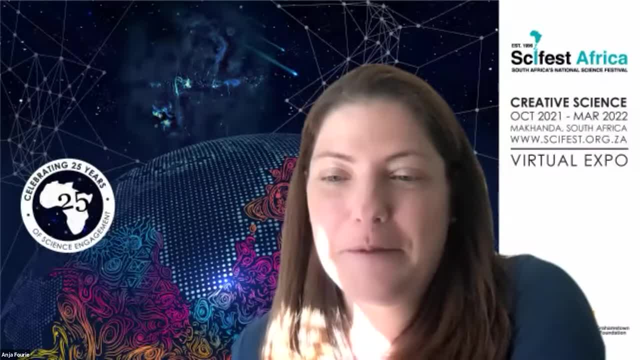 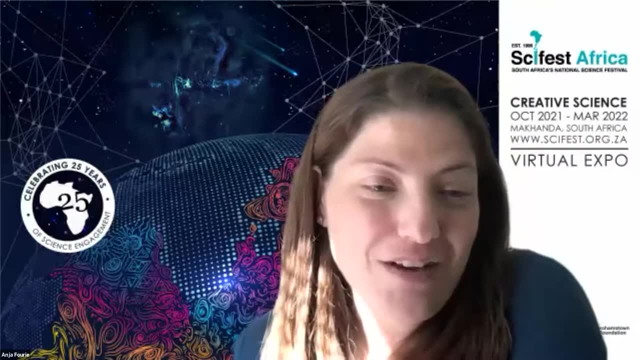 passionate about using what they do for development, or who are starting out in their research careers. Where do they start, You know, if they have an idea for using astronomy or their particular science for development, what would be a good Starting point? 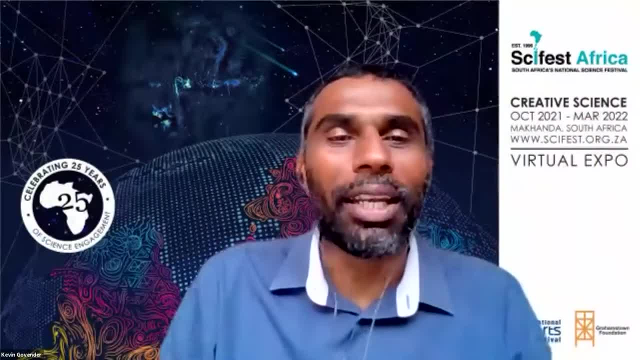 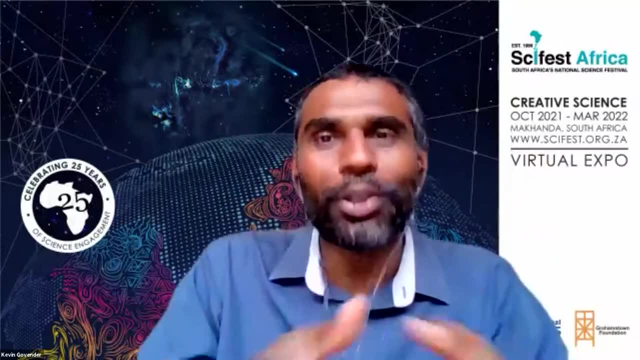 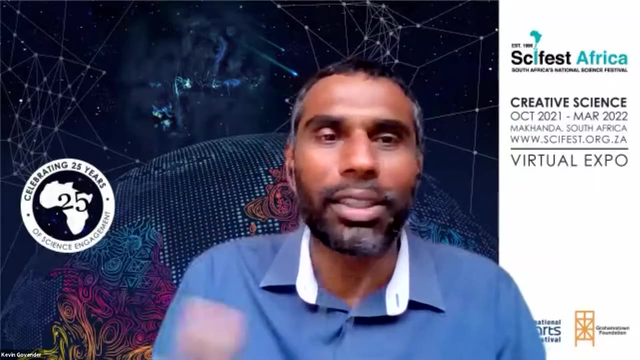 Simple answer: Get in touch with me, get in touch with us. I mean, this is exactly the reason that we created the OAD: as a space for people like Nomfundo, like you know. anyone who has ideas, who wants to put their ideas into interaction, get in touch with us, because this is a space where 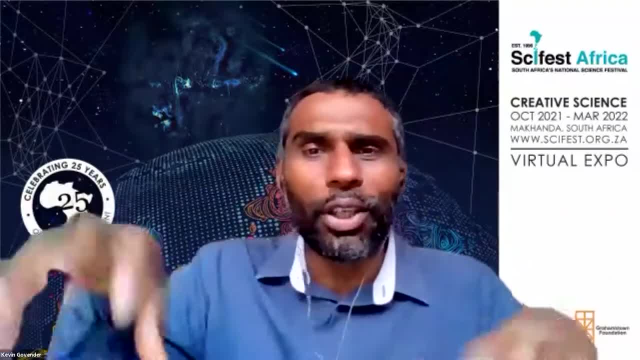 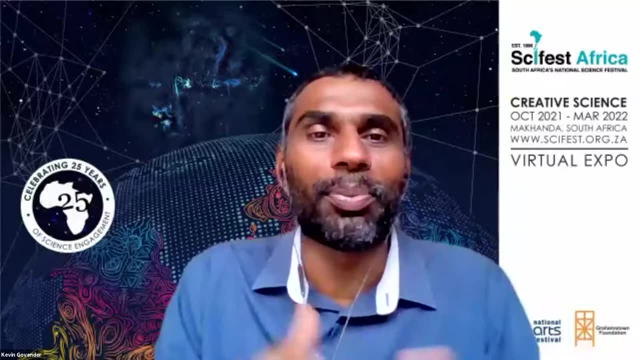 we've got a development economist, we've got an astronomer, we've got, you know, people with different skills and you know, come in, Let's brainstorm, let's figure out your ideas, and then we'll give you guidance specific to your. 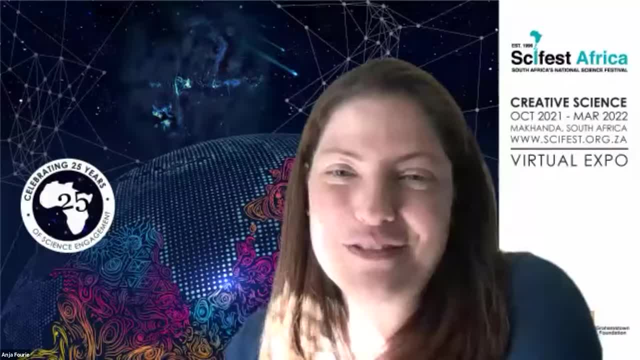 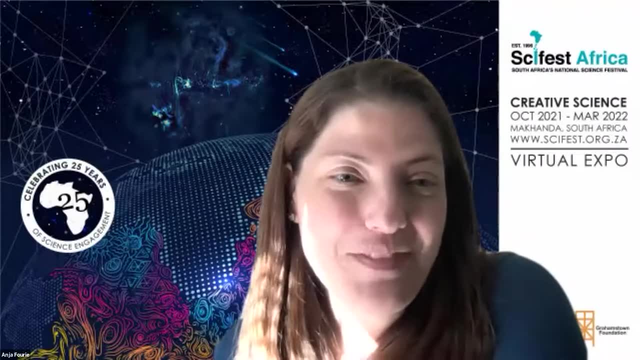 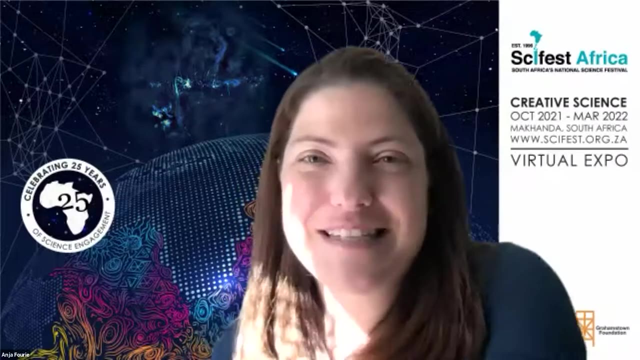 idea and your environment. Thank you very much. And of course, the great thing is is, you know, besides headquarters, there's also all these wonderful regional offices that people around the world can get in touch with, And what I would like to do is just remind or give people that website, which I always love. 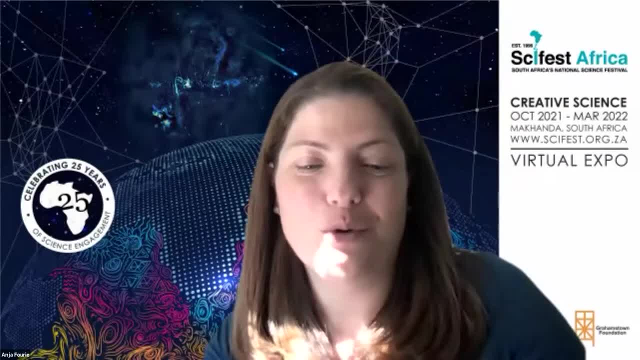 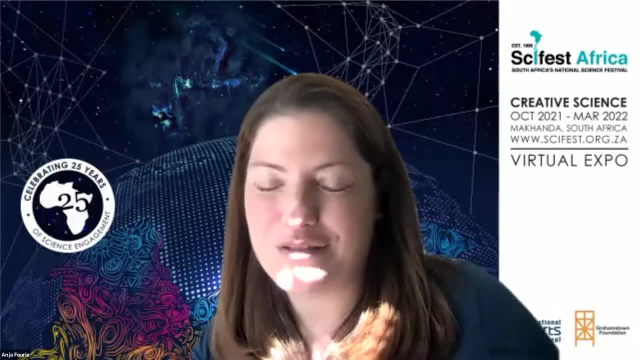 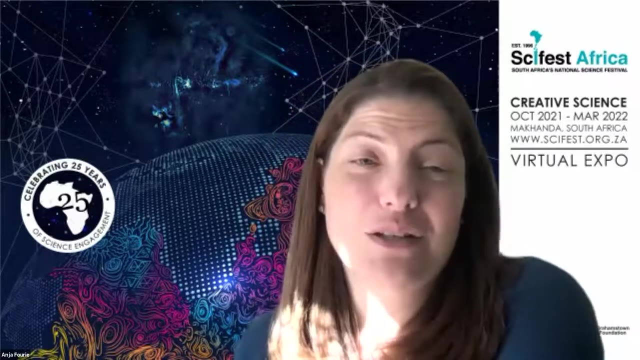 and that is astro4, as in the number 4, devorg, And we will put that in the chat to everybody but SyFest, if we could just make sure that goes onto the Facebook comments as well. So go to astro4devorg, have a look at the website, look at the incredible projects that the IAU OAD are doing. 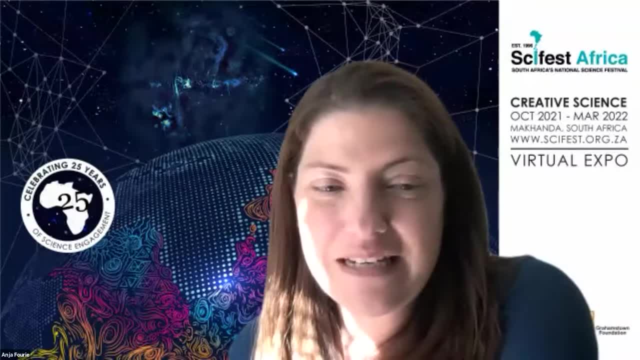 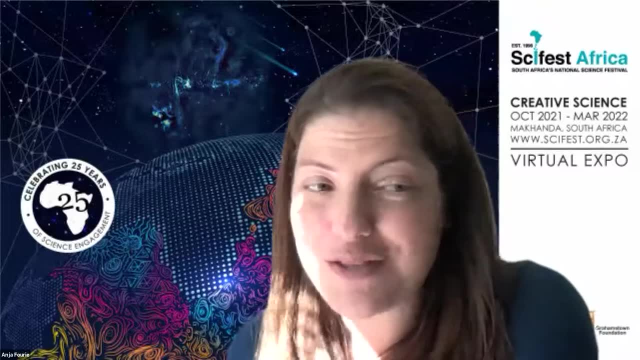 If you are in an institution in South Africa or around the world, get in touch. Often it's you know the Office for, you know Diversity and Inclusion, or an Office for Development, or go see the big boss, you know, just take that plunge. 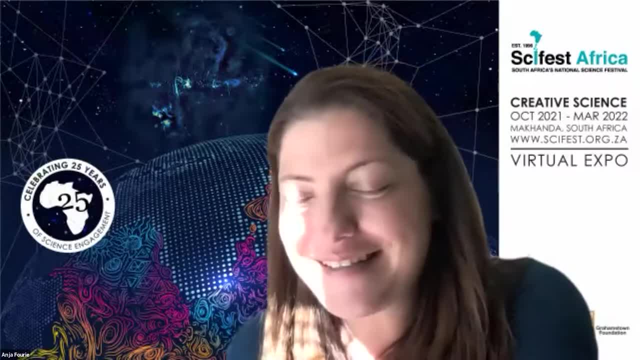 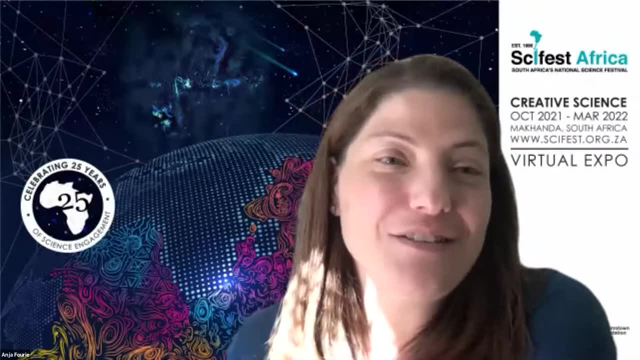 So thank you very, very much, Kevin. As I say, it's just always a delight Watching the passion that you have for this and always have had. It makes me passionate about what I do, And you know, if you have loved what Kevin has to say, you know where to get in touch with him. 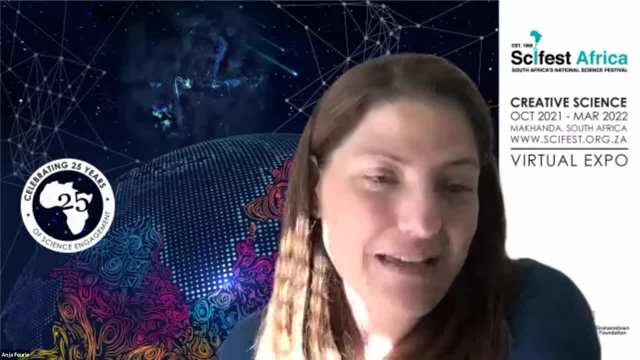 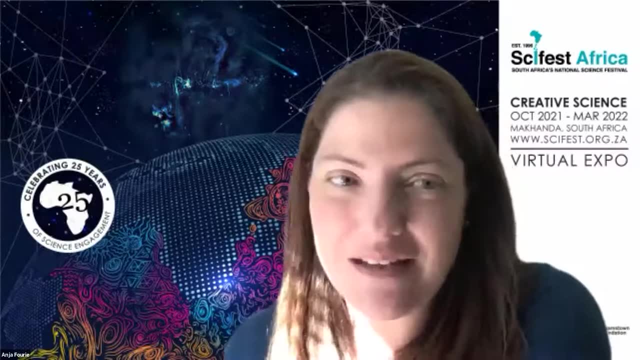 But also have a look out please, for you know, other webinars, like Kevin's on the SyFest Africa 2021 program, And you can have a look at that. That is syfestorgza. or visit the SyFest Facebook page or the Twitter page.